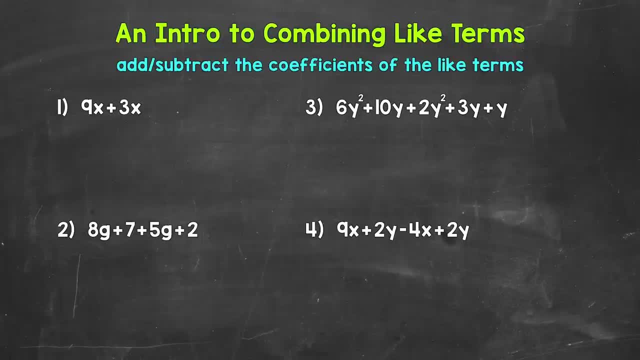 Now remember: like terms are terms with the same variables to the same powers. When we combine like terms, we look for any like terms in the given algebraic expression and combine them into one term. By combining like terms we can simplify. That just means we can rewrite the original expression in a simpler and easier way to understand and work with. 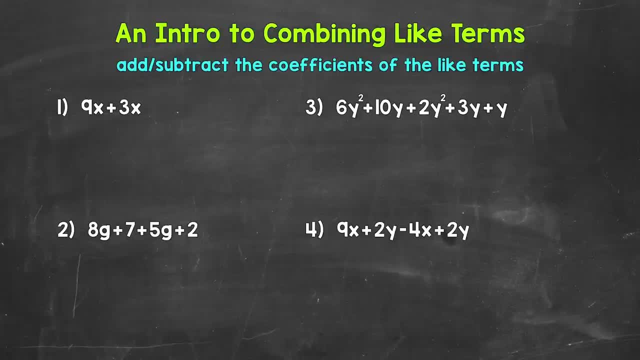 Let's jump into number one, where we have 9x plus 3x. We will start with this basic expression and work our way up. So we have two terms in this expression: 9x and 3x. Both terms have the same variable of x and these variables of x are to the same power. 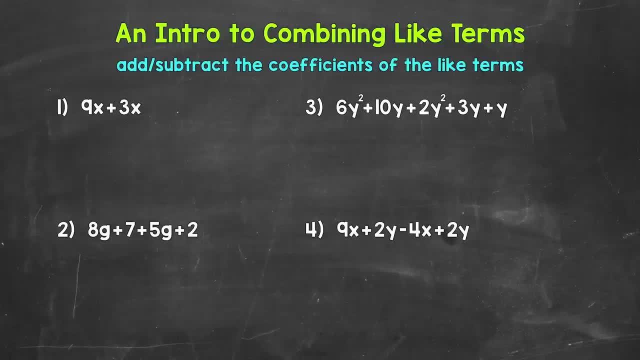 Remember, when we don't have an exponent attached to a variable, there is an understood exponent of 1.. Anything to the power of 1 is just itself. So 9x and 3x are like terms. Now, when we combine like terms, all we need to do is add or subtract the coefficients, the numbers in front of the variables. 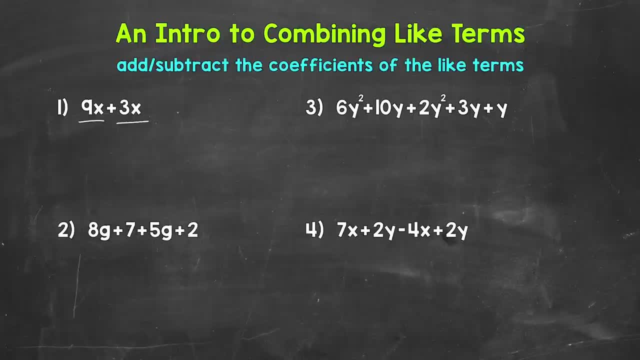 The coefficients in number one are 9 and 3.. We have a positive exponent, We have a positive 9x plus a positive 3x. So let's add those coefficients. 9 plus 3 is 12, and then we have the variable of x. 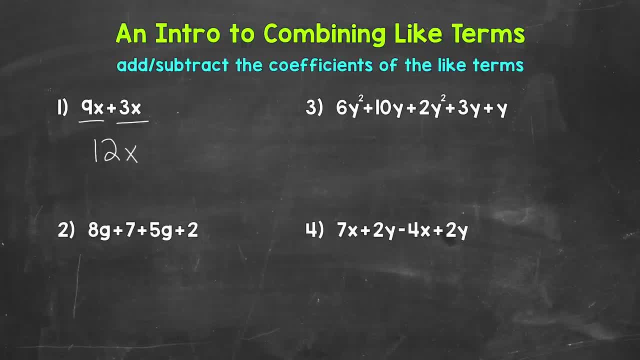 And that's it. We took those two like terms, 9x and 3x, and combined them into one term, 12x. 12x is equivalent to 9x plus 3x, So we didn't change the value of the expression. 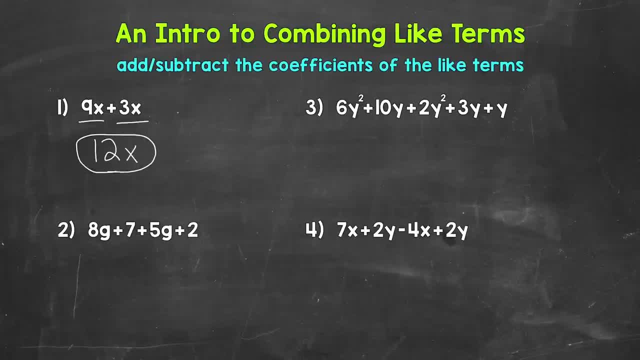 So 12x is our final simplified expression. Let's move on to number two, where we have 8g plus 7 plus 5g plus 2.. Are there any like terms that we can combine in order to simplify this expression? Yes, we have 8g and 5g. 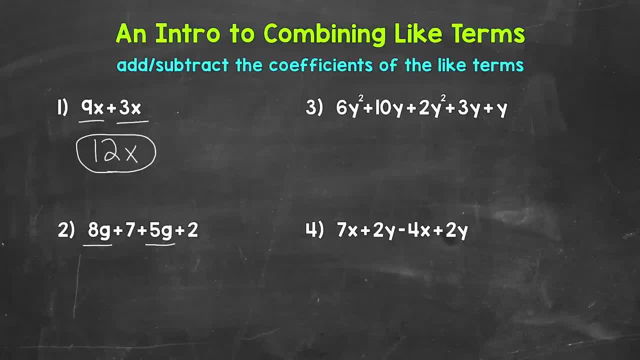 Both of those terms have that variable of g. And then we have constant terms 7 and 2. I'll box in the constant terms to separate them. I'll separate them from the 8g and the 5g. Now we can combine like terms. 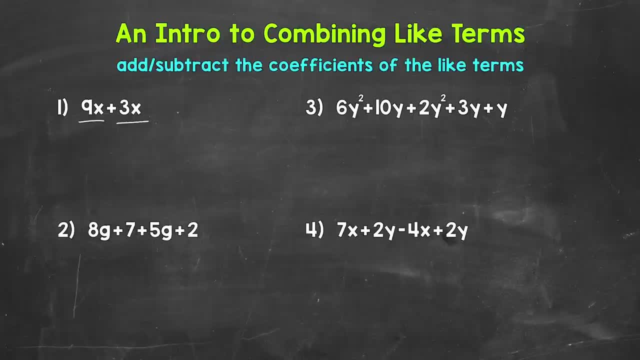 The coefficients in number one are 9 and 3.. We have a positive exponent, We have a positive 9x plus a positive 3x. So let's add those coefficients. 9 plus 3 is 12, and then we have the variable of x. 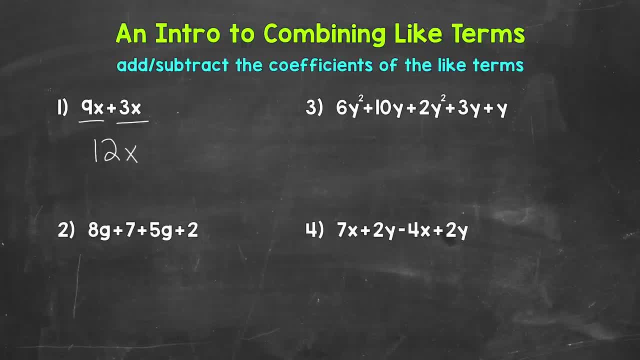 And that's it. We took those two like terms, 9x and 3x, and combined them into one term, 12x. 12x is equivalent to 9x plus 3x, So we didn't change the value of the expression. 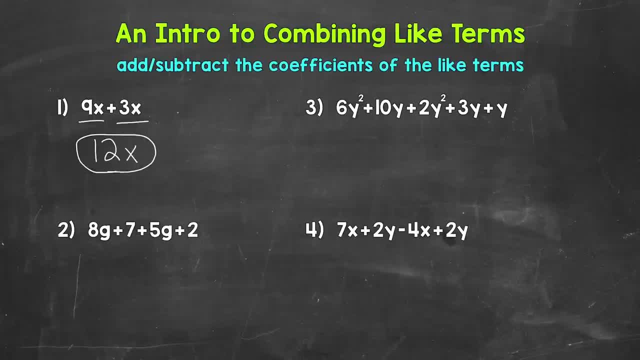 So 12x is our final simplified expression. Let's move on to number two, where we have 8g plus 7 plus 5g plus 2.. Are there any like terms that we can combine in order to simplify this expression? Yes, we have 8g and 5g. 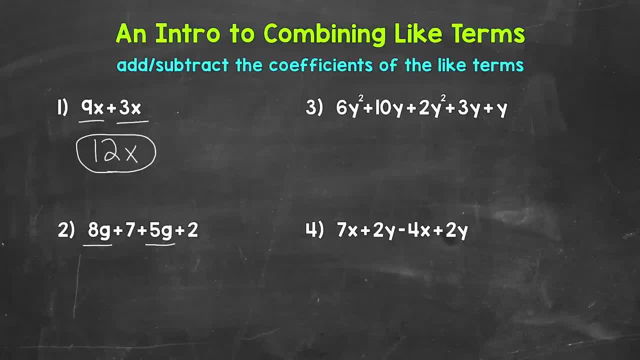 Both of those terms have that variable of g. And then we have constant terms 7 and 2. I'll box in the constant terms to separate them. I'll separate them from the 8g and the 5g. Now we can combine like terms. 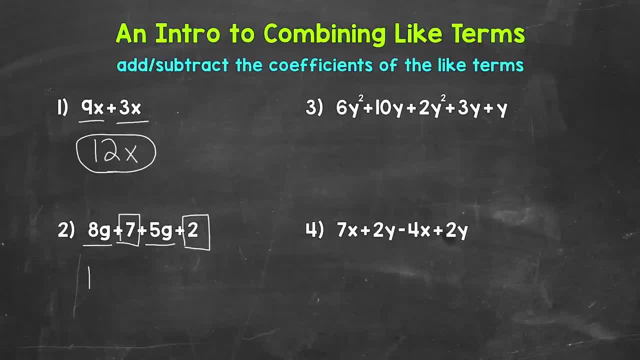 We have 8g plus 5g. That gives us 13g. And then we have 7 plus 2.. That gives us 9.. So we end up with 13g plus 9.. And that's our simplified expression. 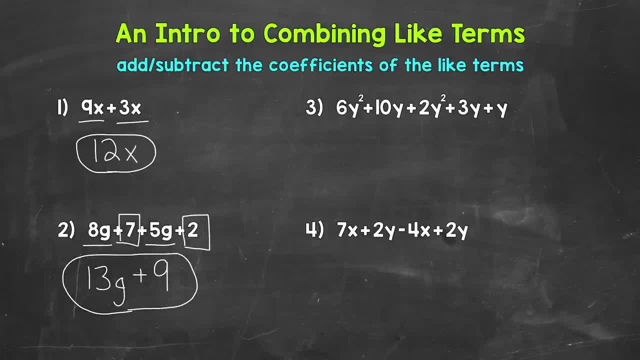 That expression of 13g plus 9 is equivalent to the original expression. We were just able to simplify the original expression by combining like terms. We started with four total terms, but we were able to combine like terms And now we only have two total terms. 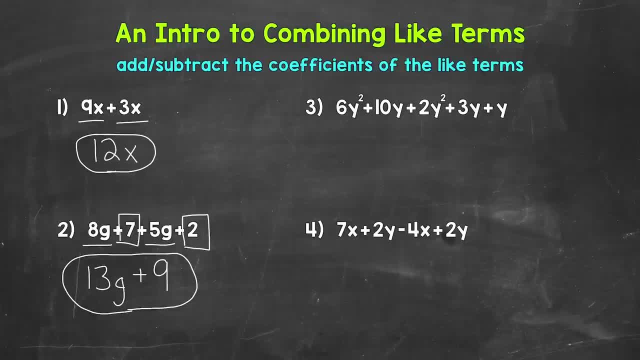 Let's move on to number three, where we have 6y squared plus 10y plus 2y squared plus 3y plus y. Let's find any like terms that we can combine. We'll start with 6y squared. 2y squared is a like term. 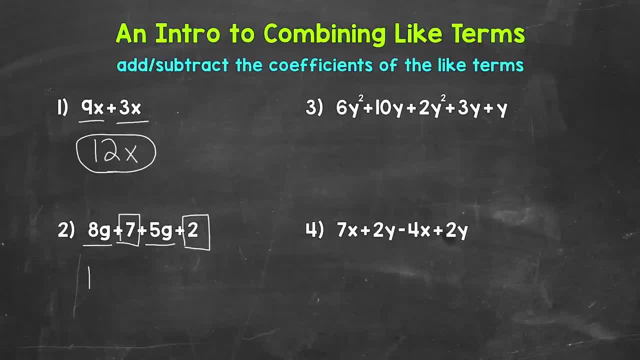 We have 8g plus 5g. That gives us 13g. And then we have 7 plus 2.. That gives us 9.. So we end up with 13g plus 9.. And that's our simplified expression. 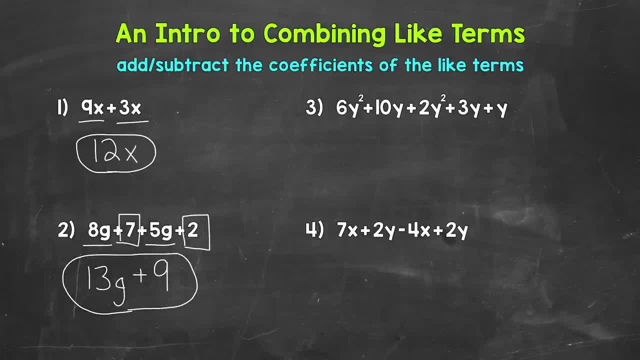 That expression of 13g plus 9 is equivalent to the original expression. We were just able to simplify the original expression by combining like terms. We started with four total terms, but we were able to combine like terms And now we only have two total terms. 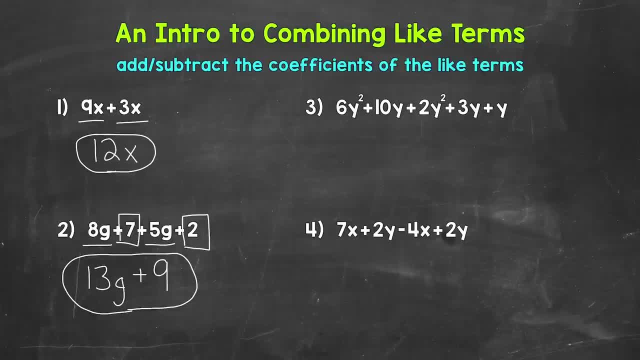 Let's move on to number three, where we have 6y squared plus 10y plus 2y squared plus 3y plus y. Let's find any like terms that we can combine. We'll start with 6y squared. 2y squared is a like term. 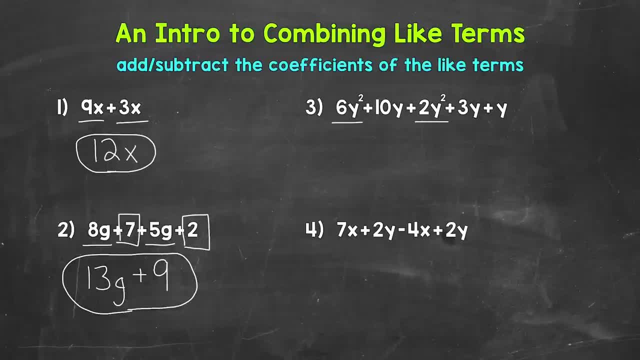 Both of those terms have that variable of y to the power of 2.. Now, do we have any other like terms within this algebraic expression that we can combine? Yes, 10y, And I will box these terms in in order to separate them from the y squared terms. 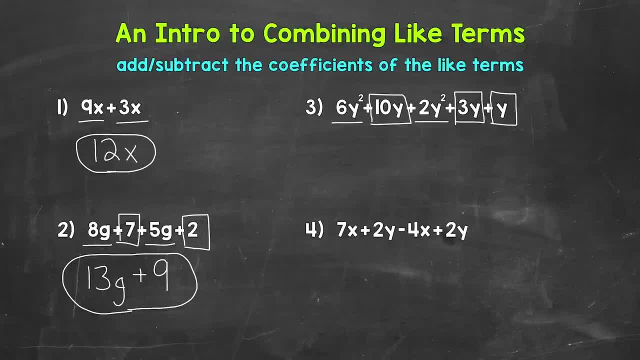 3y and then y. Now I do want to mention this term right here, The y. Of course we have to find the y squared by the variable by itself, The coefficient is 1.. We don't have a coefficient written in front. 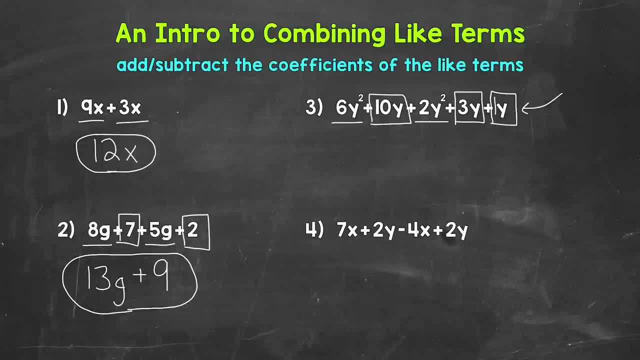 Whenever you see that the coefficient is 1. There is an understood 1 in front of a variable, It can be helpful to write that 1 in there. when you combine like terms, You can always write that 1 if you would like. 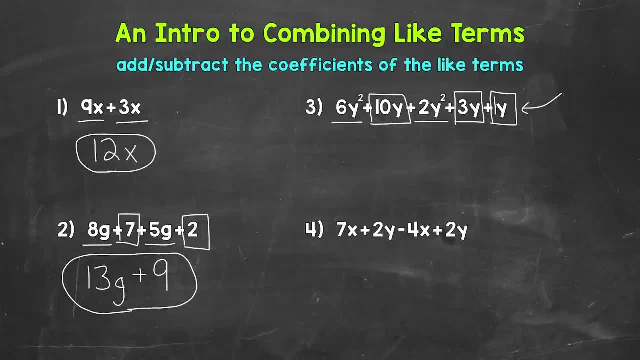 Now, since this algebraic expression has five terms and we are working with only two terms, working our way up to more complicated algebraic expressions, we're going to use a strategy to help us organize the expression. before we combine like terms, We are going to rearrange and rewrite the 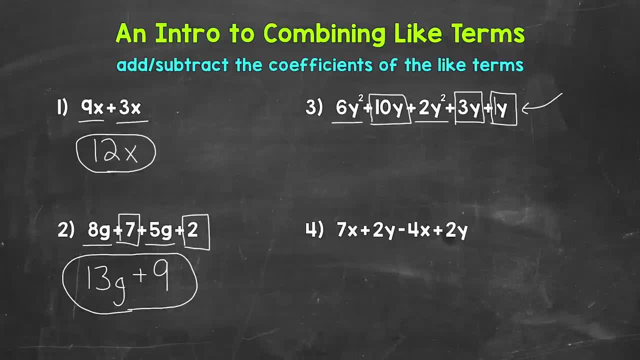 expression and put the like terms next to each other. I'll start with 6y squared plus the like term of 2y squared plus. now we have the y terms, so 10y plus 3y plus 1y, So now all of the like. 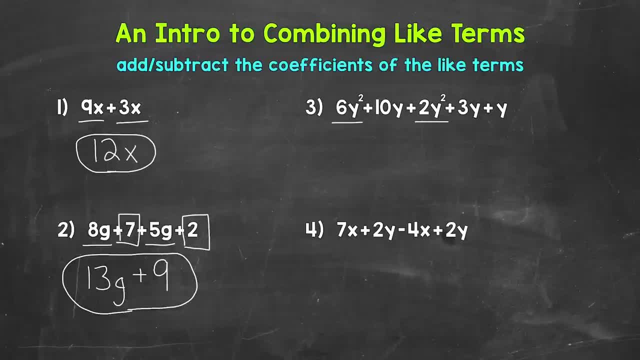 Both of those terms have that variable of y to the power of 2.. Now, do we have any other like terms within this algebraic expression that we can combine? Yes, 10y, And I will box these terms in in order to separate them from the y squared terms. 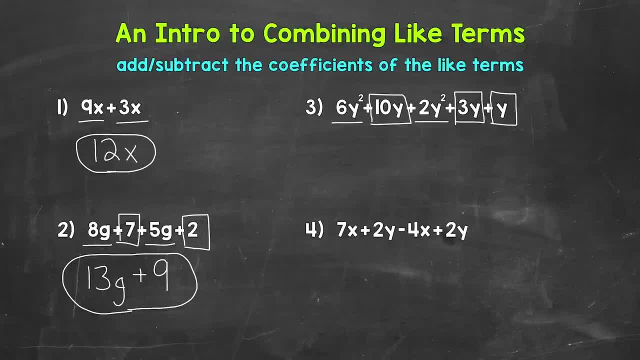 3y and then y. Now I do want to mention this term right here, The y. I put it in the first place because it's a variable of y. If I write this by the variable, by itself, the coefficient is 1.. 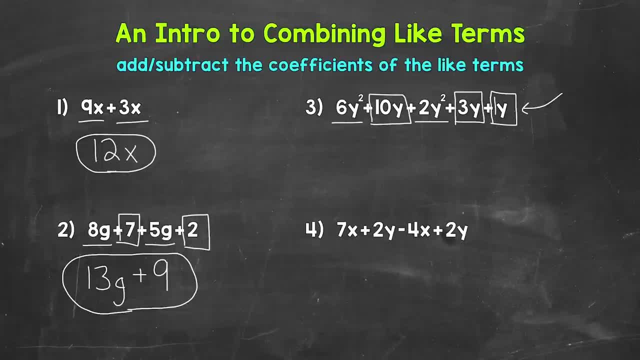 We don't have a coefficient written in front Whenever you see that the coefficient is 1.. There is an understood 1 in front of a variable And it can be helpful to write that 1 in there when you combine like terms. 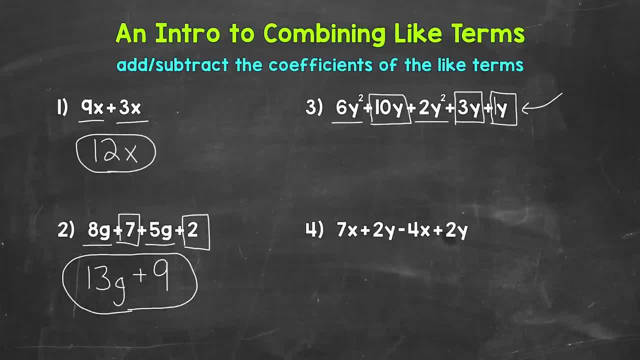 So you can always write that 1 if you would like. five terms and we are working our way up to more complicated algebraic expressions. we're going to use a strategy to help us organize the expression. before we combine like terms, We are going to rearrange and rewrite the expression and put the like terms next to. 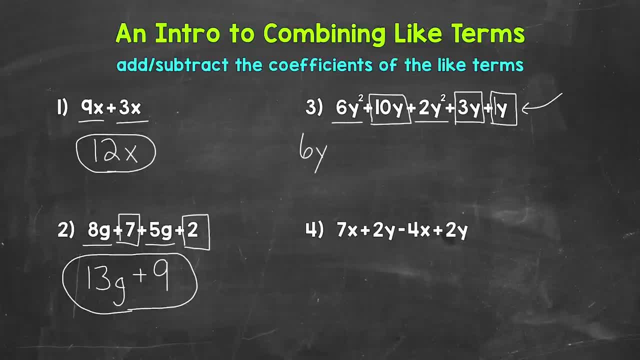 each other. I'll start with 6y squared plus the like term of 2y squared plus. now we have the y terms, so 10y plus 3y plus 1y. So now all of the like terms are next to each other and it's a little easier to see what. 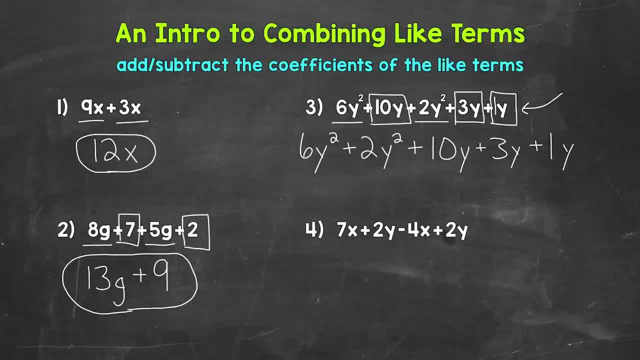 we can combine. So this is a strategy to keep in mind. Now, do you have to do this Step in order to combine like terms? No, but it can be helpful. Now we can combine like terms. We will start with 6y squared plus 2y squared. 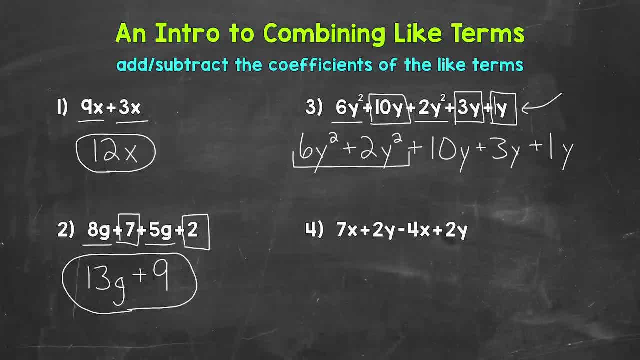 So add the coefficients: 6 plus 2 is 8, and then we have y squared plus. now we can combine the y terms, So we have 10 plus 3 plus 1.. 10 plus 3 plus 1.. 10 plus 3 is 13 plus 1 is 14.. 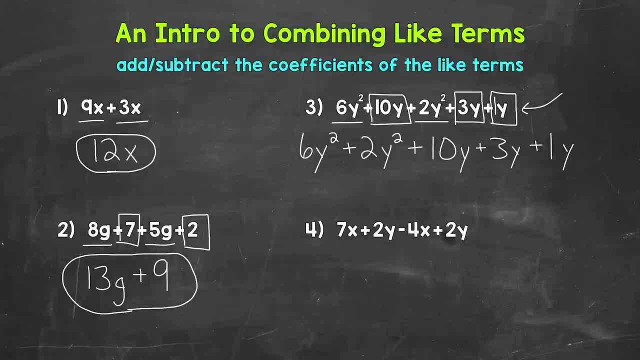 terms are next to each other and it's a little easier to see what we can combine. So this is a strategy to keep in mind. Now, do you have to do this step in order to combine like terms? No, but it can be helpful. 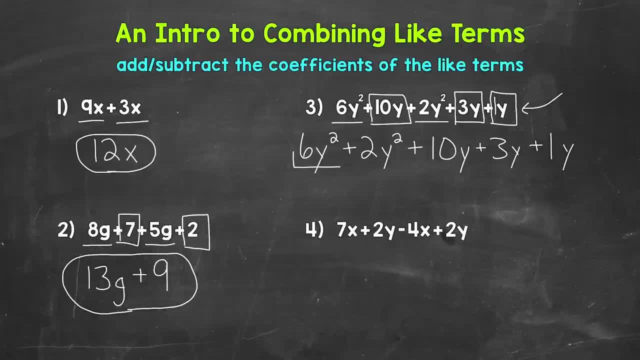 Now we can Combine like terms. We will start with 6y squared plus 2y squared, So add the coefficients: 6 plus 2 is 8, and then we have y squared plus. now we can combine the y terms, So we have 10 plus 3 plus 1.. 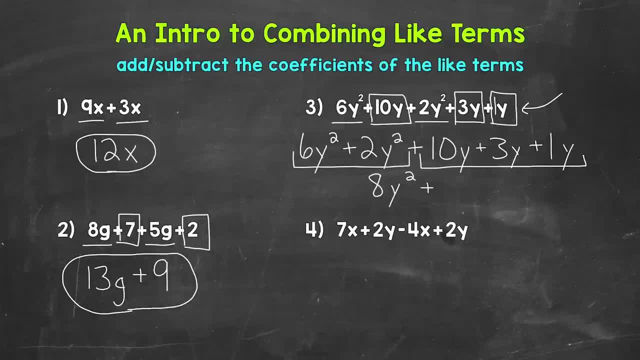 10 plus 3 is 13 plus 1 is 14.. So we get 8y, 8y squared plus 14y, And that's the simplified expression. We now have an equivalent expression that is simpler than the original. We simplified the expression. We went from 5 terms to 2 terms. 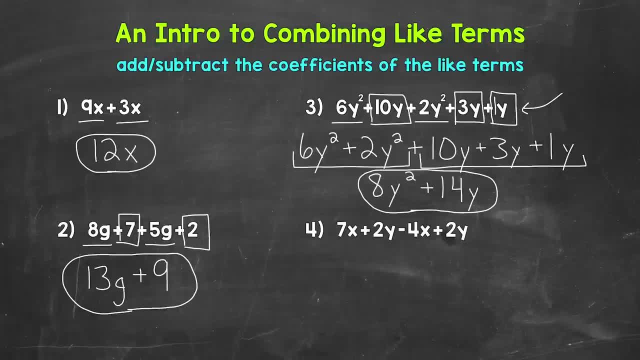 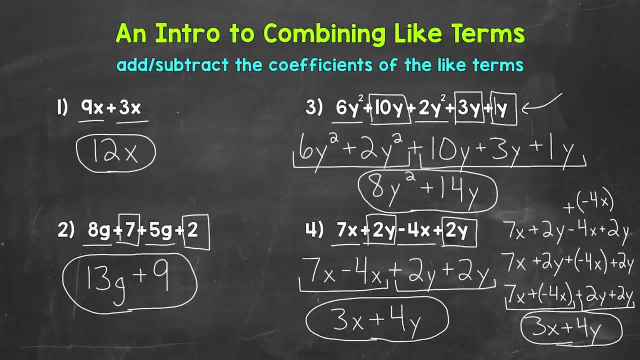 Let's move on to number 4, where we have 7x plus 2y minus 4x plus 2y. Let's find any like terms that we can combine. We will start with 7x plus 2y. 7x plus 2y minus 4x plus 2y. Let's find any like terms that we can combine. We will start with 7x plus 2y. 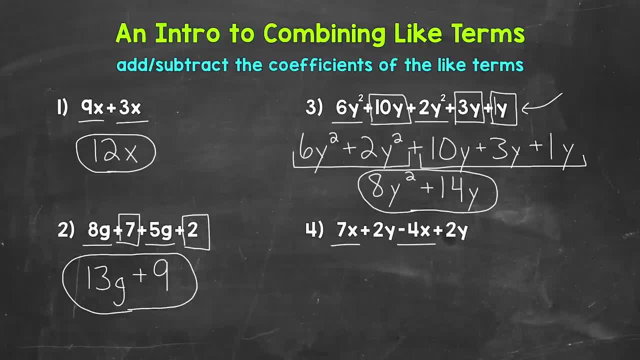 7x and negative 4x. Now, when we combine like terms, a term is going to take the sign that's in front of it, So this is negative 4x. Then we have 2y and 2y, So let's box those terms in in. 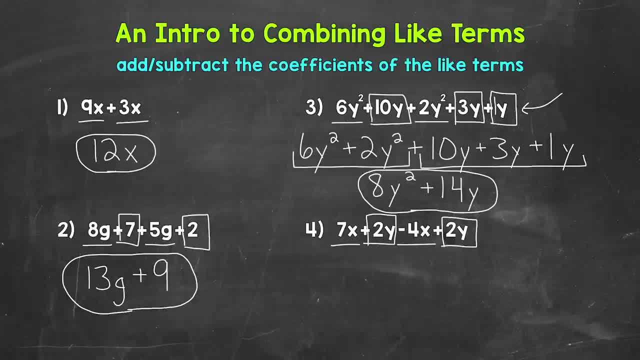 order to separate them from the x terms. Now we can rewrite this expression with the like terms next to each other. We will start with 7x, 7x minus 4x, So we have a negative 4x there. Make sure to bring the sign that's in front of. 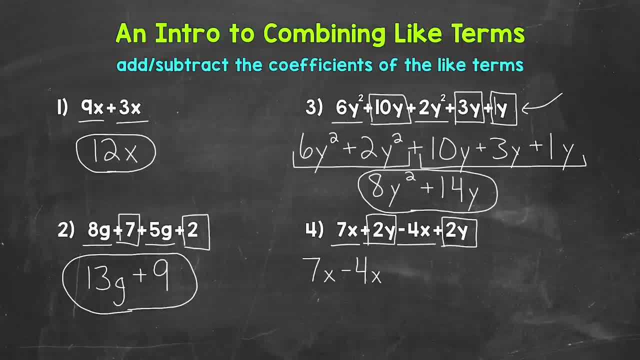 the term with it when we rewrite the expression Plus 2y. So now we have the y terms plus another 2y. Now we can combine like terms, So we have 7x minus 4x, Or you can think of this as 7x being. 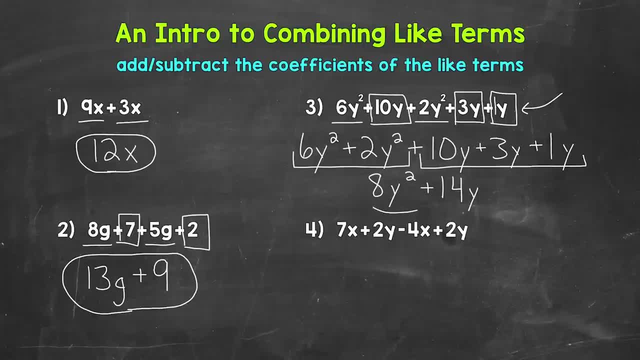 So we get 8y squared plus 14y, and that's the simplified expression. We now have an equivalent expression that is simpler than the original. We simplified the expression. We went from 5 terms to 2 terms. Let's move on to number 4, where we have 7x plus 2y minus 4x plus 2y. 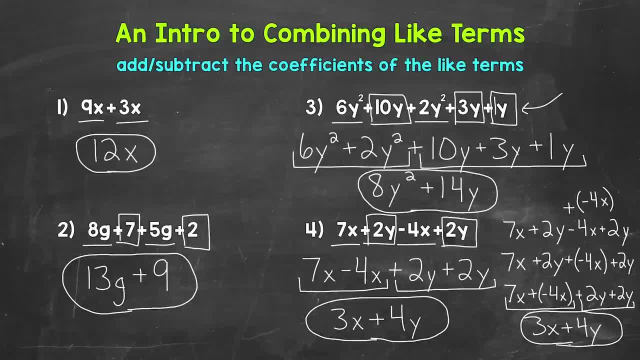 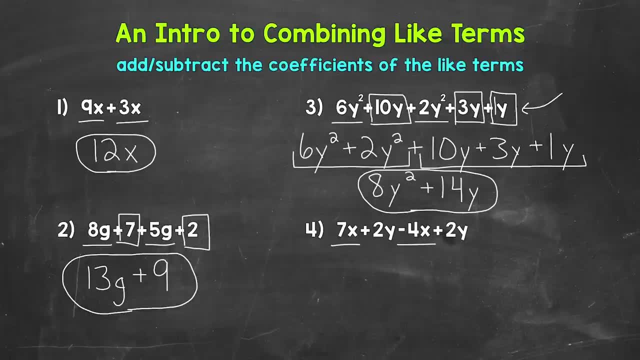 Let's find any like terms that we can combine. We will start with 7x and negative 4x. Now, when we combine like terms, a term is going to take the sign that's in front of it. So this is negative 4x. 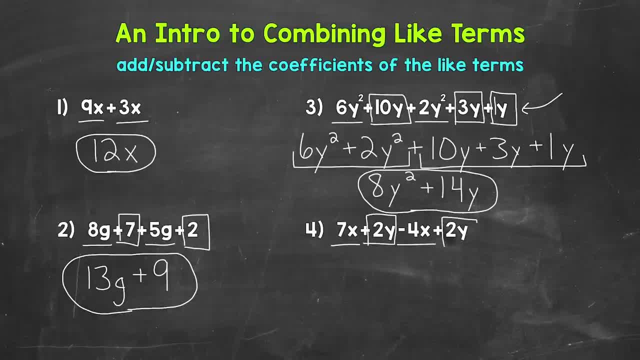 Then we have 2y and 2y, So let's box those terms in in order to separate them from the x terms. Now we can rewrite this expression. Let's start with the like terms next to each other. We will start with 7x minus 4x. 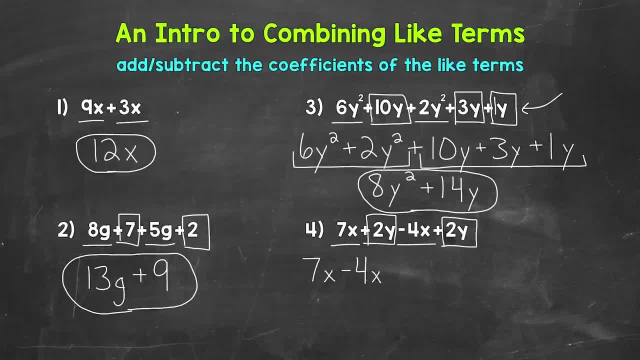 So we have a negative 4x there. Make sure to bring the sign that's in front of the term with it when we rewrite the expression Plus 2y. So now we have the y terms plus another 2y. Now we can combine like terms. 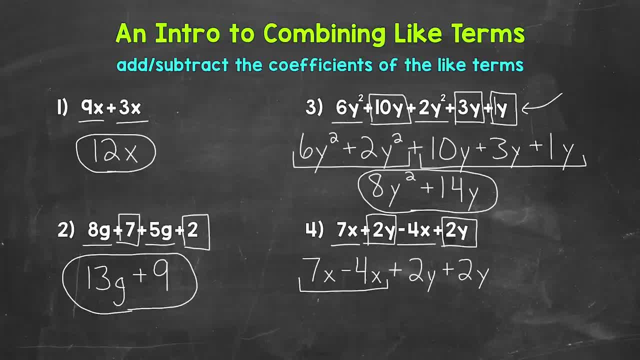 So we have 7x minus 4x, Or you can think of this as 7x being combined with negative 4x. however you want to think about it, 7 minus 4 is 3.. And then we have the x. 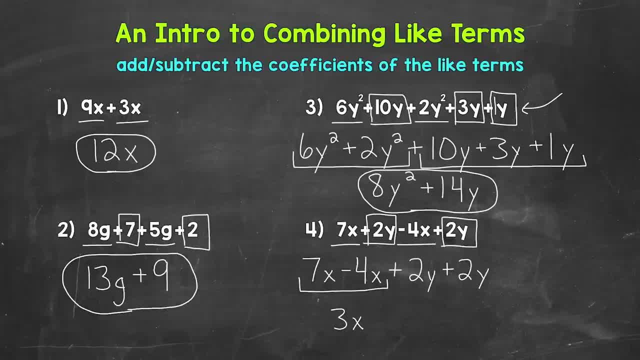 Or if you're thinking about it as 7x combined with a negative 4x, 7 and negative 4 give us 3 as well. Then we have our 2y plus 2y. That gives us plus 2y. 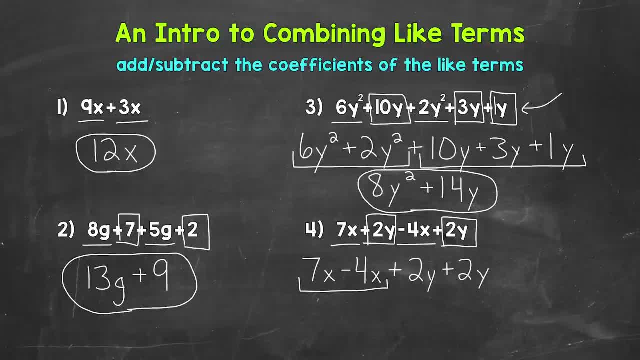 combined with negative 4x. So we have 7x minus 4x. So we have 7x minus 4x. So we have 7x minus 4x. However you want to think about it, 7 minus 4 is 3.. And then we have the x, Or, if you're, 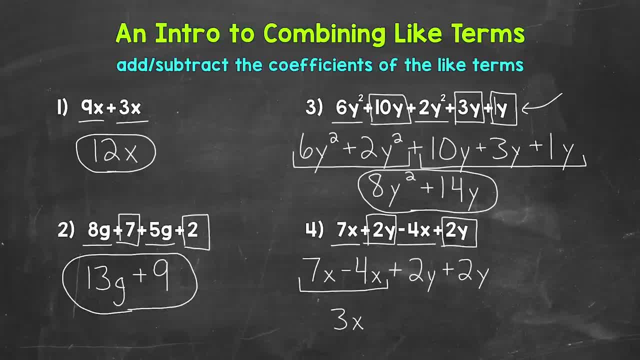 thinking about it as 7x combined with a negative 4x. 7 and negative 4 give us 3 as well. Then we have our 2y plus 2y. That gives us plus 4y, So we end up with 3x plus 4y, And then we have the. 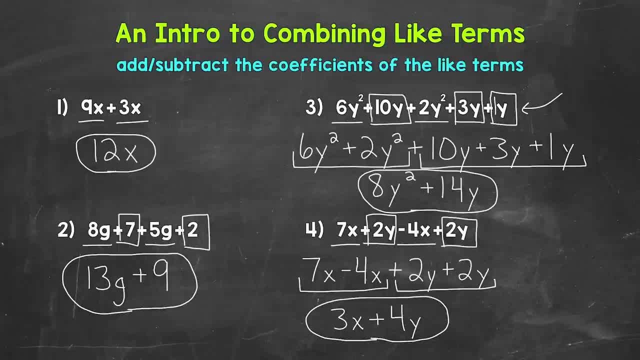 y, And that's our simplified expression. We went from 4 total terms to 2 total terms by combining like terms. 3x plus 4y is equivalent to the original expression. We were just able to again simplify this expression by combining like terms. Now I also want to go through simplifying this. 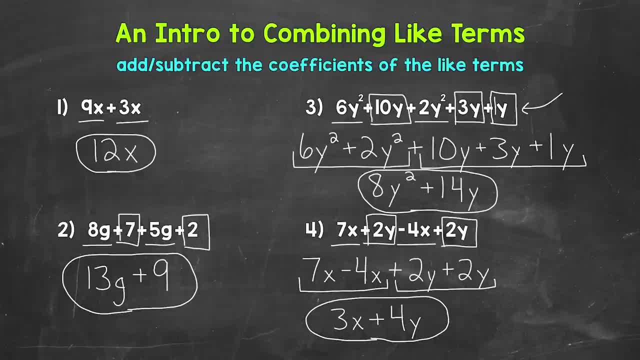 expression a slightly different way to start off, And that's by rewriting the original expression with only addition, separating the terms. We do this by changing any subtraction to adding the opposite. The benefit of having all terms separated only by addition is that it's a little simpler to identify all of the terms. 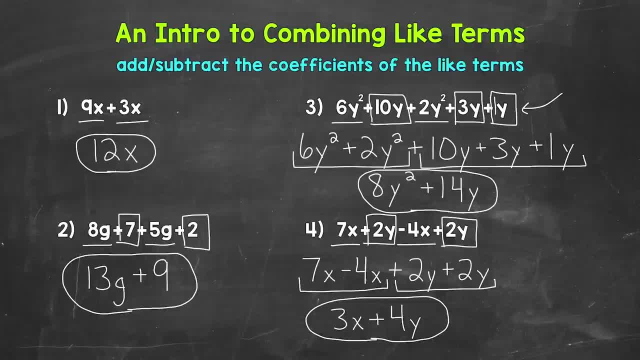 especially any negative terms. It kind of organizes the expression and helps any negatives stand out. I'll rewrite the expression off to the side here, So 7x plus 2y minus 4x plus 2y. So let's rewrite subtraction as adding the opposite, So adding the opposite of a positive. 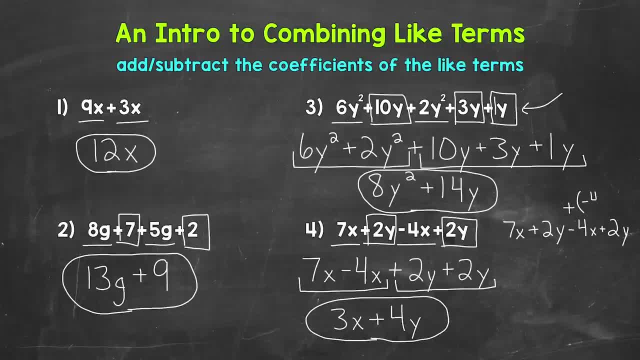 4x is a negative 4x, So adding the opposite. Let's rewrite the expression with that change, So we have 7x plus 2y plus negative 4x plus 2y. Let's rewrite that expression with like terms next to each other, So 7x plus negative 4x plus. 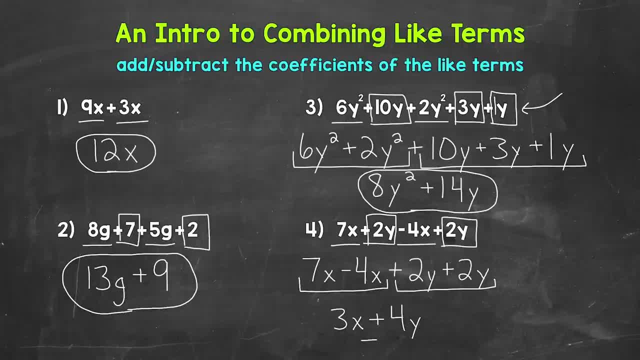 Plus 4y, So we end up with 3x plus 4y And that's our simplified expression. We went from 4 total terms to 2 total terms by combining like terms. 3x plus 4y is equivalent to the original expression. 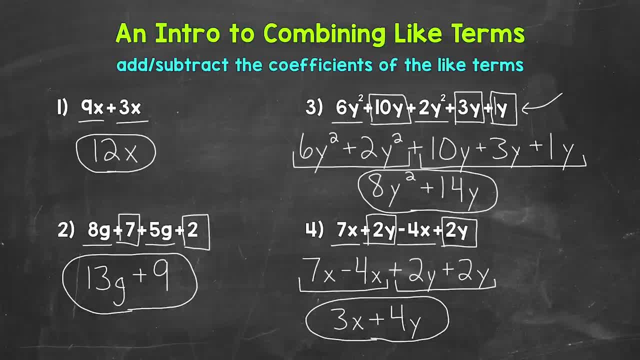 We were just able to again simplify this expression by combining like terms. Now I also want to go through simplifying this expression a slightly different way to start off, And that's by rewriting the original expression with only addition, separating the terms. We do this by changing any subtraction to adding the opposite. 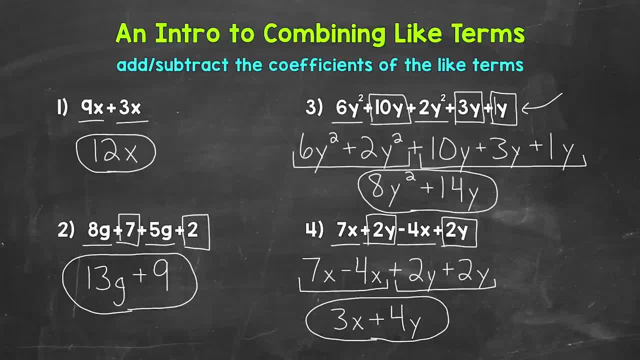 The benefit of having all terms separated only by addition is that it's a little simpler to identify all of the terms, especially any negative terms. It kind of organizes the expression and helps any negatives stand out. I'll rewrite The expression off to the side here. 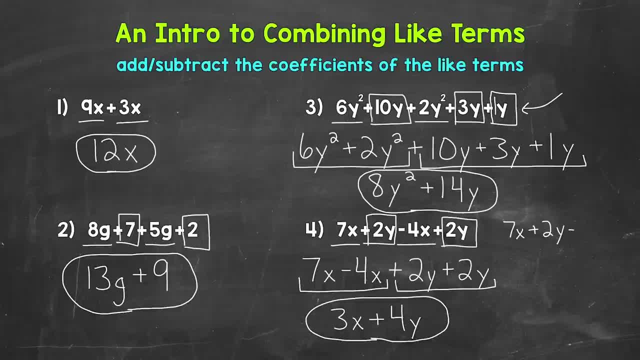 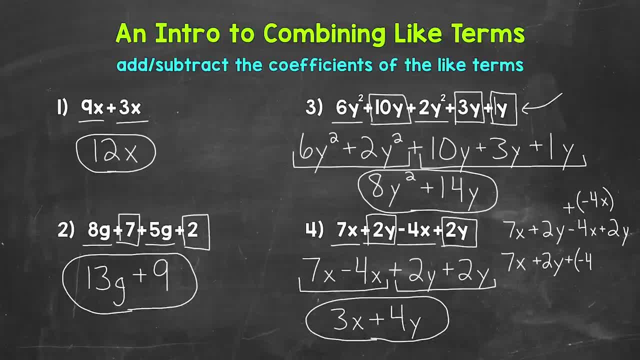 plus 4x plus 2y minus 4x plus negative 4x plus 2y, So 2y will be negative 4x plus 4x. Other letter here is negative: 4x plus 4x plus 2y. 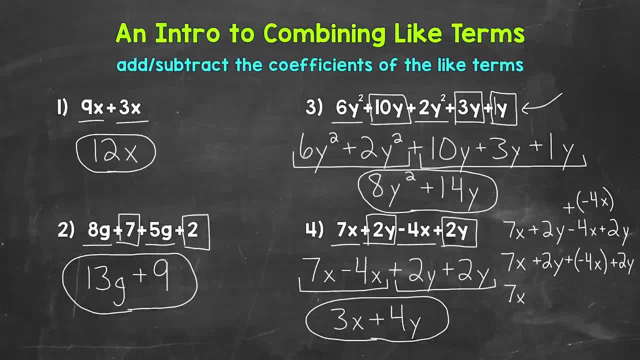 Let's rewrite that expression with like terms next to each other. Now we have 7x plus negative 4x plus 2y plus 2y. Now we can combine like terms: We have 7x plus negative 4x plus 2y. 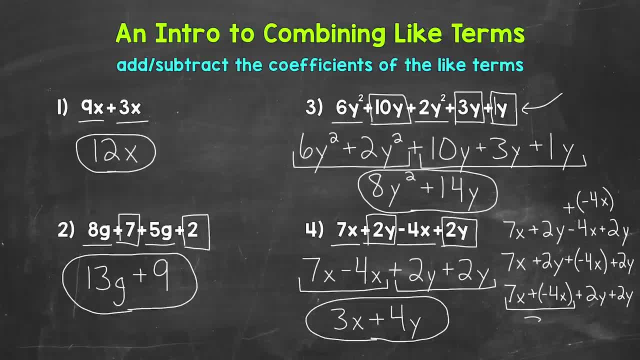 Let's write the expression in the same order: plus negative 4x. that gives us 3x. And then we have 2y plus 2y. so that gives us plus 4y, 3x plus 4y- that way as well. So that's just another strategy to be aware of. 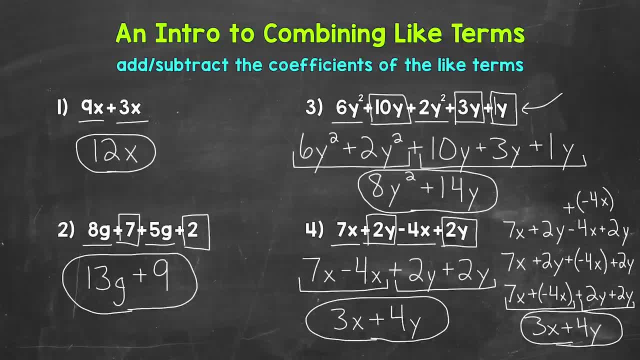 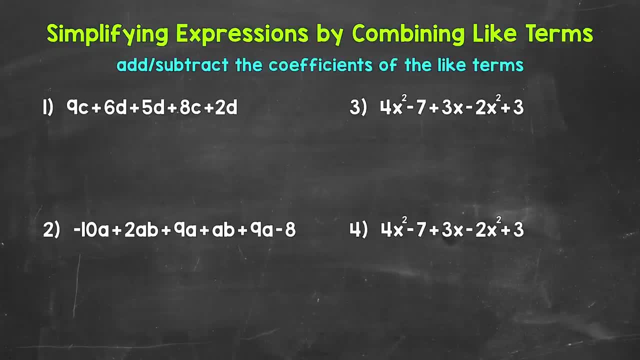 So there's an introduction to combining like terms. Let's take a look at more examples. Here are more examples of algebraic expressions that we will simplify by combining like terms. Let's jump into number one, where we have 9c plus 6d plus 5d plus 8c plus 2d. 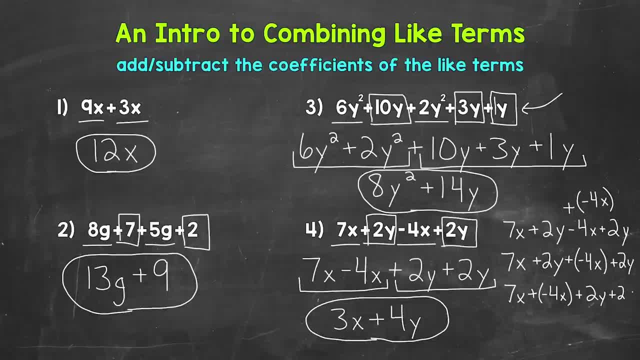 2y plus 2y. Now we can combine like terms: We have 7x plus negative 4x. That gives us 3x. And then we have 2y plus 2y, So that gives us plus 4y, 3x plus 4y That way as well. So that's just another strategy to be aware of. 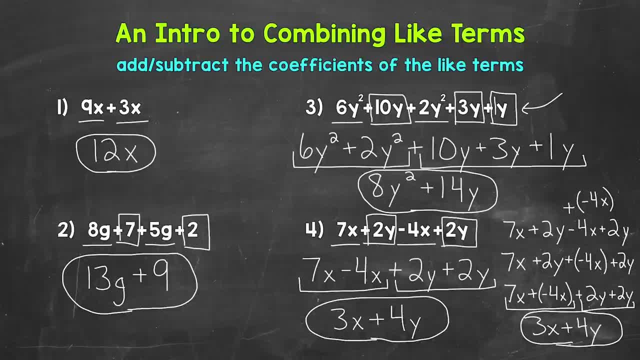 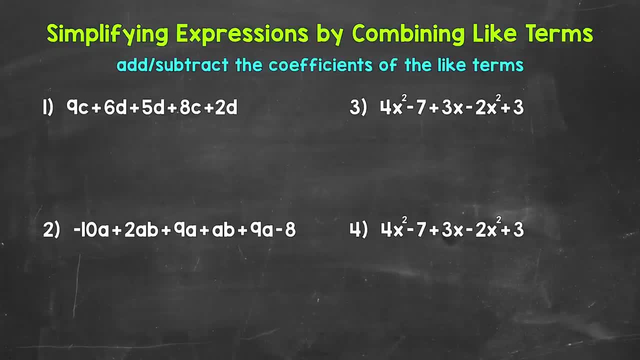 So there's an introduction to combining like terms. Let's take a look at more examples. Here are more examples of algebraic expressions that we will simplify by combining like terms. Let's jump into number one, where we have 9c plus 6d plus. 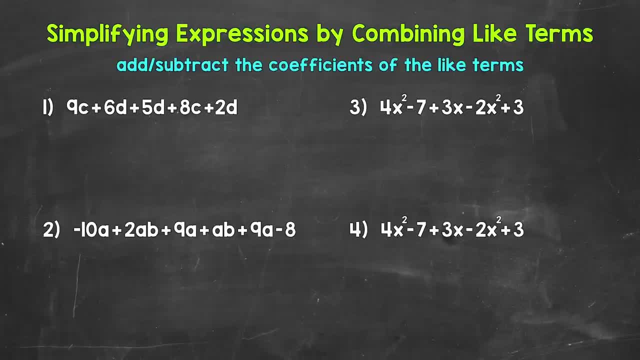 5d plus 8c plus 2d. The first thing that we need to do is identify any like terms that we can combine. So are there any like terms that we can combine in this expression? Yes, Let's start with 9c and 8c. Both of those terms have the same variable, to the same power. Both terms have the 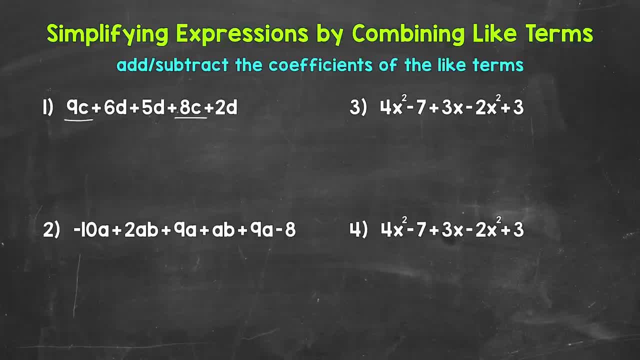 same variable of c to the same understood power of 1.. So they are like terms. Remember, when we don't have an exponent attached to a variable, there is an understood exponent of 1.. Something is to the power of 1.. Anything to the power of 1 is just. 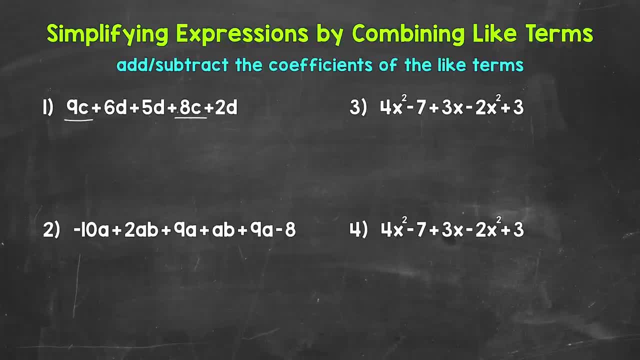 itself. Do we have any other like terms that we can combine? Yes, We have 6d, 5d and 2d. All of those terms have the same variable of d to the same understood power of 1.. So let's box. 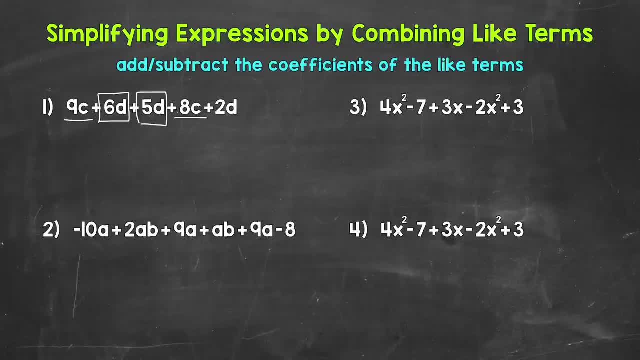 Those terms in in order to separate them from the other terms. Are there any other like terms that we can combine? No, All of the like terms have been identified. So what we can do now, we can rewrite this expression with the like terms next to each other, By rewriting this expression. 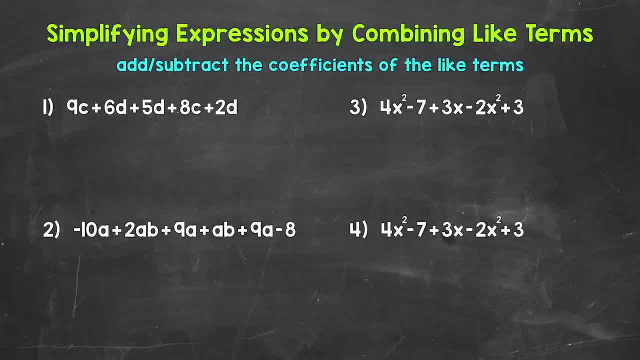 The first thing that we need to do is identify any like terms that we can combine. So, are there any like terms that we can combine in this expression? Yes, Let's start with 9c and 8c. Both of those terms have the same variable to the same power. 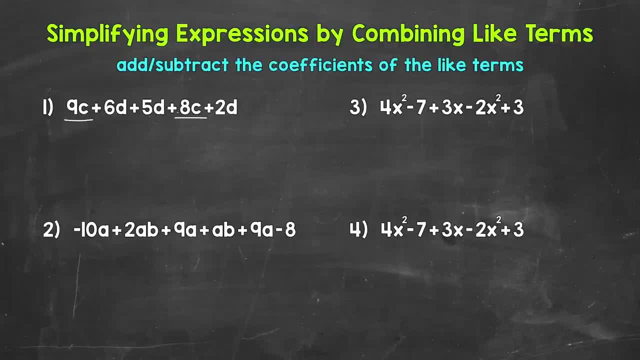 Both terms have the same variable of c to the same understood power of 1.. So they are like terms. Remember, when we don't have an exponent attached to a variable, there is an understood exponent of 1.. Something is to the power of 1.. 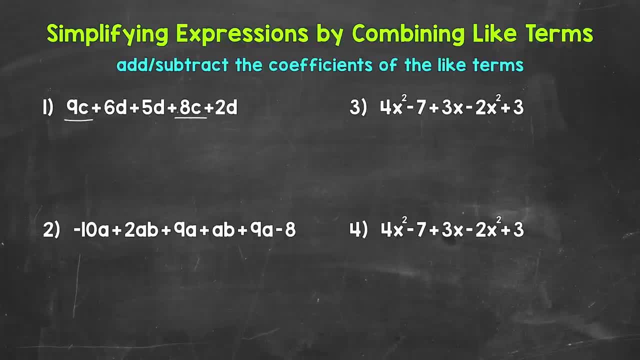 Anything to the power of 1 is just itself. Do we have any other like terms that we can combine? Yes, We have 6d, 5d and 2d. All of those terms have the same variable of d to the same understood power of 1.. 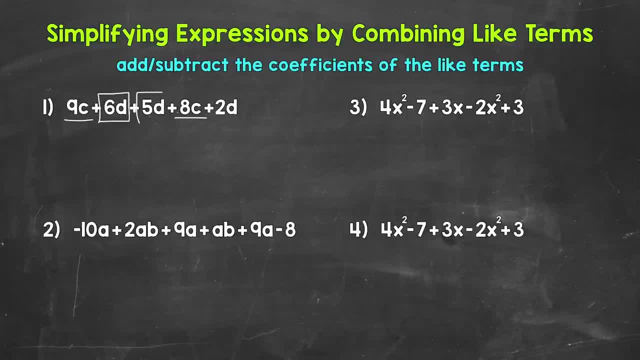 So let's box those terms in in order to separate them from the other terms. Are there any other like terms that we can combine? No, All of the like terms have been identified. So what we can do now, we can rewrite this expression with the like terms next to each other. 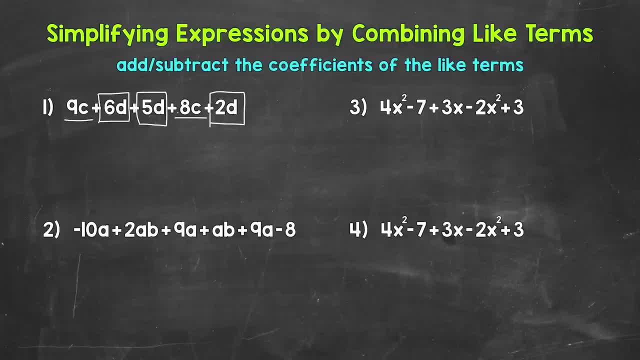 By rewriting this expression with all of the like terms next to each other. this will help us organize the expression. It will make combining like terms a little simpler. We have 9c plus 8c plus 6d plus 5d plus 5d. 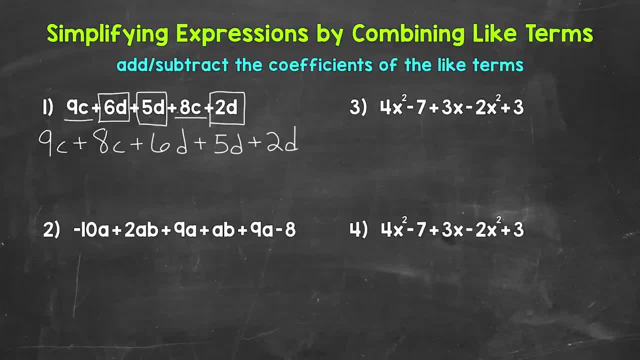 Plus 2d. So now all of the like terms are next to each other And it's a little easier to see what we need to combine. So this is a strategy to keep in mind. Now do we have to do this step in order to combine like terms? 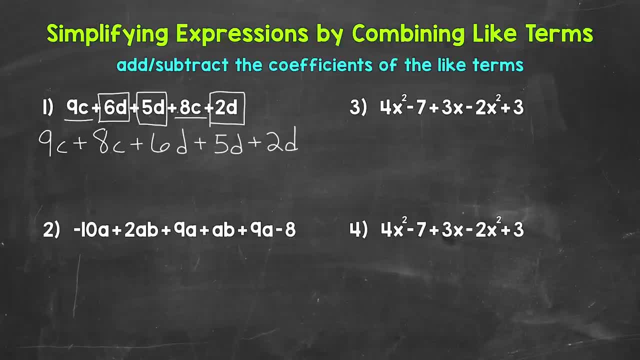 No, But it can be helpful. Now we can combine like terms. Let's start with 9c and 8c, So we have 9c plus 8c. We need to add the coefficients, The numbers in front of the variables. 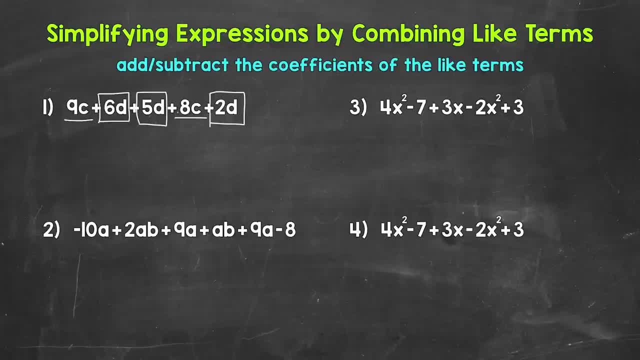 with all of the like terms next to each other. this will help us organize the expression. It will make combining like terms a little simpler. We have 9c plus 8c plus 6d plus 5d plus 2d, So now 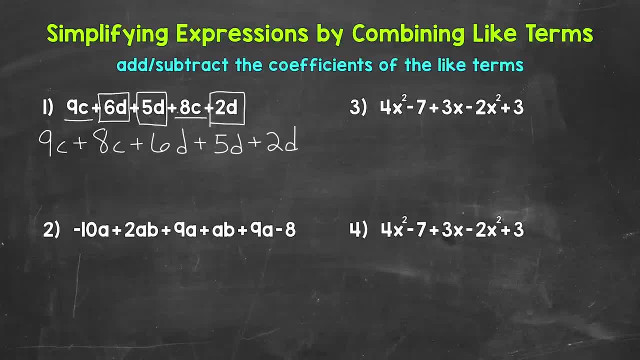 all of the like terms are next to each other and it's a little easier to see what we need to combine. So this is a strategy to keep in mind. Now, do we have to do this step in order to combine like terms? No, But it can be helpful. Now we can combine like terms. Let's start with. 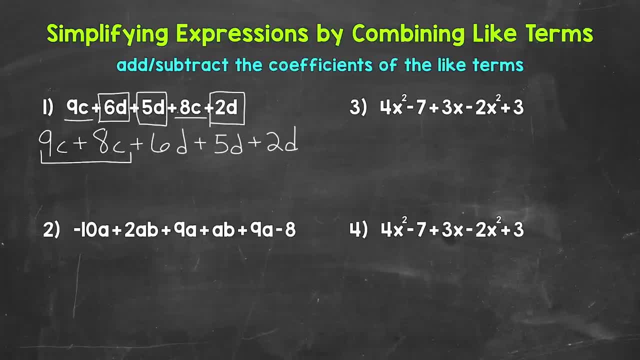 9c and 8c, So we have 9c plus 8c. We need to add the coefficients, the numbers in front of the variables, So we have 9 plus 8, which is 17.. So we have 17c plus and now we can combine these terms. 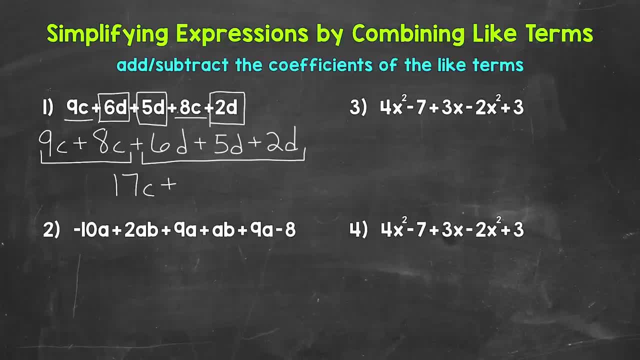 So we have 6d plus 5d plus 2d. 6 plus 5 is 11 plus 2 is 13.. So we have 13d, And this is our final simplified expression: 17c plus 13d. Now, 17c plus 13d is equivalent to the original expression. 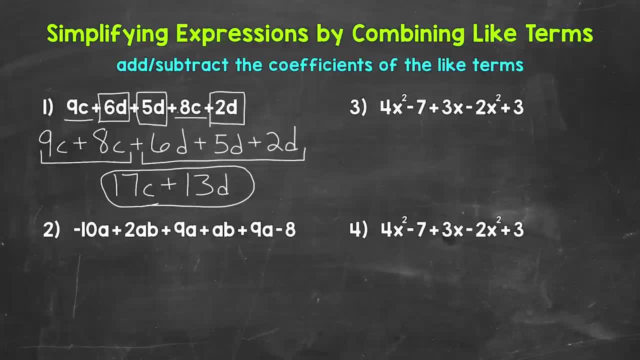 We went from 5 total terms in the original expression, simplified it to two total terms by combining like terms. Let's move on to number two, where we have negative 10a plus 2ab plus 9a plus ab plus 9a minus 8.. Let's start by identifying any like. 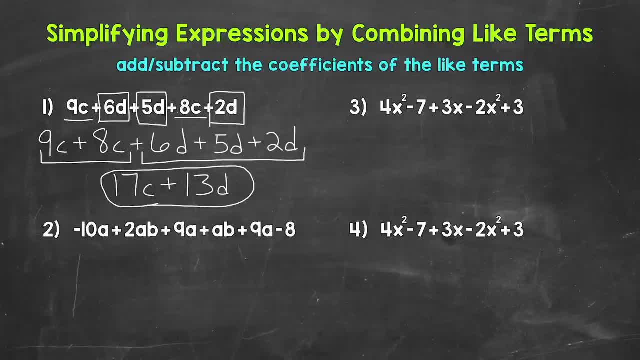 terms that we can combine. So do we have any like terms that we can combine? Yes, We have negative 9a and another 9a. All three of those terms have the same variable to the same power, The variable of a to the understood power of one. Do we have any other like terms that we can combine? Yes, We. 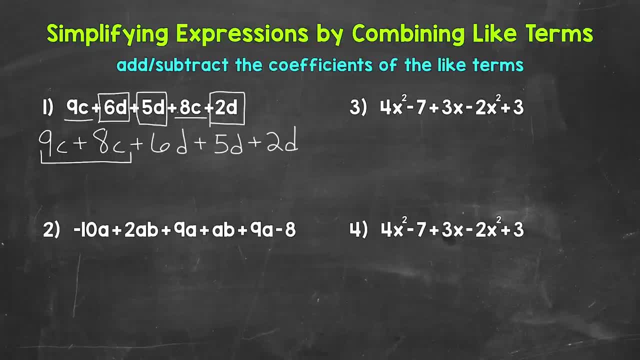 So we have 9 plus 8, which is 17.. So we have 17c plus, And now we can combine these terms, So we have 6d plus 5d plus 2d. 6 plus 5 is 11.. 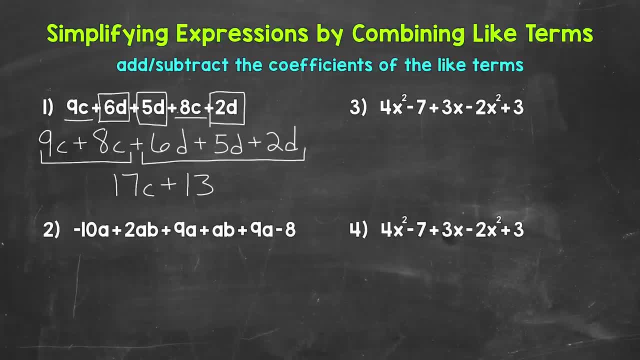 Plus 2 is 13.. So we have 13d, And this is our final simplifier Expression: 17c plus 13d. Now 17c plus 13d is equivalent to the original expression. We went from 5 total terms in the original expression. 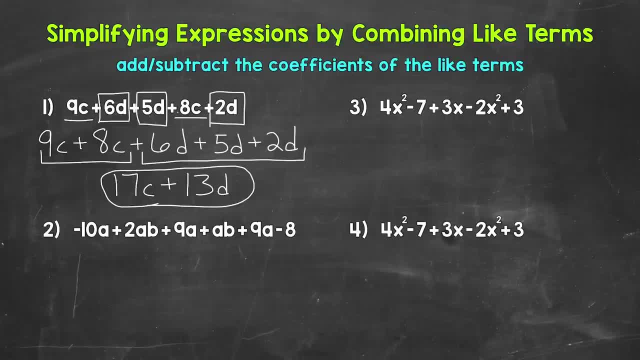 And simplified it to 2 total terms By combining like terms. Let's move on to number 2.. Where we have negative 10a plus 2ab Plus 9a plus ab Plus 9a minus 8.. Let's start by identifying any like terms that we can combine. 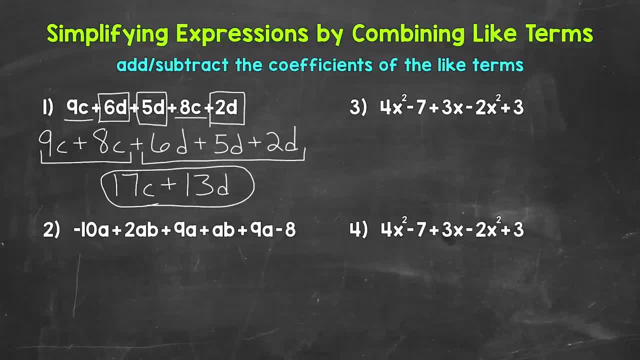 So do we have any like terms that we can combine? Yes, We have negative 10a And 9a And another 9a. All three of those terms have the same variable to the same power, The variable of a to the understood power of 1.. 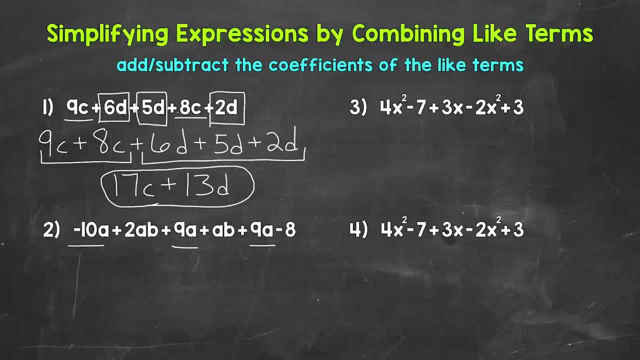 Do we have any other like terms that we can combine? Yes, We have 2ab. Let's box these in in order to separate them, And then ab. Now, this term right here, ab- does not have a coefficient written in front. Whenever we see this, there is an understood coefficient of 1.. 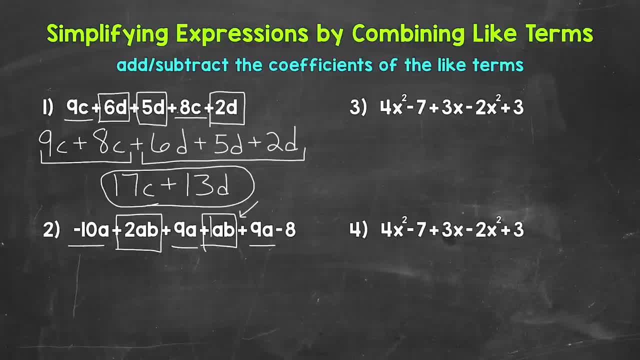 So this is 1ab And we're able to write that one in as the coefficient, And it's helpful to do so when combining like terms. That way you know you need to combine that one. Are there any other like terms within this expression that we can combine? 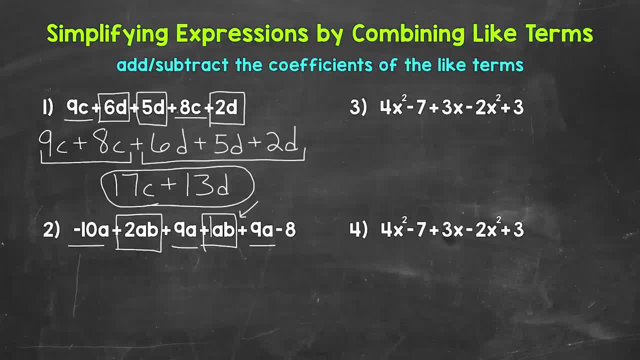 No, But we do have one more term: Negative 8.. So we have a constant term of negative 8. And I'll circle that term in order to separate it. Even though we don't have anything to combine it with, We still need to include it in the simplified expression. 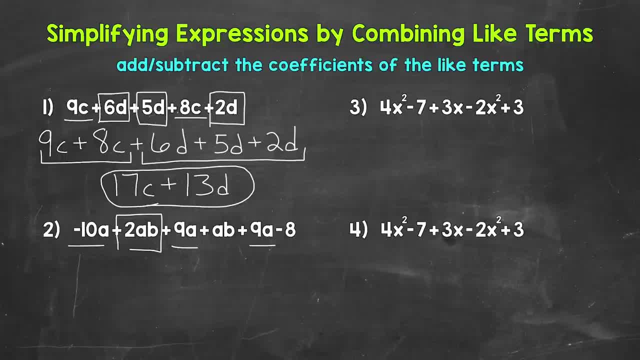 have 2ab. Let's box these in in order to separate them. And then ab- Now this term right here, ab does not have a coefficient written in front. Whenever we see this, it is an understood coefficient of 1.. So this is 1ab And we're able to write that one in. 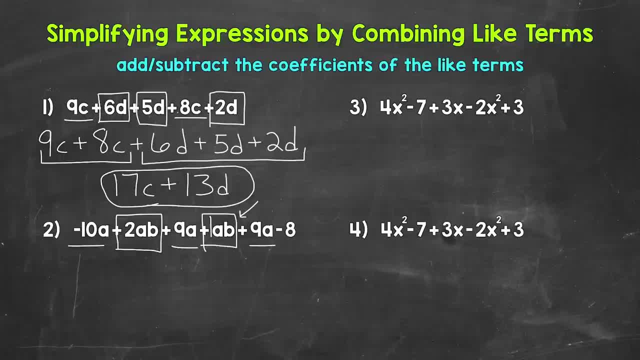 as the coefficient, And it's helpful to do so when combining like terms. That way, you know you need to combine that one. Are there any other like terms within this expression that we can combine? No, But we do have one more term: negative 8.. So we have a constant term of negative 8.. And 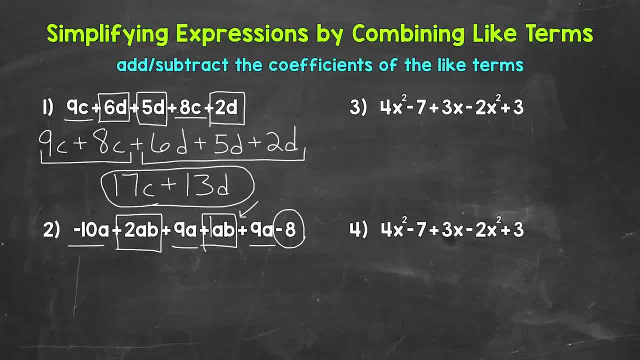 I'll circle that term in order to see it. So we have negative 8. And we have negative 8. And we need to separate it. Even though we don't have anything to combine it with, we still need to include it in the simplified expression, And that is negative 8.. Remember, a term will take the sign. 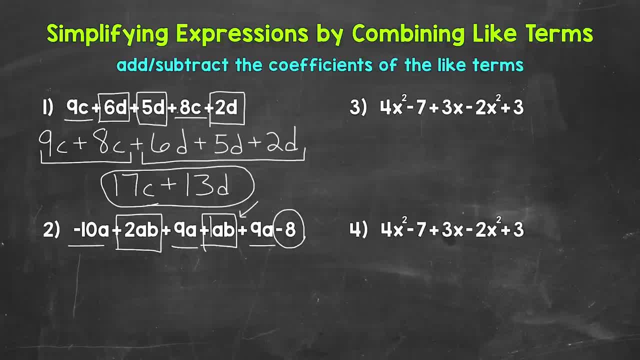 that's in front of it. So we have negative 8 and negative 10a within this expression. Now we can rewrite this expression with the like terms next to each other. We have negative 10a plus 9a plus 2ab plus 1ab minus 8.. Now we can combine like terms. Let's start with negative 10a plus 9a plus. 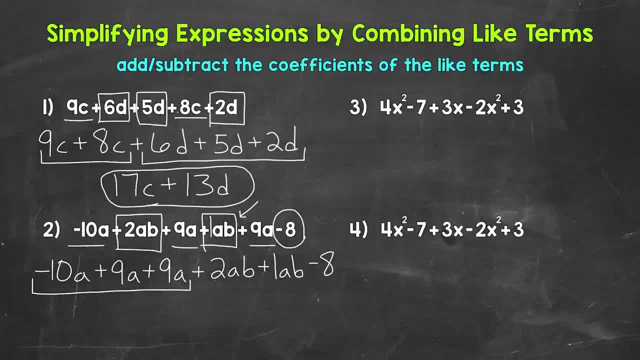 9a Negative. 10 plus 9 is negative. 1 plus 9 is 8.. A positive 8.. So we have 8a. And then plus 2ab plus 1ab, 2 plus 1 is 3.. So we have 3ab. And then, lastly, we have a negative 8 or 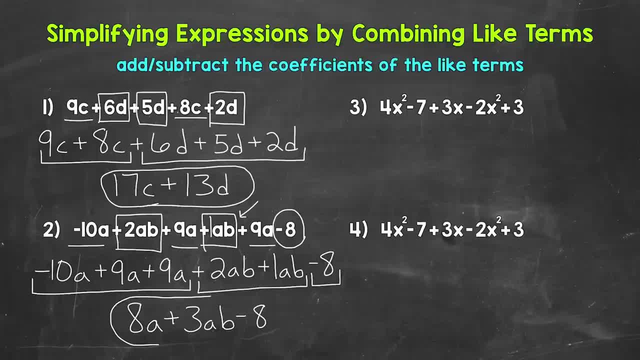 minus 8 here. So 8a plus 3ab minus 8 is our final simplified expression. We went from 6 total terms in the original expression to 3 total terms in the simplified expression, And then we have the simplified expression by combining like terms. Let's move on to numbers 3 and 4, where we 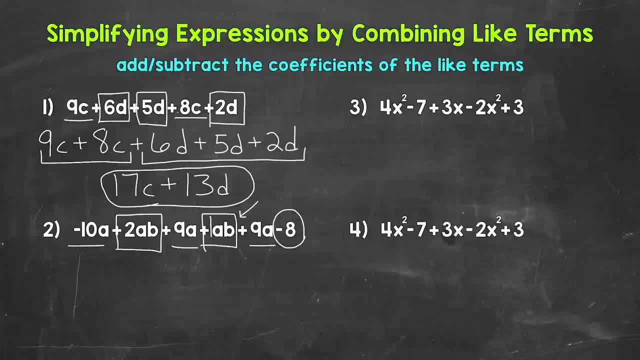 And that is negative 8.. Remember, A term will take the sign that's in front of it, So we have negative 8 and negative 10a within this expression. Now we can rewrite this expression with the like terms next to each other. 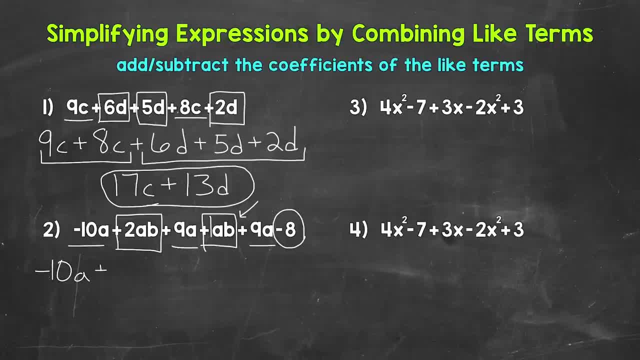 We have negative 10a plus 9a plus 9a plus 2ab plus 1ab Minus 8.. Now we can combine like terms. Let's start with negative 10a plus 9a plus 9a. 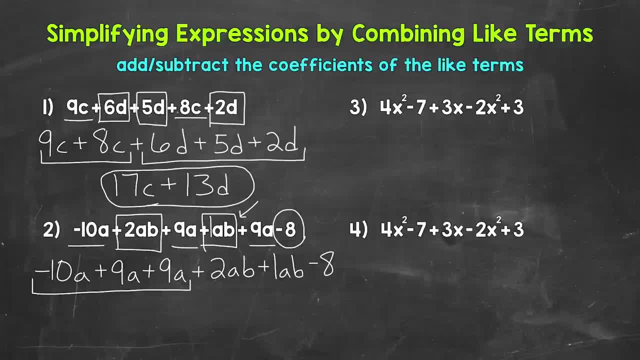 Negative. 10 plus 9 is negative: 1. Plus 9 is 8.. A positive 8.. So we have 8a. And then plus 2ab, plus 1ab. 2 plus 1 is 3. So we have 3ab. 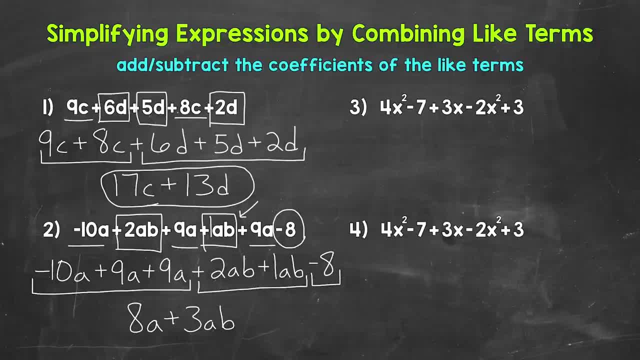 And then, lastly, we have a negative 8 or minus 8 here. So 8a plus 3ab minus 8 is our final simplified expression. We went from 6 total terms in the original expression To 3 total terms in the simplified expression by combining like terms: 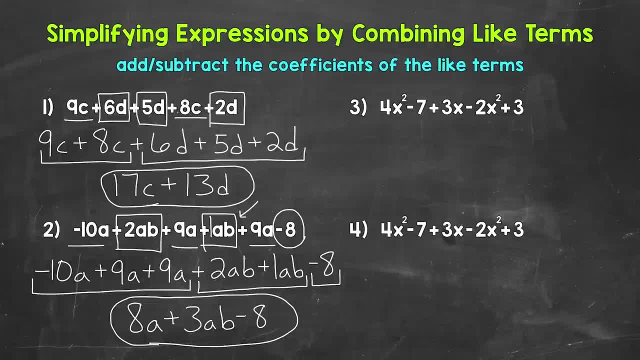 Let's move on to numbers 3 and 4. Where we actually have the same exact expression: 4x squared minus 7 plus 3x minus 2x squared plus 3.. We're going to go through this two slightly different ways. 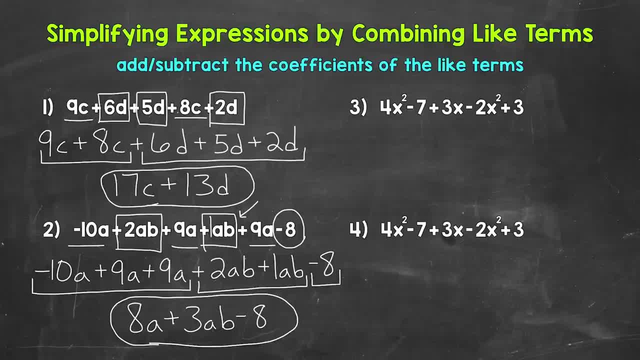 First we will go through simplifying the expression as it currently is, And that's for number 3.. For number 4, we're going to rewrite the expression, So all of the terms are separated only by addition. We will talk more about that strategy once we get to number 4.. 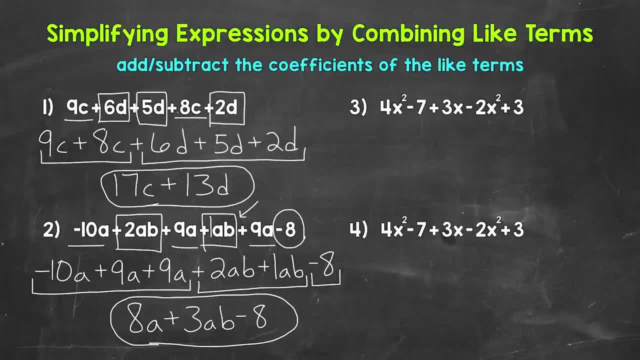 actually have the same exact expression: 4x squared minus 7 plus 3x minus 2x squared plus 3.. We're going to go through this two slightly different ways. First, we will go through simplifying the expression as it currently is, And that's for number 3.. For number 4,: 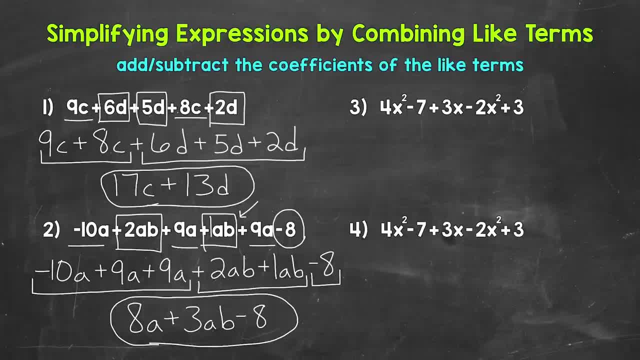 we're going to rewrite the expression, So all of the terms are separated only by addition. We will talk more about that strategy once we get to number 4.. Let's start number 3 by identifying any like terms. So do we have any like terms that we can combine? Yes, we have 4x squared and negative 2x squared- Both of these. 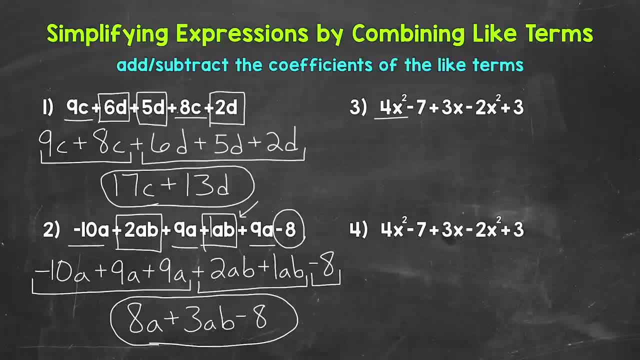 terms have the same variable of x to the same power of 2.. So 4x squared and negative 2x squared. Remember, a term takes the sign that's in front of it, So that's negative 2x squared. Do we have? 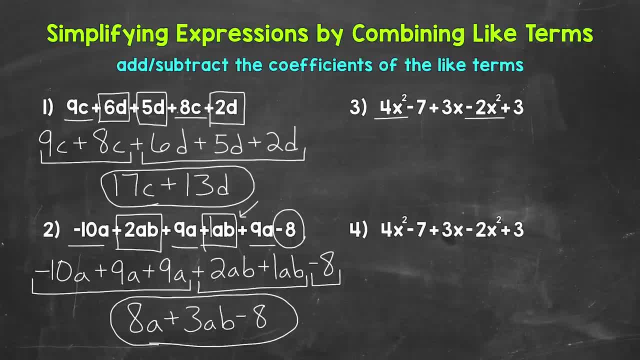 any other like terms that we can combine. Yes, we have two constant terms, negative, 7 and 3. I'll box those terms in in order to separate them. And then, lastly, we have 3x. We don't have any. 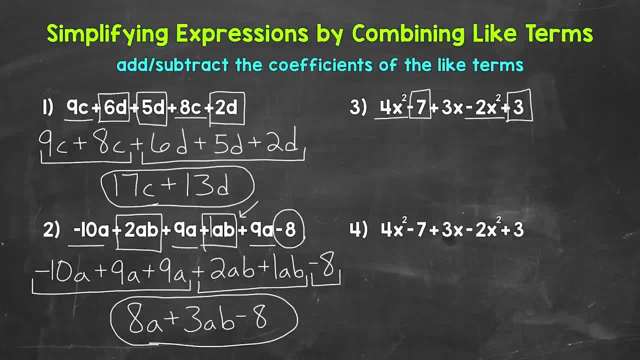 like terms to combine 3x with, but I will circle it in order to separate them. Now we can rewrite this expression with the like terms next to each other. Remember, bring the sign that's in front of the term with it as you rewrite this expression. So we have 4x. 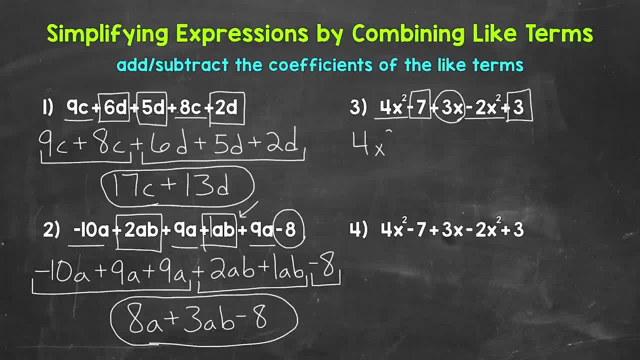 squared and then negative. 2x squared is the like term, So this is going to be 4x squared minus 2x squared. Then we have plus 3x And then our constant terms last. So we have minus 7, a negative 7 plus 3.. 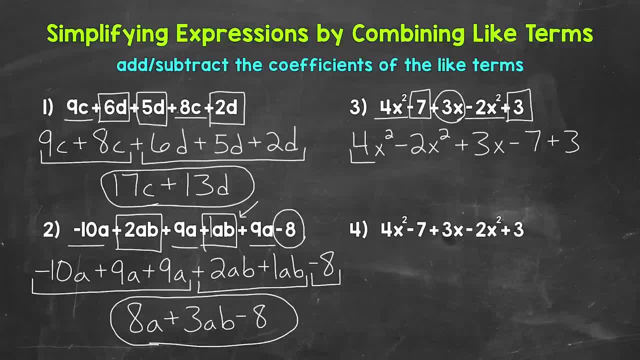 Now we can combine like terms. We have 4x squared minus 2x squared, Or you can think of this as combining 4x squared and negative 2x squared. However you want to think about it, you'll get the same thing either way. Let's subtract the coefficients, We have 4 minus 2, which 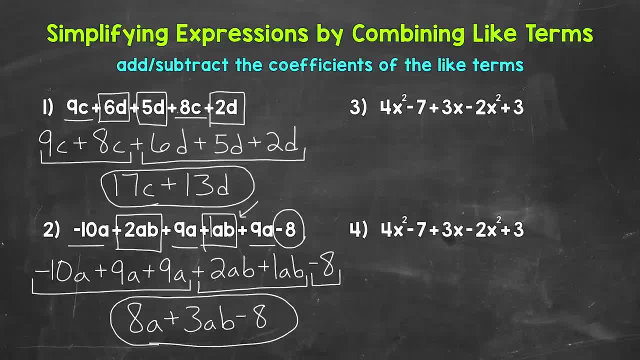 Let's start number 3 by identifying any like terms. So do we have any like terms that we can combine? Yes, we have 4x squared and negative 2x squared. Both of these terms have the same variable of x to the same power of 2.. 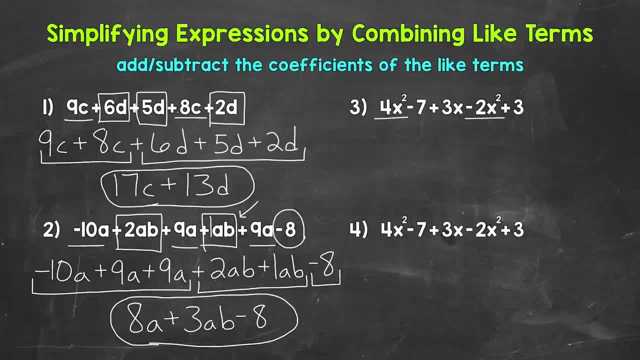 So 4x squared and negative 2x squared. Remember, a term takes the sign that's in front of it, So that's negative 2x squared. Do we have any other like terms that we can combine? Yes, we have two constant terms. 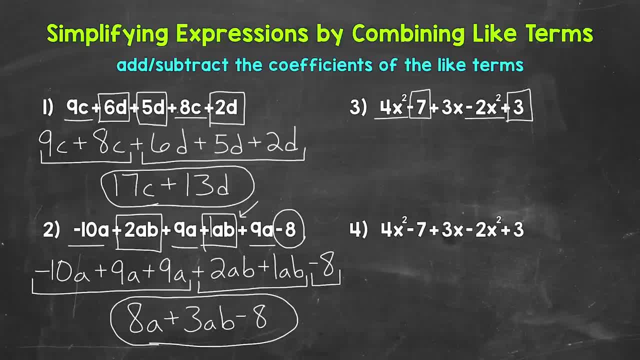 Negative 7 and 3.. I'll box those terms in in order to separate them. And then, lastly, we have 3x. We don't have any like terms to combine 3x with, But I will circle it in order to separate it from the other terms. 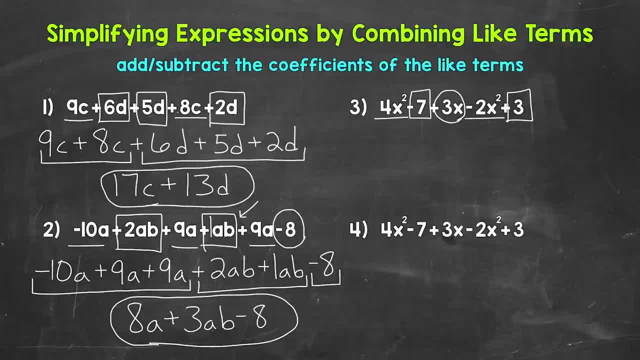 Now we can rewrite this expression with the like terms next to each other. Remember, bring the sign that's in front of the term with it as you rewrite this expression. So we have 4x squared And then negative 2x squared is the like term. 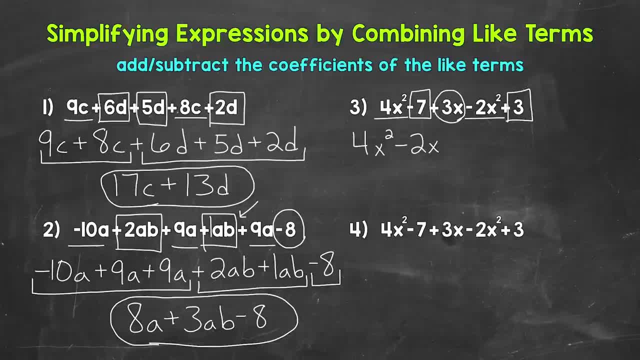 So this is going to be 4x squared minus 2x squared, Then we have plus 3x And then our constant terms last. So we have minus 7.. A negative 7 plus 3.. Now we can combine like terms: 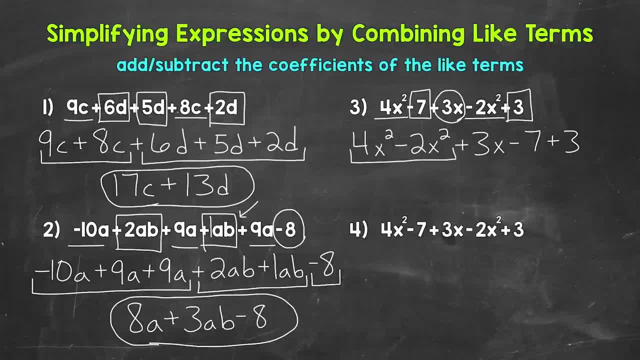 We have 4x squared minus 2x squared, Or you can think of this as combining 4x squared and negative 2x squared. However you want to think about it, you'll get the same thing either way. Let's subtract the coefficients. 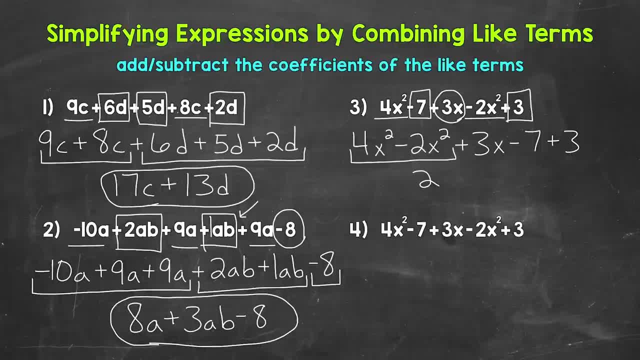 4 minus 2, which gives us 2.. Or if you thought about it as 4 combined with negative 2, that gives us 2 as well. So this is 2x squared, Then we have plus 3x, And then we can combine negative 7 and 3.. 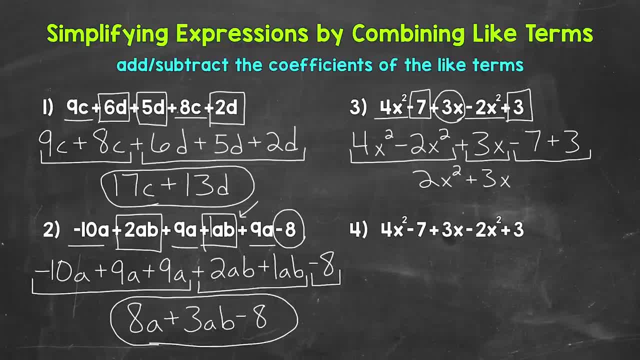 Positive 3.. So we have negative 7 plus 3. That gives us negative 4.. So our final simplified expression is 2x squared plus 3x minus 4.. We went from 5 total terms in the original expression to 3 total terms by combining like terms: 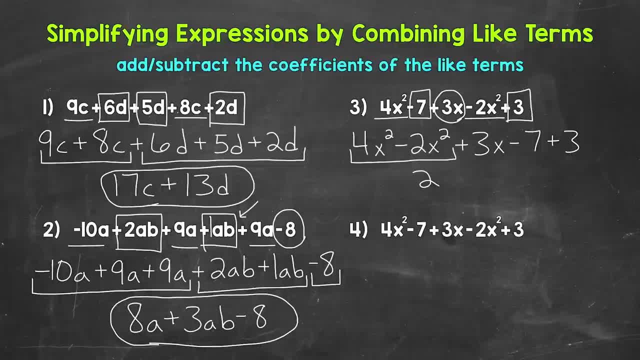 gives us 2.. Or if you thought about it as 4 combined with negative 2,, that gives us 2 as well. So this is 2x squared, Then we have plus 3x, And then we can combine negative 7 and 3,. 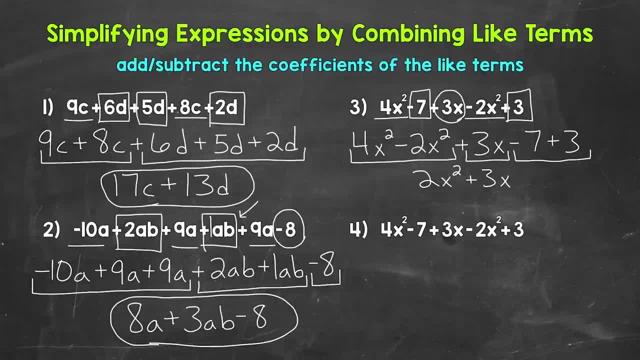 positive 3.. So we have negative 7 plus 3.. That gives us negative 4.. So our final simplified expression is 2x squared plus 3x minus 4.. We went from 5 total terms in the original expression to 3 total terms by combining like terms. Let's move on to number 4, where we 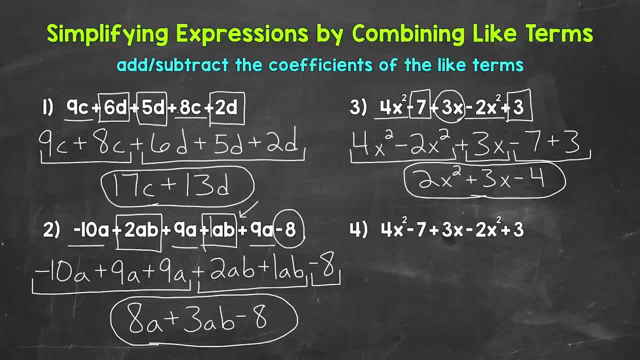 will take a look at a strategy we can use when we have subtraction or negatives involved in the expression. We're going to rewrite the original expression by combining like terms With only addition separating the terms. The benefit of having all terms separated only by addition is that it's a little simpler to identify all of the terms, especially any negative terms. 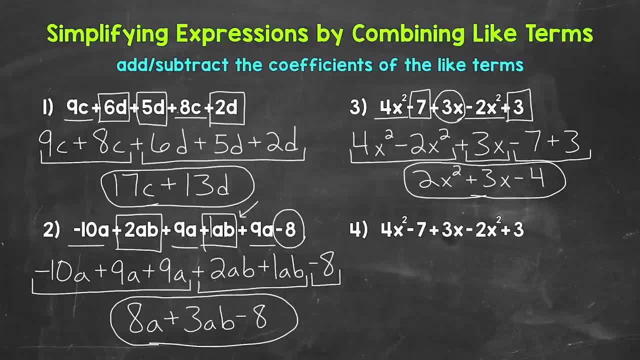 It kind of organizes the expression and helps any negatives stand out. Now do you have to use this strategy? No, but it can be helpful. So I wanted to at least go over it. So let's rewrite this expression with only addition, separating the terms. We do this by adding the opposite, So change any subtraction to. 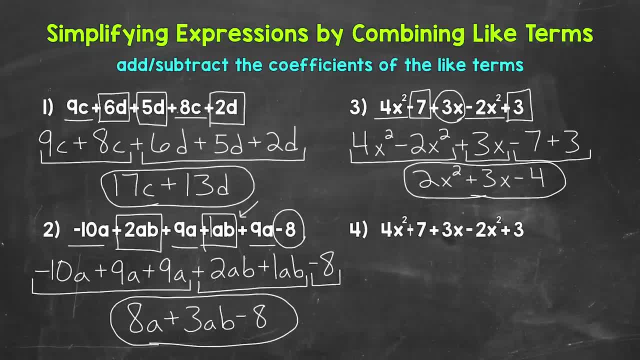 adding the opposite. Let's change this to addition, And then the opposite of positive 7 is negative 7.. So add the opposite. Then let's add the opposite here as well. So the opposite of positive 2x squared is negative 2x squared. So let's rewrite this with those changes. 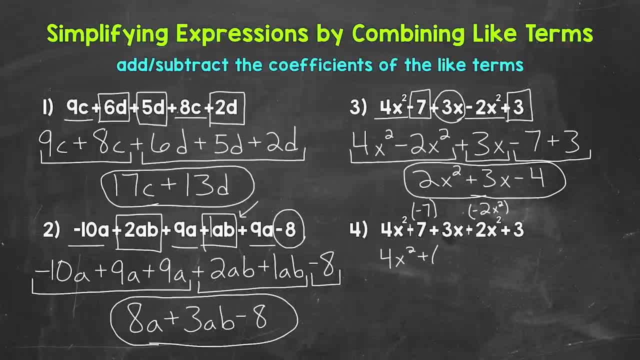 So we have 4x squared plus negative, 7 plus 3x plus negative, 2x squared plus 3.. So now all of the terms are separated only by addition. Now we can identify any like terms. We have 4x squared and. 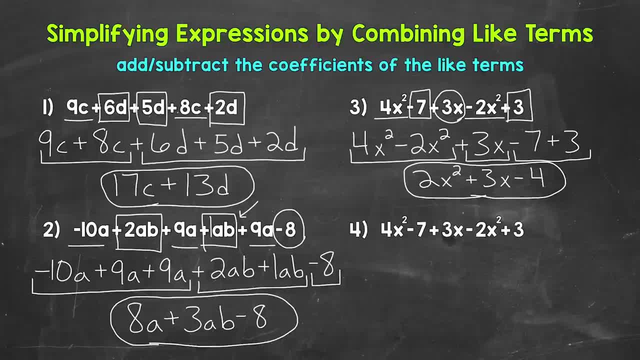 Let's move on to number 4, where we will take a look at a strategy we can use when we have subtraction or negatives involved in the expression. We're going to rewrite the original expression With only addition, separating the terms. The benefit of having all terms separated only by addition is that it's a little simpler to identify all of the terms. 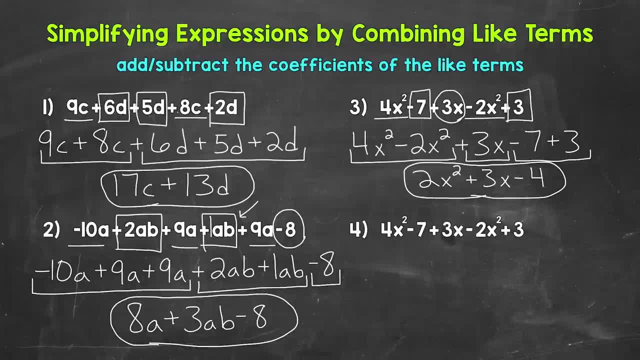 Especially any negative terms. It kind of organizes the expression and helps any negatives stand out. Now do you have to use this strategy? No, but it can be helpful. So I wanted to at least go over it. So let's rewrite this expression. 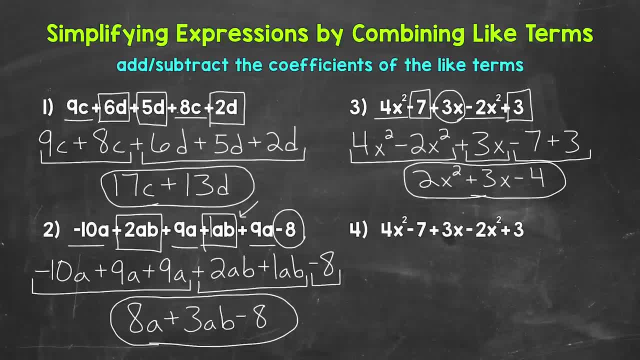 With only addition, separating the terms. We do this by adding the opposite. So change any subtraction to adding the opposite. Let's change this to addition, And then the opposite of positive 7 is negative 7.. So add the opposite. Then let's add the opposite here as well. 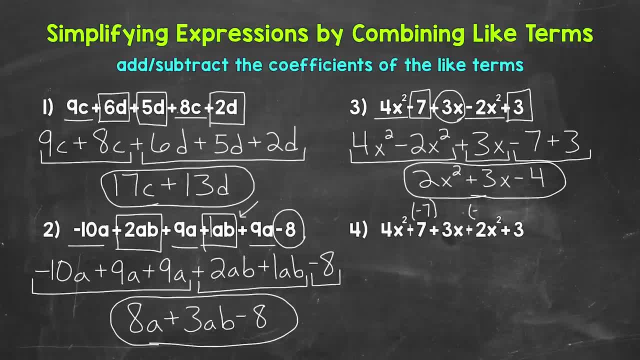 So the opposite of positive 2x squared is negative 2x squared. Let's rewrite this with those changes. So we have 4x squared plus negative, 7 plus 3x plus negative, 2x squared plus 3.. So now all of the terms are separated only by addition. 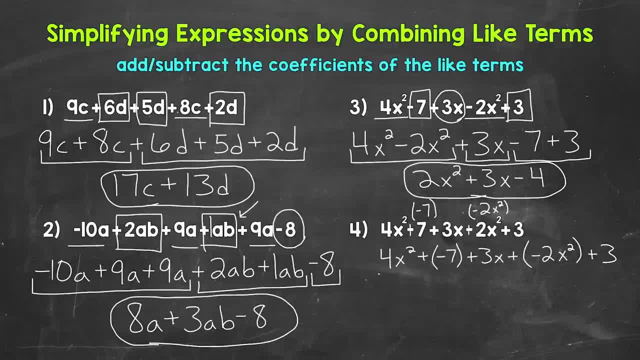 Now we can identify any like terms. We have 4x squared And negative 2x squared, Then we have negative 7 and 3 and then 3x. Now let's rewrite this expression with the like terms next to each other. 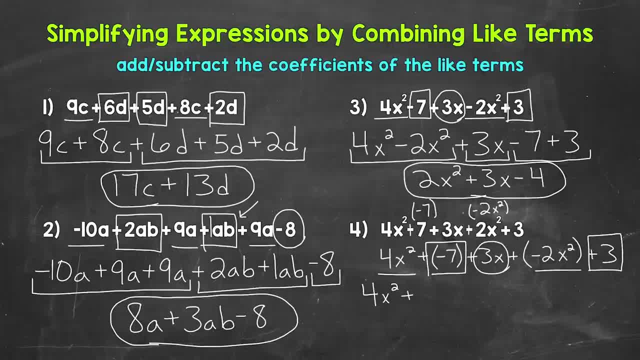 So we have 4x squared plus negative, 2x squared plus 3x plus negative: 7. Negative: 7 plus 3. Now we can combine like terms: We have 4x squared plus negative, 2x squared, 4 plus negative 2 is 2.. 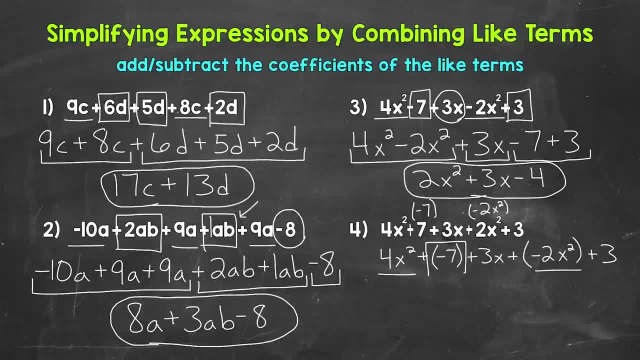 negative 2x squared, Then we have negative 2x squared and negative 2x squared, So we have negative 7 and 3 and then 3x. Now let's rewrite this expression with the like terms next to each other. So we have 4x squared plus negative 2x squared plus 3x, plus negative 7 plus 3.. Now we can. 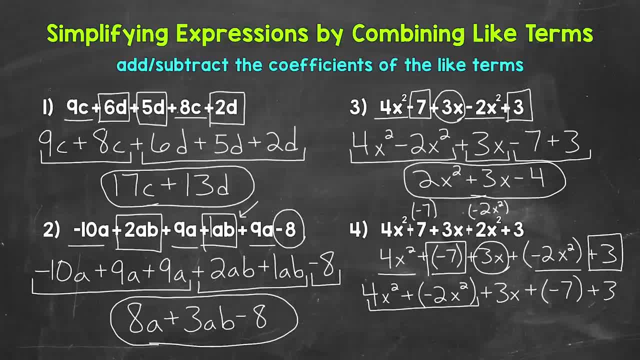 combine like terms. So we have 4x squared plus negative, 2x squared, 4 plus negative 2 is 2.. So we have 2x squared plus 3x, plus negative 7 plus 3.. Negative 7 plus 3 is negative 4.. So plus negative 4.. Now this is correct. but we can clean this up a little bit, so to speak. So we have 4x squared plus negative, 2x squared plus negative, 7 plus 3.. Negative: 7 plus negative: 2x squared plus 3. Place that in the middle of it. 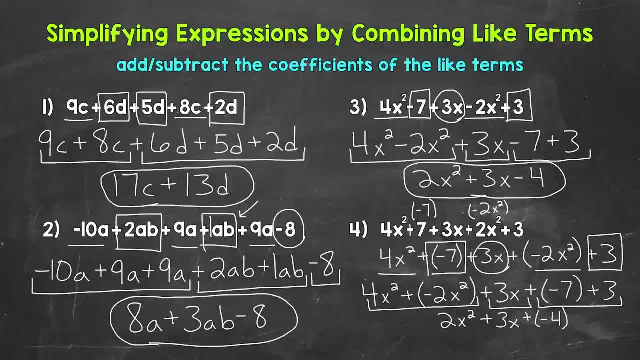 So now let's display 157, helping us obtain this paper formula that will give us the right answer. so we have. we have a double sign. we are adding a negative, adding a negative four. adding a negative four is the same as subtracting four. we are decreasing in value by four. so we can rewrite this with just one sign. we don't need. 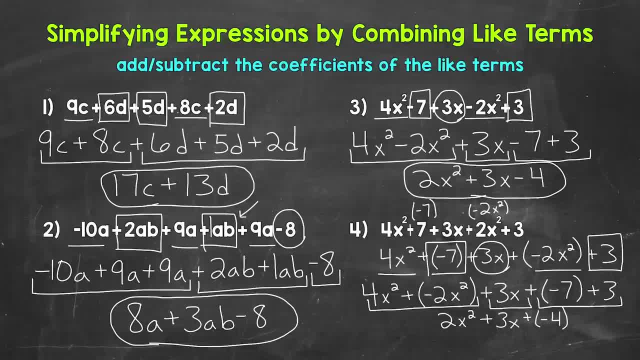 both of those signs. when we add a negative, that's the same as just subtracting a positive. so let's change this to subtracting 4.. And again, getting rid of the double sign will make this a little simpler. It will clean it up. We can rewrite this as: 2x squared plus 3x minus 4.. 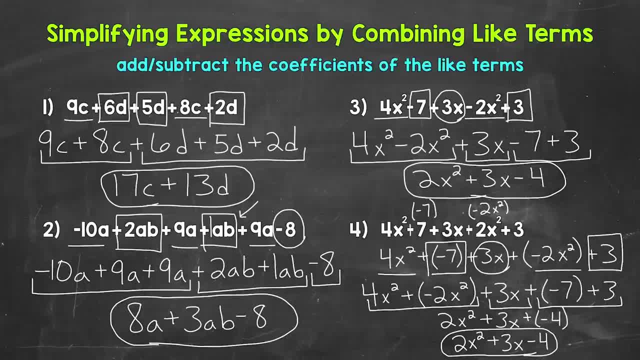 And that's our final simplified expression. So you can see that we got the same exact simplified expression for number 3 and 4.. Just slightly different strategies as far as organizing the expression. to start Now, I do want to mention one last thing, and it's about writing. 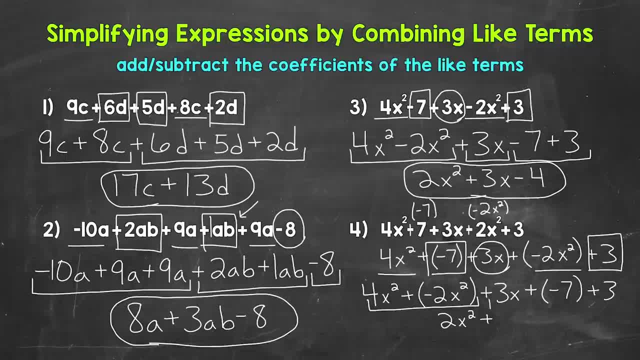 So we have 2x squared plus 3x, plus negative 7 plus 3.. Negative 7 plus 3 is negative 4. In this case we add a negative 4 to the negative to the positive, So we can find the original value of our total. 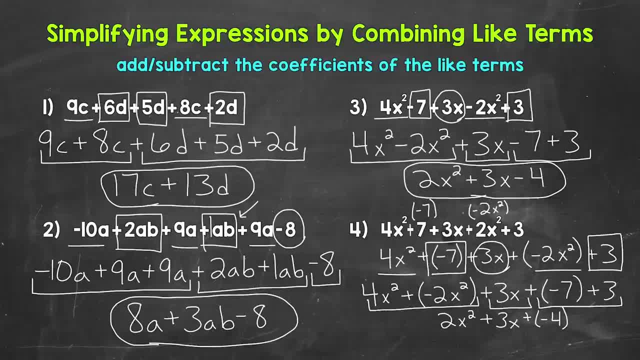 We add this in half, So what we get here is a plus and a minus in our sum. We do not subtract anything like negative, And so it turns out that we have one plus and a minus. That's the same as just subtracting a positive. 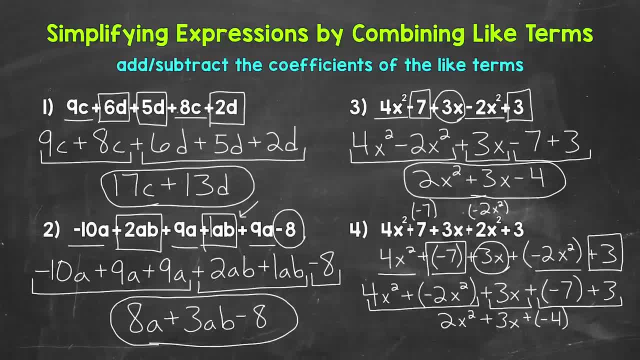 So let's change this to subtracting 4.. And again, getting rid of the double sign will make this a little simpler. It will clean it up. We can rewrite this as 2x squared plus 3x minus 4. And that's our final simplified expression. 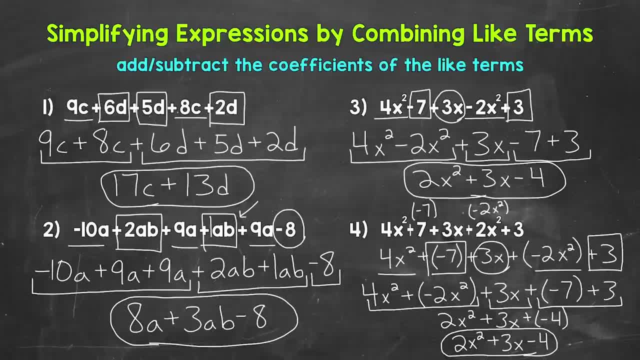 So you can see that we got the same exact simplified expression for number 3 and 4.. Just slightly different strategies as far as organizing the expression. to start Now, I do want to mention one last thing, and it's about writing out expressions. 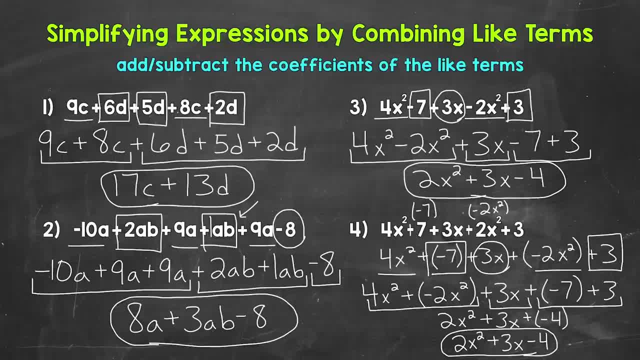 When we write an expression, we typically want any exponents first. If there are multiple exponents, write them from greatest to least. If we have the same exponent, go in ABC order and then constant terms always come last. So for example, in number 1, we have the variables of C and D. 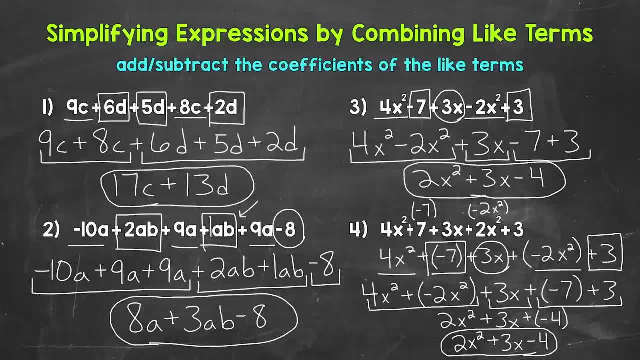 out expressions. When we write an expression, we typically want any exponents first. If there are multiple exponents, write them from greatest to least. If we have the same exponent, go in ABC order And then constant Terms always come last. So for example, in number 1, we have the variables of c and d. 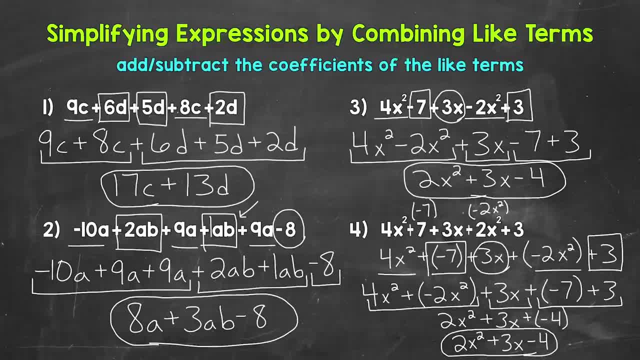 Both are to the understood power of 1.. So we go in ABC order. For number 2, we have a and ab. Everything here is to the understood power of 1.. So we go in ABC order: A comes first, then ab, and then the constant term comes last. For numbers 3 and 4, we have x squared. 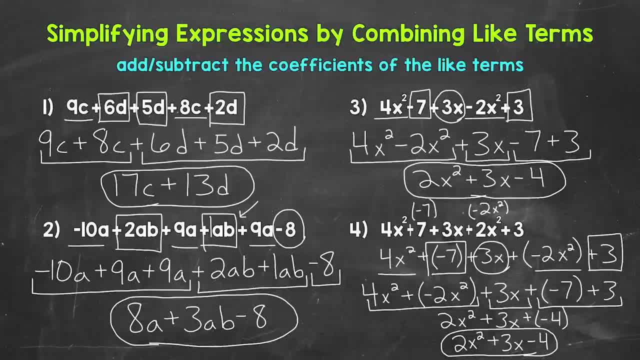 so the greatest exponent, 2.. Then we have the variable of x to the understood power of 1.. And then, lastly, we have the constant term. So something to keep in mind when you are writing expressions. So there's how to combine like terms. Let's move on to the distributive property. 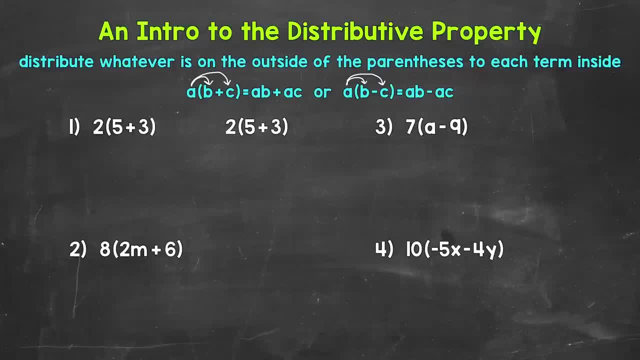 Here is an introduction to the distributive property. Now the distributive property can help us remove parentheses within algebraic expressions. This helps us simplify expressions when we do not have like terms within parentheses that we can combine. Now remember when we have something next to parentheses. 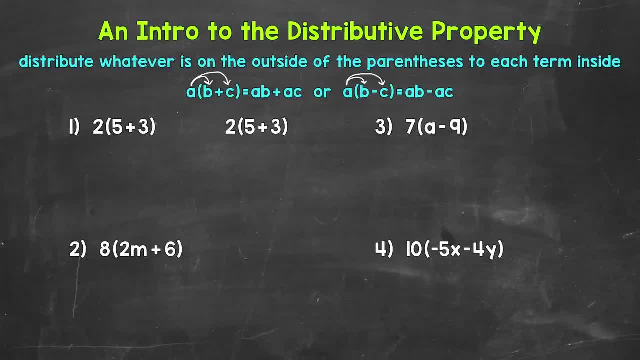 that means multiplication. So we can use the distributive property to distribute whatever is on the outside of the parentheses to the terms inside the parentheses. The distributive property works when we have addition or subtraction inside of the parentheses. So at the top of the screen there is a. 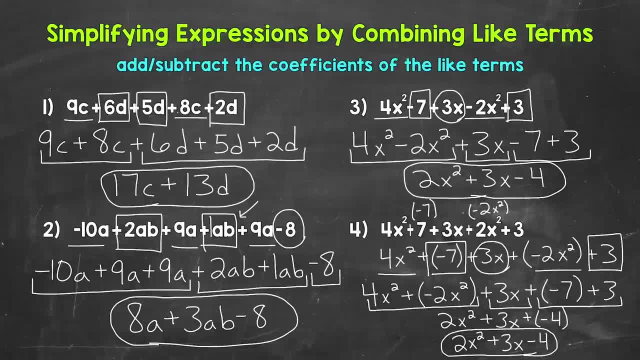 Both are to the understood power of 1.. So we go in ABC order. For number 2, we have A and AB. Everything here is to the understood power of 1.. So we go in ABC order: A comes first, then AB and then the constant term comes last. 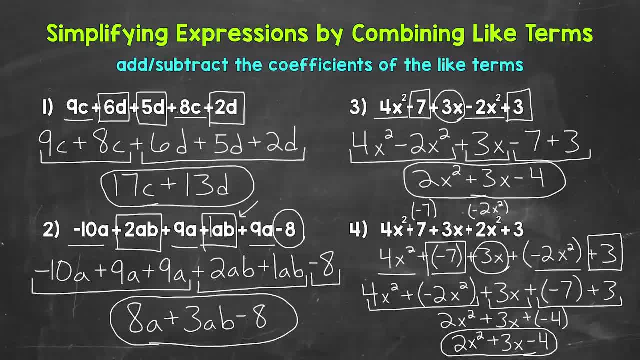 For numbers 3 and 4, we have x squared, so the greatest exponent, 2.. Then we have the variable of x to the understood power of 1.. And then, lastly, we have the constant term. So something to keep in mind when you are writing expressions. 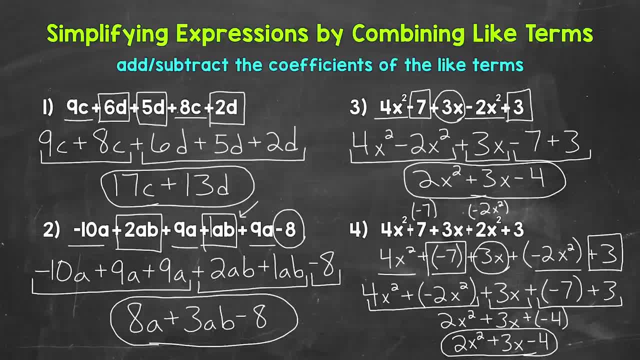 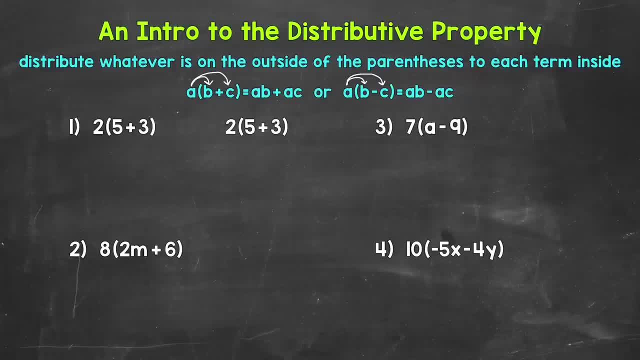 So there's how to combine like terms. Let's move on to the distributive property. Here is an introduction to the distributive property. Now, the distributive property can help us remove parentheses within algebraic expressions. This helps us simplify expressions when we do not have like terms within parentheses that we can combine. 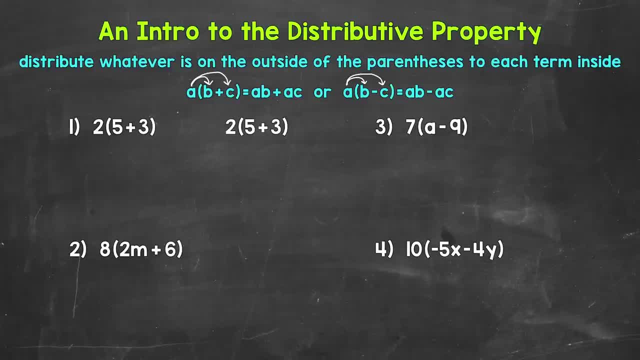 Now remember when we have something next to parentheses, that means multiplication, So we can use the distributive property to distribute whatever is on the outside of the parentheses to the terms inside the parentheses. The distributive property works when we have addition or subtraction. 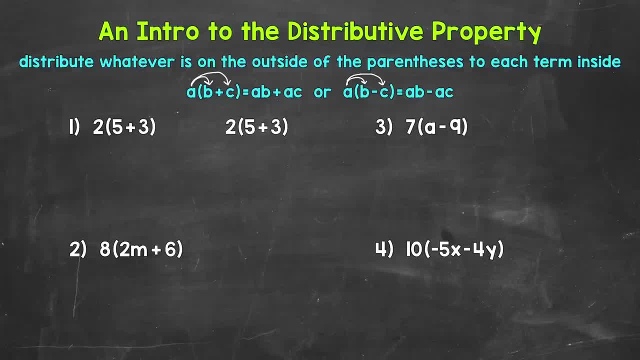 inside of the parentheses. So at the top of the screen there is a general overview of the distributive property where A is being distributed to the terms inside of the parentheses, The distributive property. and that overview will make a lot more sense as we go through our examples. 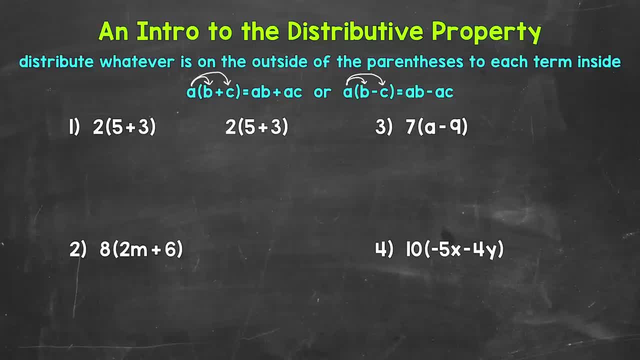 Let's jump into number 1, where we have 2 and then, in parentheses, 5 plus 3.. And we're going to do this two different ways: By using the order of operations, So doing what's in the parentheses first, and then also using the distributive property. 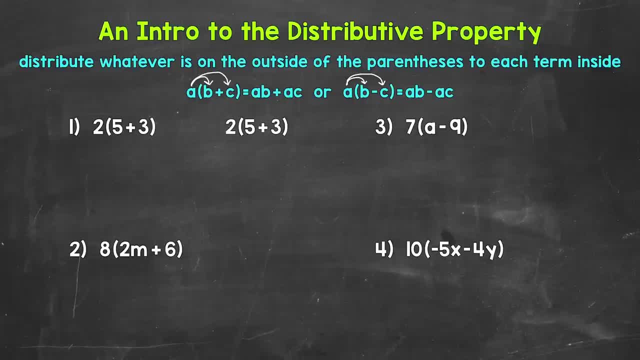 general overview of the distributive property where a is being distributed to the terms inside of the parentheses, The distributive property, and that overview will make a lot more sense as we go through our examples. Let's jump into number one, where we have two and then, in parentheses, five. 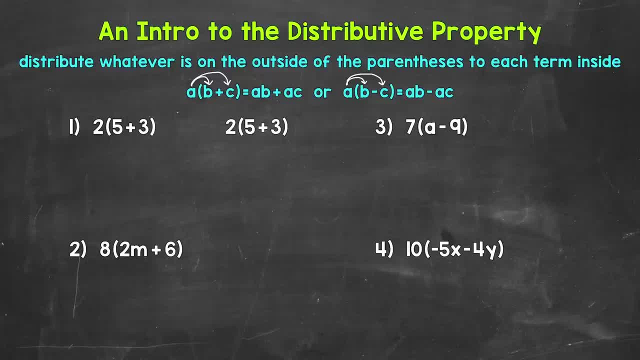 plus three. And we're going to do this two different ways: by using the order of operations, So doing what's in the parentheses first, and then also using the distributive property. Now for number one, we don't have any variables involved. We are actually able to add what's in the parentheses. 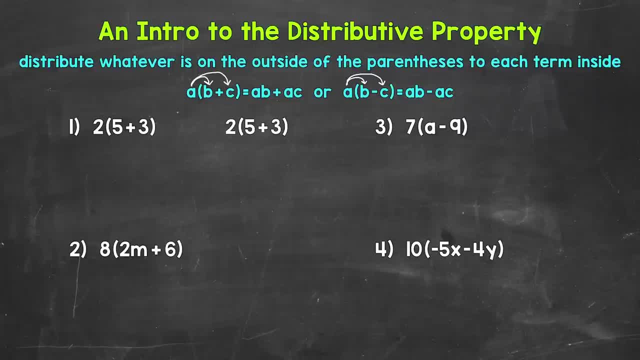 Now for number 1, we don't have any variables involved. We are actually able to add what's in the parentheses first and then go from there. We don't have to use the distributive property. But the point of number 1 is to show us that we get the same thing either way. 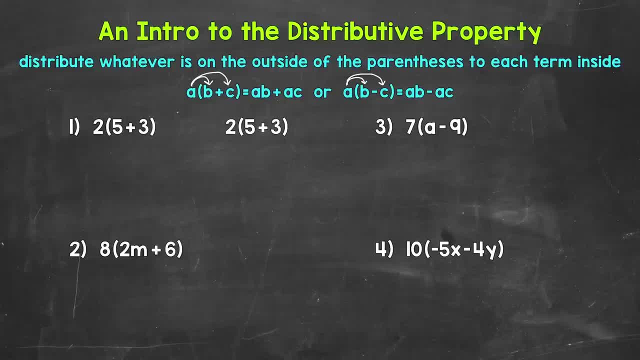 This is going to show us that the distributive property doesn't change the value of an expression. We are able to use this strategy, So again, we get the same thing. either way, Let's start by using the order of operations and doing what's in the parentheses first. 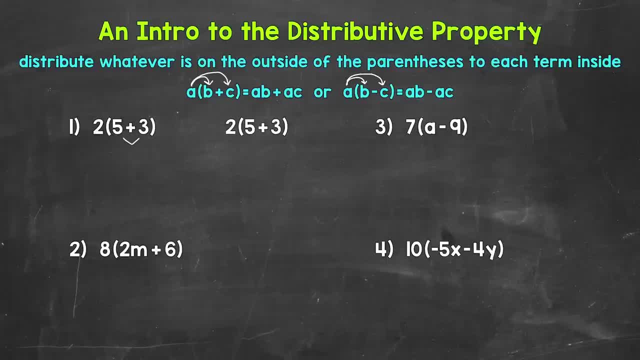 We have 5 plus 3, which is 8.. Bring down the 2. And now we have 2 times 8,, which is 16.. Now let's use the distributive property and see if we still get 16.. 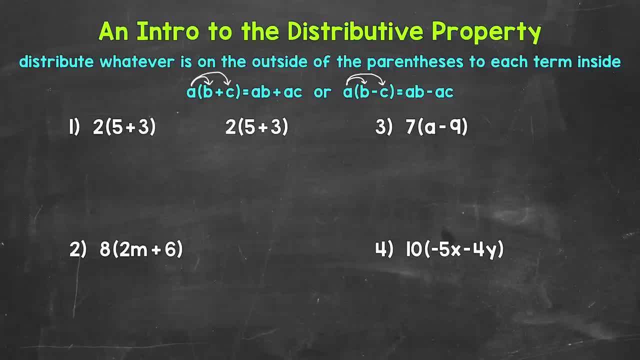 first and then go from there. We don't have to use the distributive property. but the point of number one is to show us that we get the same thing either way. This is going to show us that the distributive property doesn't change the value of an expression. We are able to use this. 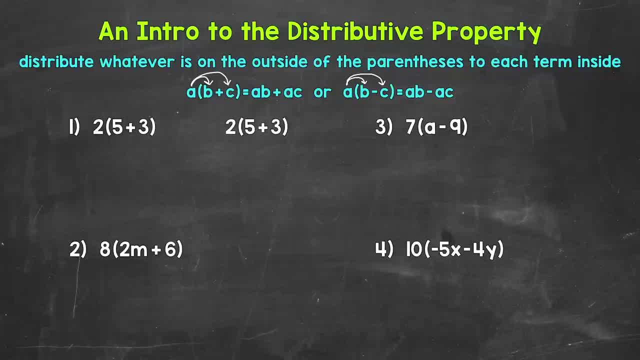 story. So again we get the same thing. either way, Let's start by using the order of operations and doing what's in the parentheses. first We have five plus three, which is eight. Bring down the two, and now we have two times eight, which is sixteen. Now let's use the distributive property and see. 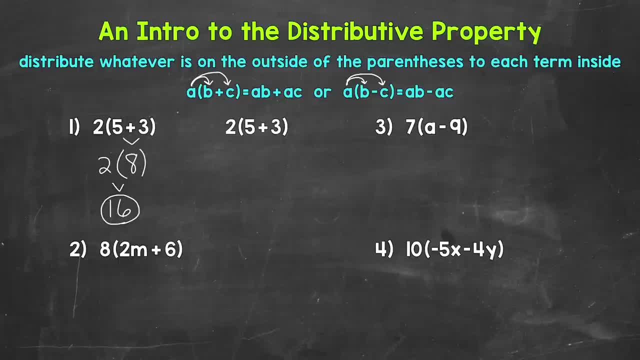 if we still get sixteen. So we need to take that two on the outside of the parentheses and we're going to do that by using the order of operations. So again, we get the same thing. either way, Let's start by using the order of operations and doing what's in the parentheses. first We are able to use the. 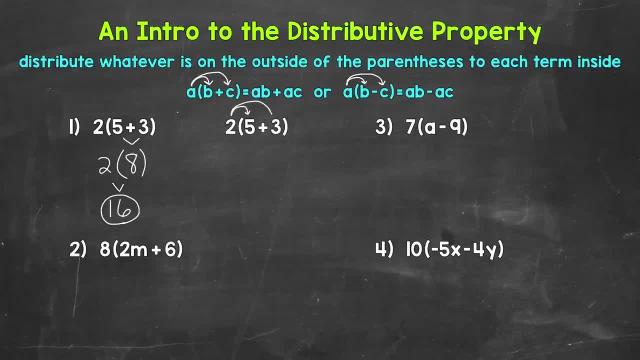 and distribute it to the five and to the three. So we have two times five plus two times three. Two times five gives us ten, plus two times three gives us six. Ten plus six is sixteen. So we get sixteen that way as well. 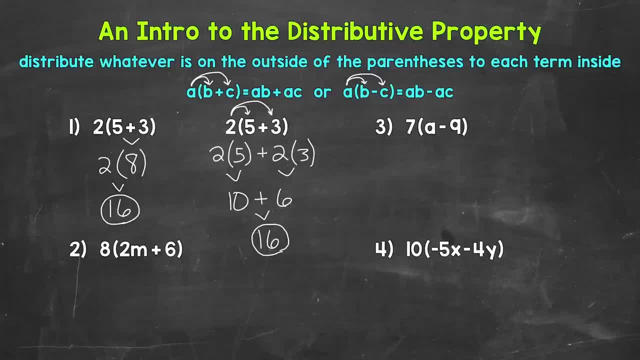 So we can see that the distributive property doesn't change the value of an expression and we are able to use it. Let's move on to number two, where we will apply this to an algebraic expression. in order to simplify the expression, We are going to remove the parentheses For number 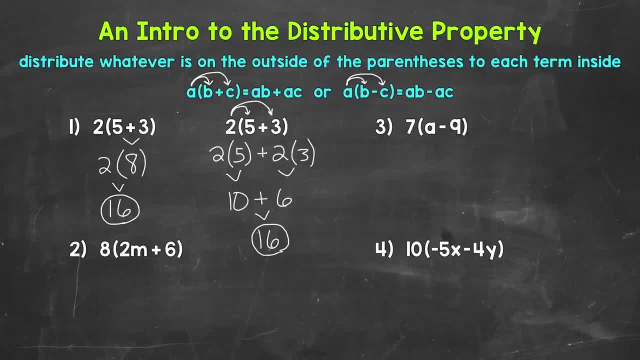 two, we have eight, and then in parentheses, two m plus six. Now we can't combine those terms in parentheses. So what we can do, we can use the distributive property to remove those parentheses and simplify this expression. So let's distribute the eight to the two m and to the six, This gives us eight times two m plus eight. 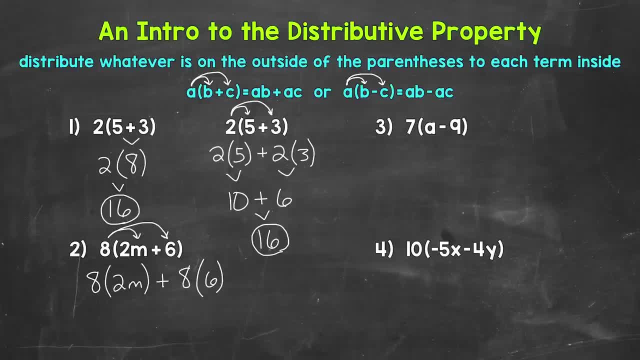 times six, Eight times two, m is sixteen m plus eight times six is forty eight. Now, sixteen m and forty-eight are unlike terms, So we don't have any terms that we can combine. So we are done here. Sixteen m plus forty-eight is our. 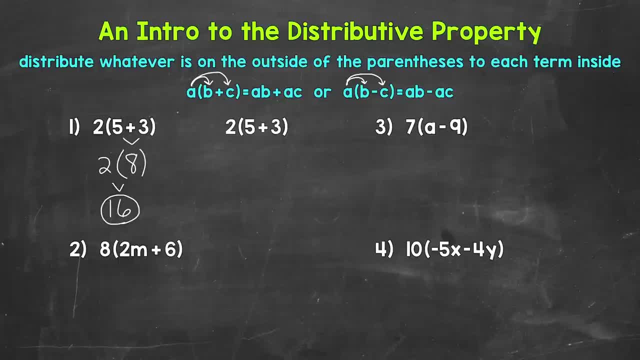 So we need to take that 2. On the outside of the parentheses, And distribute it to the 5 and to the 3. So we have 2 times 5 plus 2 times 3.. 2 times 5 gives us 10.. 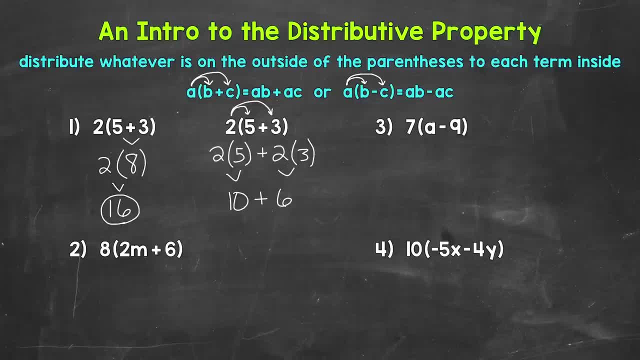 Plus 2 times 3 gives us 6.. 10 plus 6 is 16.. So we get 16 that way as well. So we can see that the distributive property doesn't change the value of an expression And we are able to use it. 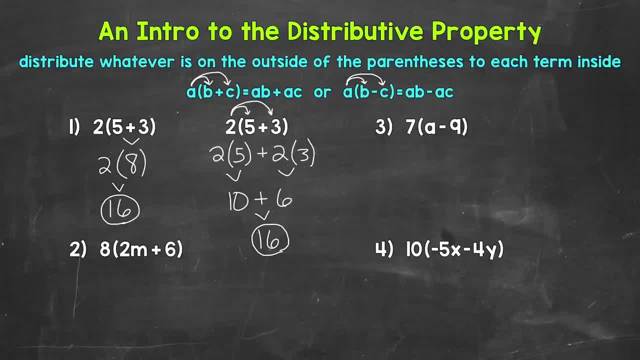 Let's move on to number 2, where we will apply this to an algebraic expression. In order to simplify the expression, we are going to remove the parentheses. For number 2, we have 8.. And then, in parentheses, 2m plus 6.. 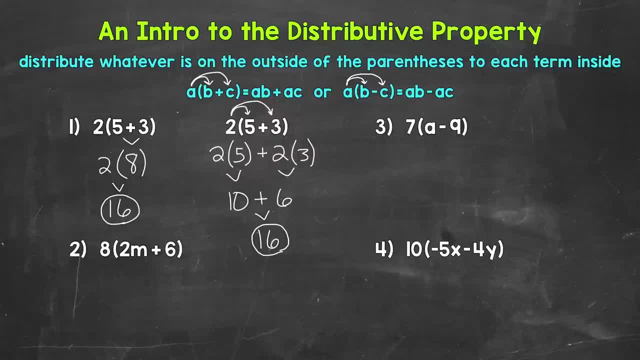 Now we can't combine those terms in the parentheses. So what we can do, we can use the distributive property to remove those parentheses and simplify this expression. So let's distribute the 8 to the 2m and to the 6.. 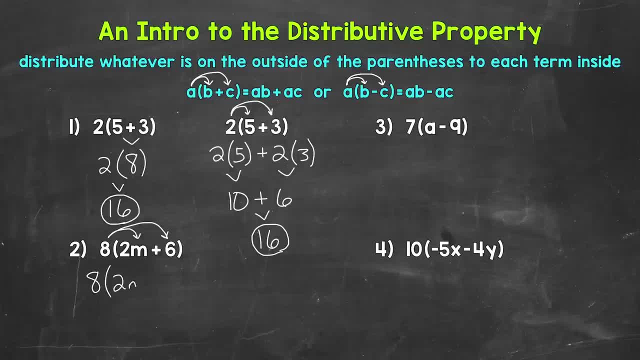 This gives us 8 times 2m plus 8 times 6.. 8 times 2m is 16m. Plus 8 times 6 is 48. Now 16m and 48 are unlike terms, So we don't have any terms that we can combine. 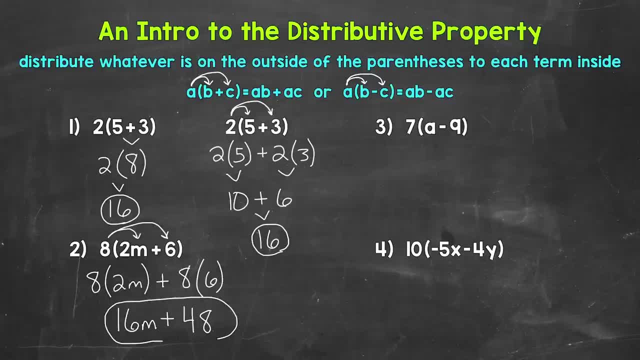 So we are done here. 16m plus 48 is our simplified expression. Let's move on to number 3, where we have 7. And then, in parentheses, a minus 9.. Let's distribute that 7 to the a and to the 9.. 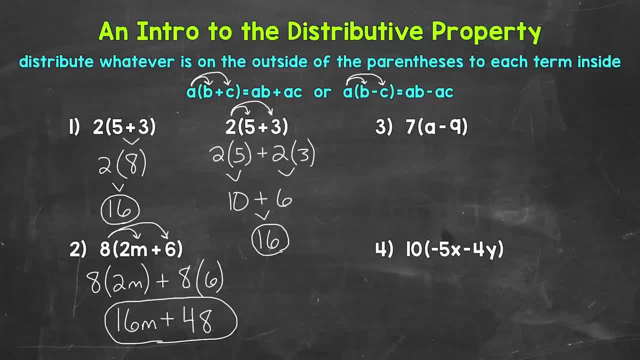 simplified expression. Let's move on to number three, where we have seven and then, in parentheses, a minus nine. Let's distribute that seven to the a and to the nine. That gives us seven times a minus. bring the subtraction sign down seven times nine. seven times a is just seven. 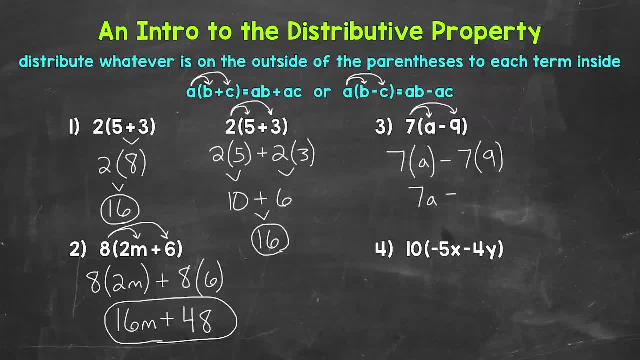 a minus seven times nine is 63. so we end up with 7a minus 63. we don't have any like terms that we can combine, so we are simplified and done again: 7a minus 63.. now i do want to mention another way. 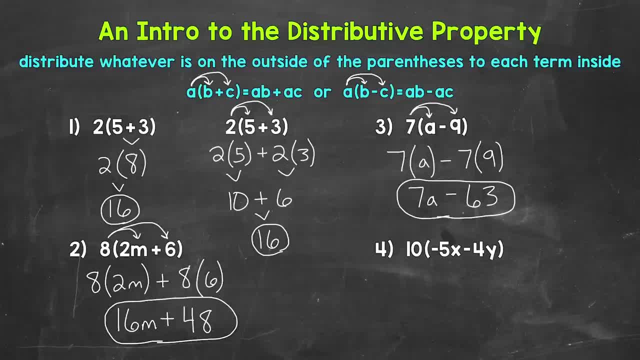 to think through this and this is another way to think through whenever subtraction or negatives are involved. so let me rewrite the expression and then distribute the 7.. so we have 7 times a, which is 7a, and then we can think of that subtraction sign and the 9 as a negative 9, so including the sign. 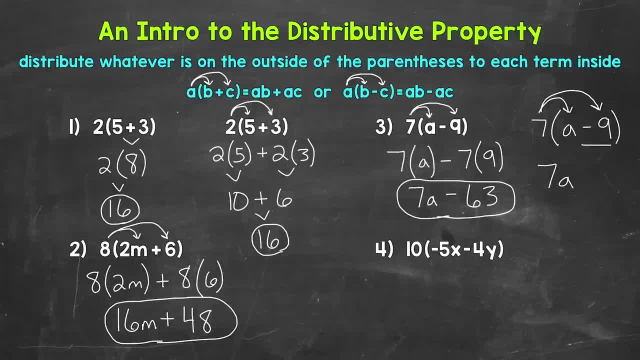 in front with the 9, so we think of that as a negative 9.. so let's distribute that 7 to the negative 9.. 7 times negative 9 is negative 63, so negative 63, and we get 7a minus 63. 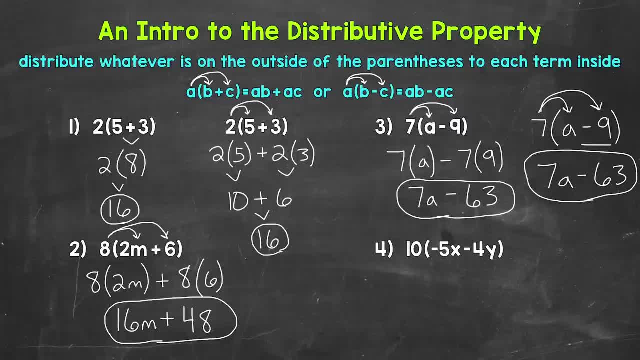 and again. that's just a different way to think through it. you get the same thing either way, but you can include the sign in front of the term and think of that as a negative 9.. so something to keep in mind. let's move on to number four, where we have 10, and then in 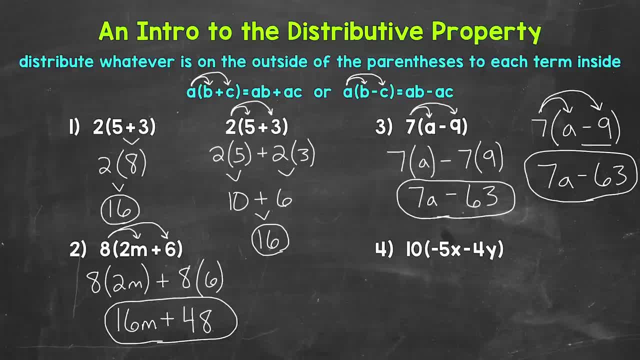 parentheses: negative 5x minus 4y. let's distribute the 10 to the negative 5x and to the 4y, so 10 times negative 5x minus 10 times 4 y. 10 times negative 5x gives us negative 50 x minus 10 times. 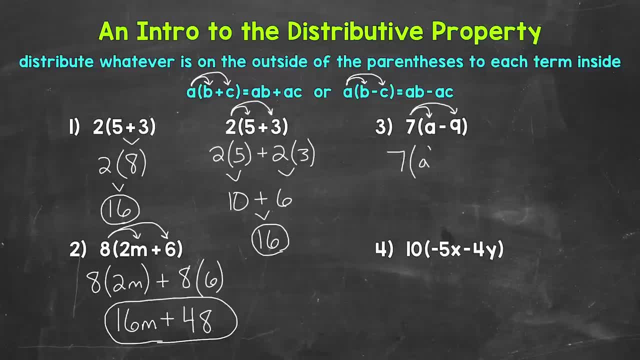 That gives us 7 times a minus. bring the subtraction sign down 7 times 9.. 7 times a is just 7a. minus 7 times 9 is 63. So we end up with 7a minus 63.. 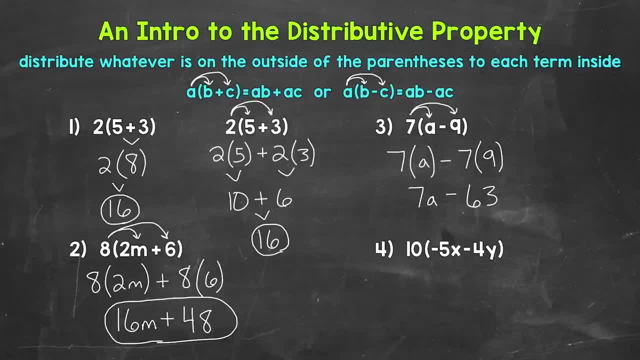 We don't have any like terms that we can combine, So we are simplified and done Again: 7a minus 63.. Now I do want to mention another way to think through this, And this is another way to think through whenever subtraction or negatives are involved. 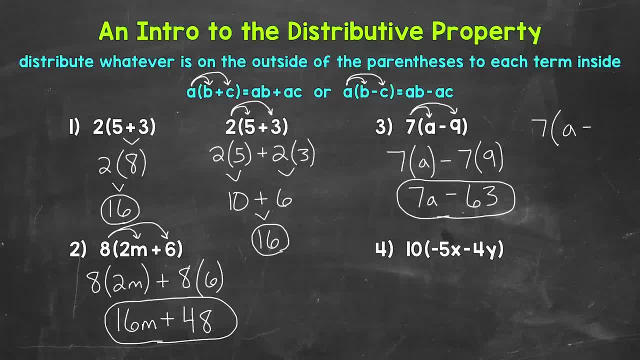 So let me rewrite the expression And then distribute the 7.. So we have 7 times a, which is 7a, And then we can think of that subtraction sign and the 9 as a negative 9.. So including the sign in front with the 9.. 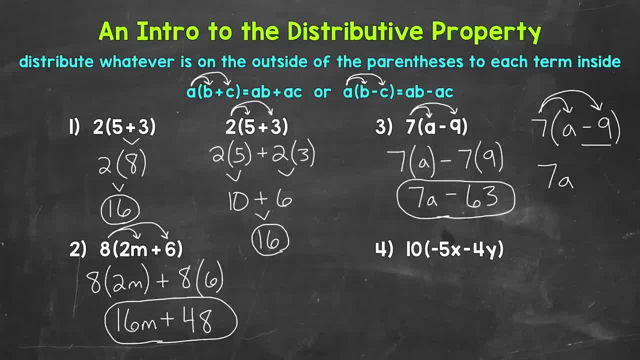 So we think of that as a negative 9.. So let's distribute that 7 to the negative 9.. 7 times negative 9 is negative 63. So negative 63. And we get 7a minus 63 that way as well. 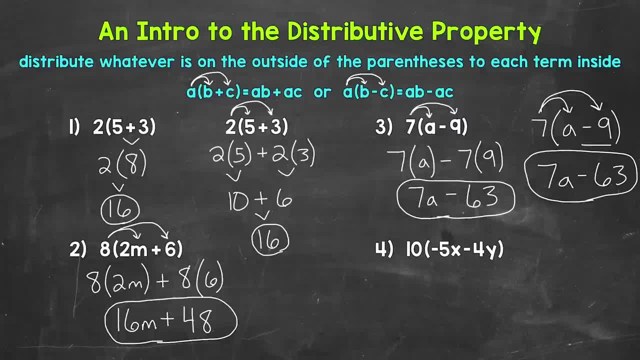 And again, that's just a different way to think through it. You get the same thing either way, But you can include the sign in front of the term and think of that as a negative 9.. So something to keep in mind. Let's move on to number 4, where we have 10 and then, in parentheses, negative 5x minus 4y. 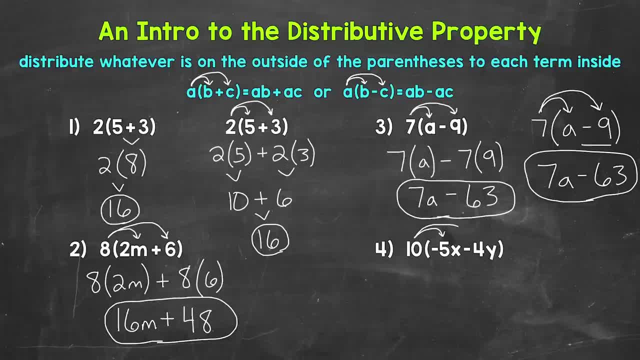 Let's distribute the 10 to the negative 5x And to the 4y. So 10 times negative 5x minus 10 times 4y. 10 times negative 5x gives us negative 50x. Minus 10 times 4y gives us 40y. 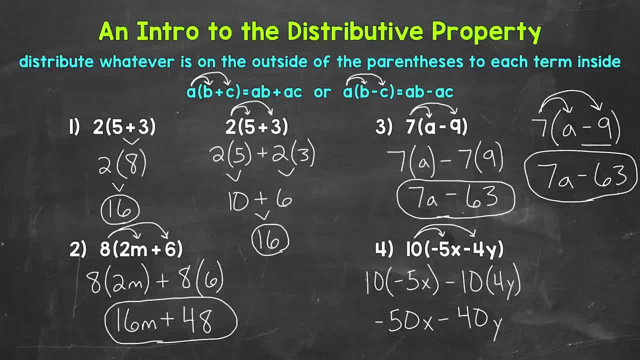 So we end up with Negative 50x minus 40y. We don't have any like terms that we can combine. So we are done Again: negative 50x minus 40y. Now let's take a look at a different way to think through this. 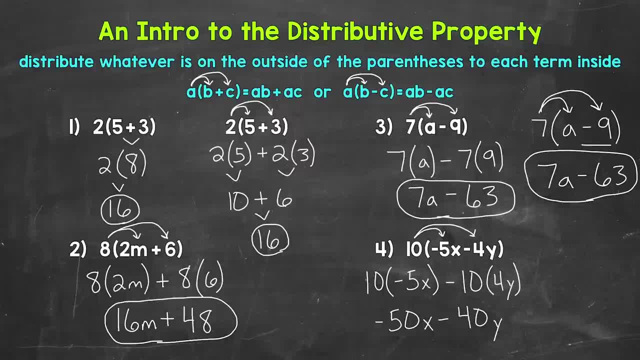 4y gives us 40 y, so we end up with negative 50 x minus 40 y. we don't have any like terms that we can combine, so we are done again: negative 50 x minus 40 y. now let's take a look at a different way to. 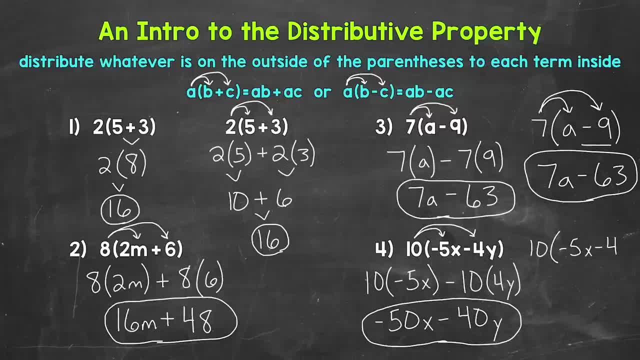 think through this, so i will rewrite the expression off to the side. so let's distribute the 10 to the negative 5x and then we will think of that as negative 4y, so include the sign in front of that term. 10 times negative 5x is negative 50x, And then 10 times negative 4y is negative 40y. So we 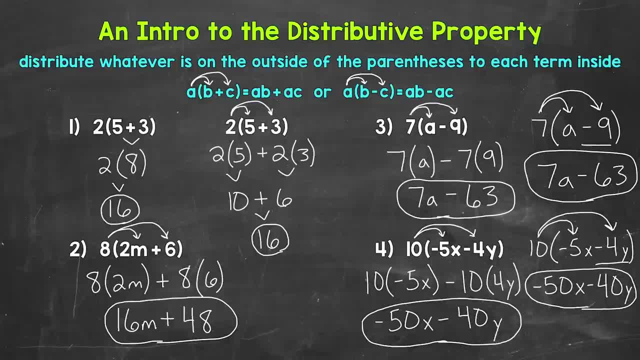 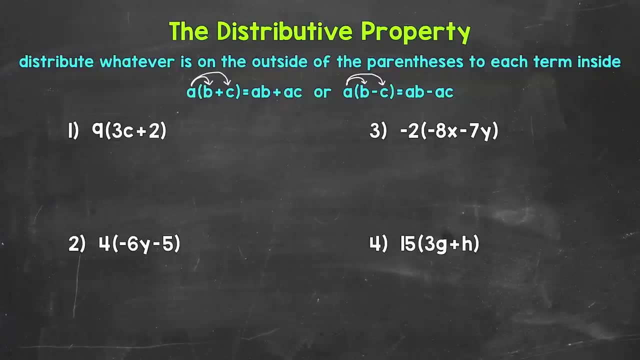 get the same thing that way as well. Negative 50x minus 40y. So there is an introduction to the distributive property. Let's take a look at four more examples. Here are more examples that we can go through to get the distributive property down. Let's jump into number one, where we have 9. 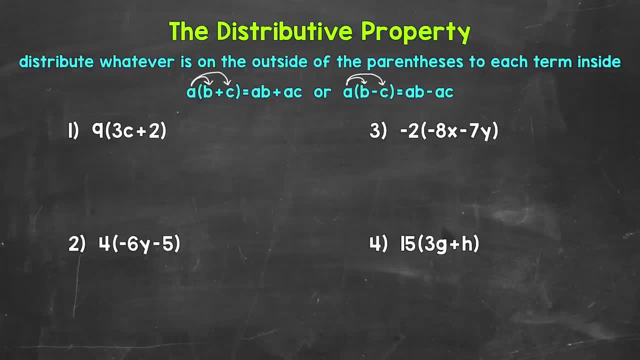 and then 3c plus 2 in the parentheses. Let's distribute that 9 to the 3c and to the 2.. So we have 9 times 3c, which is 27c plus. so we bring that addition sign down and then we have 9 times. 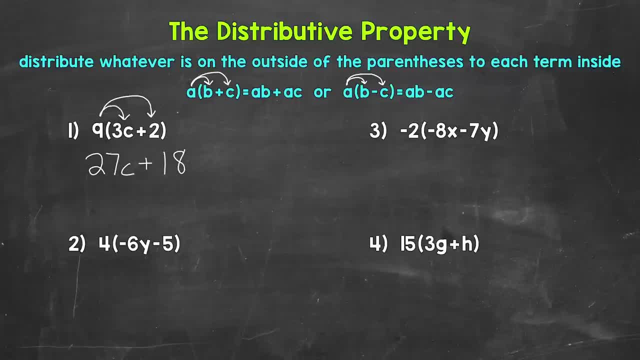 2,, which is 18.. So we end up with 27c plus 18.. Now we don't have any like terms that we can combine, So this has been simplified. We can't simplify any further. So again, 27c plus 18.. Let's move on to number two. 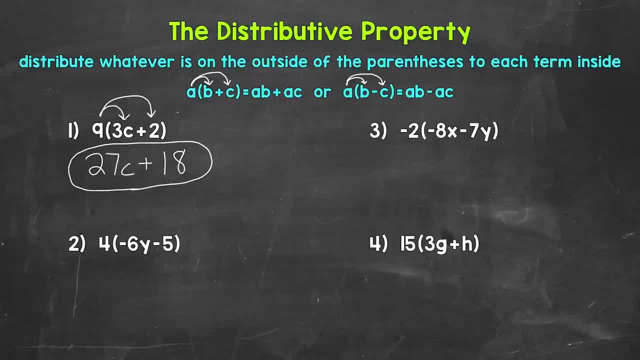 where we have 4 and then, in parentheses, negative 6y minus 5.. Let's distribute that 4 to the negative 6y plus negative 6y plus negative 24y. Bring the subtraction sign down and then we have 4 times 5,. 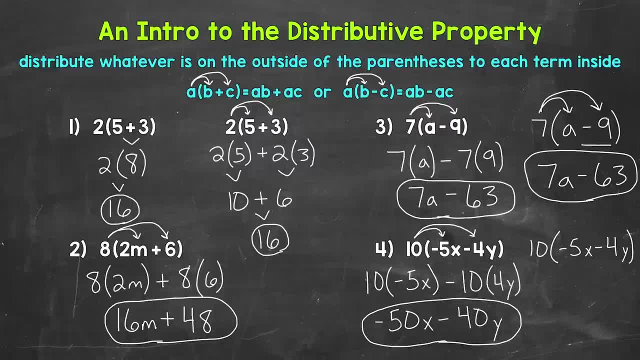 So I will rewrite the expression off to the side. So let's distribute the 10 to the negative 5x And then we will think of that as negative 4y, So include the sign in front of that term. 10 times negative 5x is negative 50x. 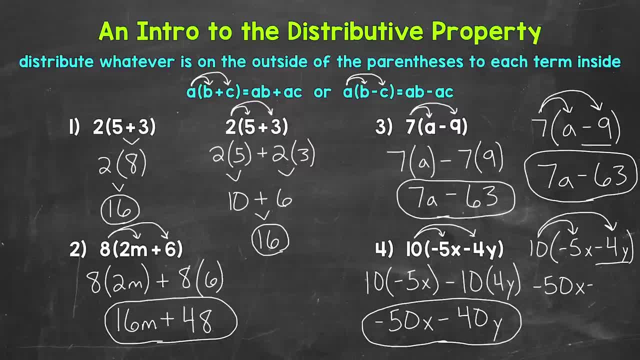 And then 10 times negative 4y is negative 40y. So we get the same thing that way as well. Negative 50x minus 40y. So there is an introduction to the distributive property. Let's take a look at four more examples. 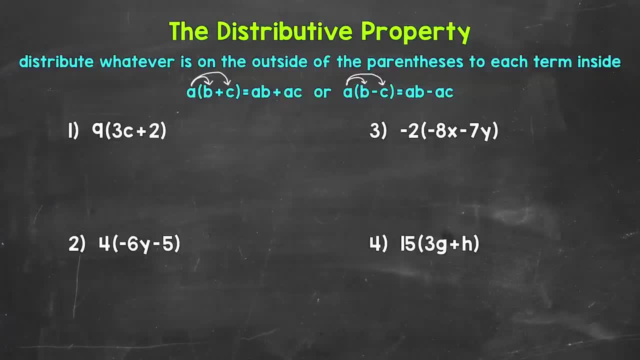 Here are more examples that we can go through to get the distributive property down. Let's jump into number 1, where we have 9 and then 3c plus 2 in the parentheses. Let's distribute that 9 to the 3c. 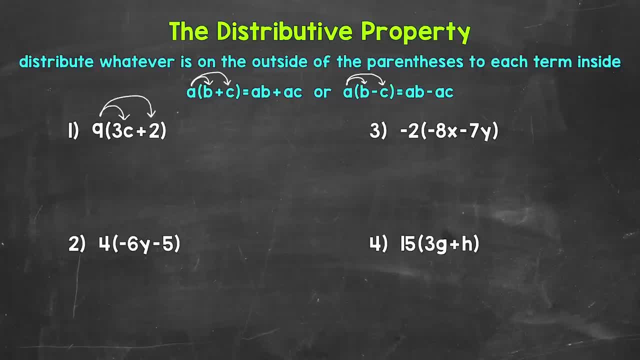 And to the 2.. So we have 9 times 3c, Which is 26.. Which is 27c Plus. So we bring that addition sign down And then we have 9 times 2., Which is 18.. 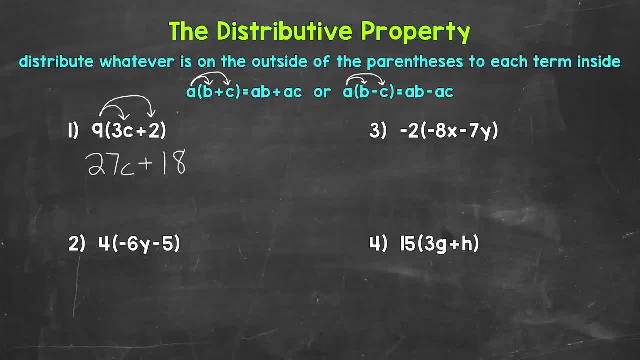 So we end up with 27c plus 18.. Now we don't have any like terms that we can combine, So this has been simplified. We can't simplify any further. So again: 27c plus 18.. Let's move on to number 2, where we have 4.. 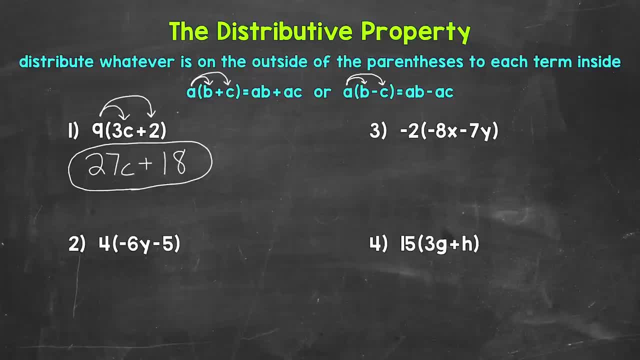 And then in parentheses: Negative 6y minus 5.. Let's distribute that 4 to the negative 6y And to the 5.. So 4 times negative 6y Is negative 24y. Bring the subtraction sign down. 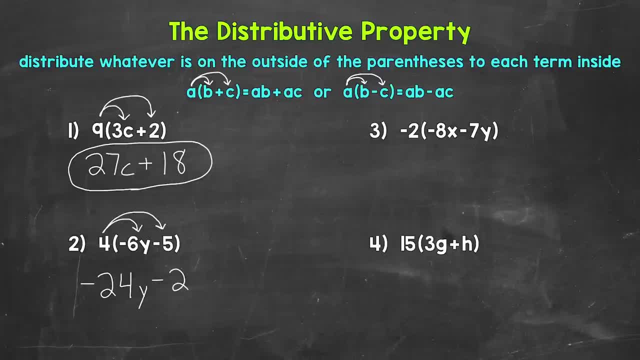 And then we have 4 times 5., Which is 20.. So we end up with negative 24y minus 20.. We don't have any like terms that we can combine, So this is simplified Again: negative 24y minus 20.. 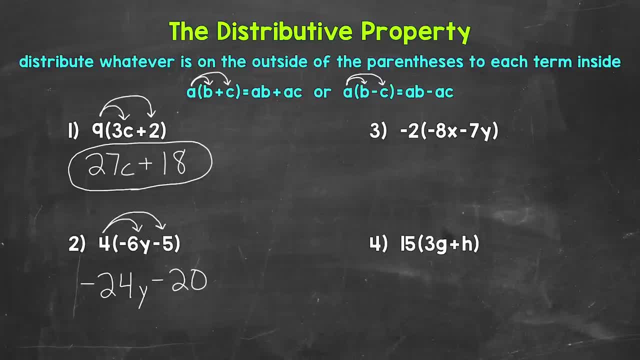 which is 20.. So we end up with negative 24y minus 20.. We don't have any like terms that we can combine, So this is simplified Again: negative 24y minus 20.. Now I do want to mention another. 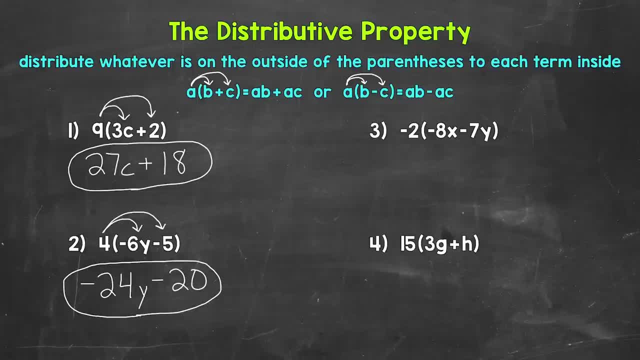 way to think through number two. It's going to be a little bit more complicated, but I'm going to- And this is an option when we have subtraction. So let me rewrite the expression here- And then we need to distribute the 4.. So distribute to the negative 6y. 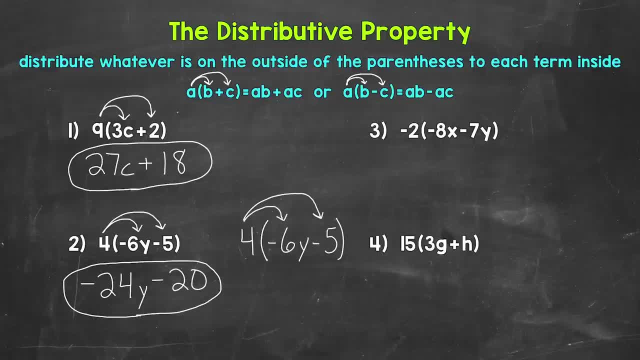 And then when we distribute to the 5,, we are going to look at this as negative 5.. So we are including that subtraction sign, the sign in front of the 5, and look at this as negative 5.. This gives us, well, 4 times negative 6y is negative 24y, And then 4 times negative 5 is. 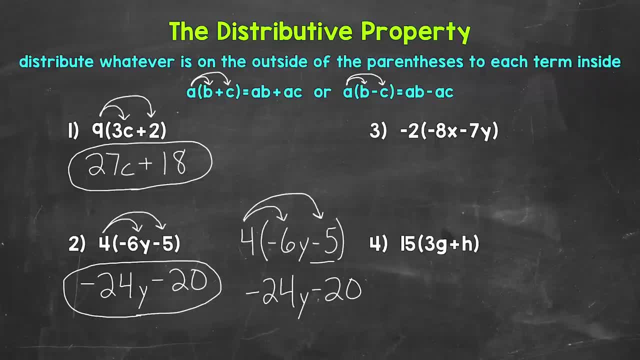 negative 20.. So we get negative 24y minus 20 that way as well. So we get the same thing either way, just slightly different. as far as working through the distributive property. Let's move on to number three, where we have negative 2 and then in parentheses, 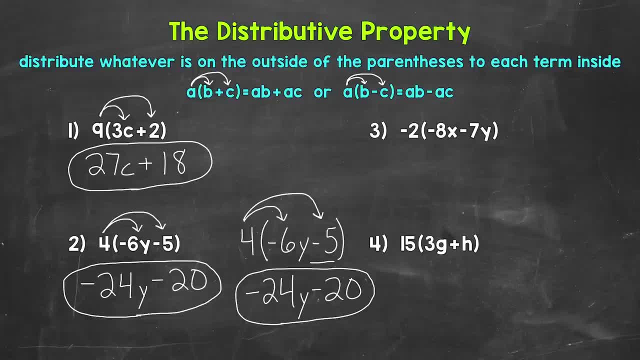 negative 8x minus 7y. Let's distribute the negative 2 to the negative 8x and to 7y. So negative 2 times negative 8x gives us 16x. Remember a negative times a negative is a positive, So 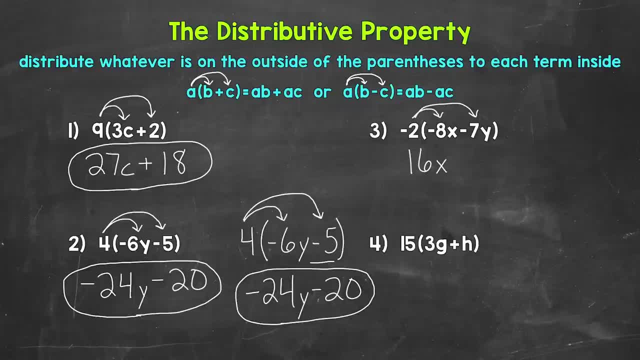 negative 2 times negative, 8 is a positive 16. And then we have that x, Then we can bring down the subtraction sign. And then we have negative 2 times negative, 8 is a positive 16. And then we can bring. 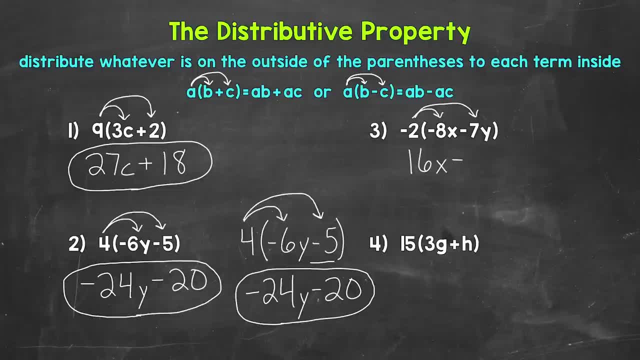 2 times 7y, That gives us negative 14y. Now this is correct, but we can clean this up a little bit. so to speak, We have a double sign, the subtraction, and then the negative. We don't need both of those signs. 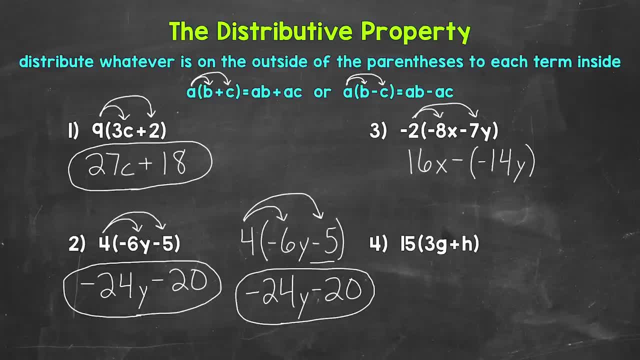 We can rewrite it with just 1. Think about working with negatives. When we subtract a negative, that's the same as adding a positive. We can change this to addition and that will make this simpler And, like I said, clean it up a little bit. 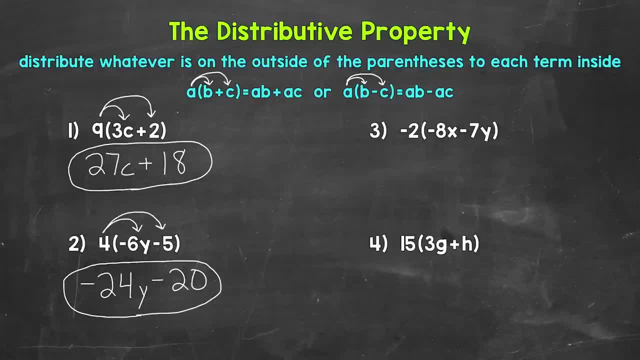 Now I do want to mention another way to think through number 2. And this is an option when we have subtraction, So let me rewrite the expression here. And then we need to distribute the 4. So distribute to the negative 6y. 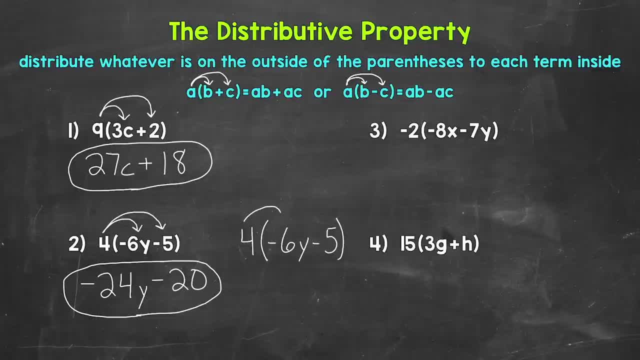 And then when we distribute to the 4., We have negative 6y, Which is minus 5.. And to the negative 6y, And then when we distribute to the 5, we are going to look at this as negative 5.. 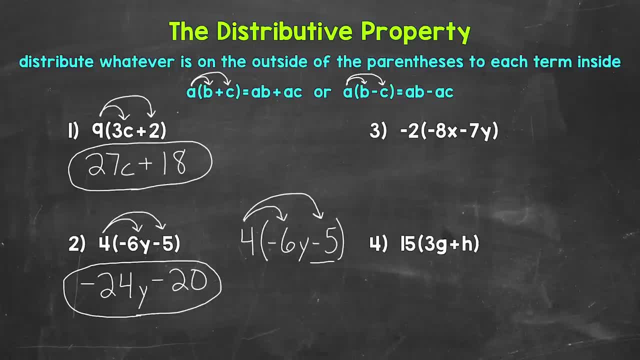 So we are including that subtraction sign, the sign in front of the 5, and look at this as negative 5.. This gives us: well, 4 times negative 6y is negative 24y, And then 4 times negative 5 is negative 20.. 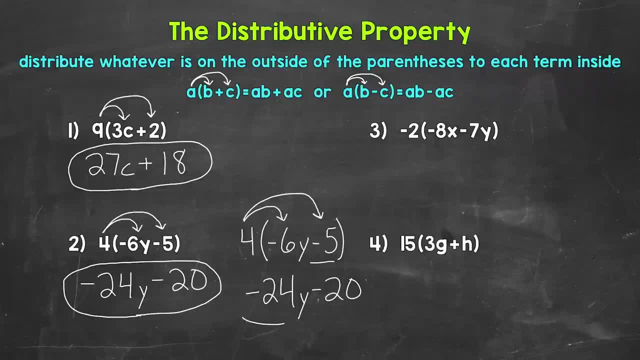 So we get negative 24y minus 20.. That way as well. So we get the same thing either way, just slightly different. as far as working through the distributive property. Let's move on to number 3, where we have negative 2 and then, in parentheses, negative 8x minus 7y. 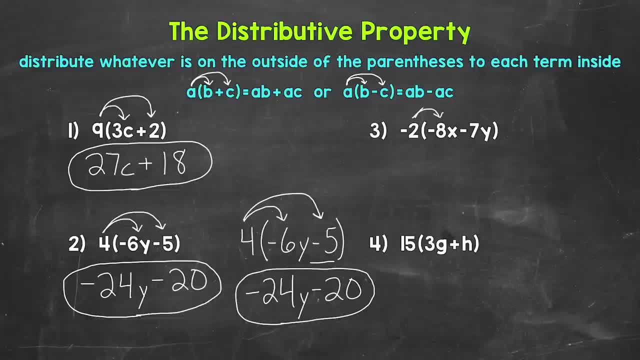 Let's distribute the negative 2 to the negative, 8x and to 7y. So negative 2 times negative, 8x gives us 16x. Remember. Remember a negative times a negative is a positive. So negative 2 times negative, 8 is a positive 16.. 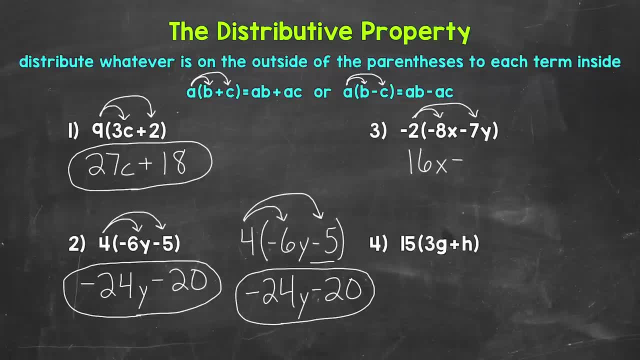 And then we have that x, Then we can bring down the subtraction sign And then we have negative 2 times 7y. That gives us negative 14y. Now this is correct, but we can clean this up a little bit, so to speak. 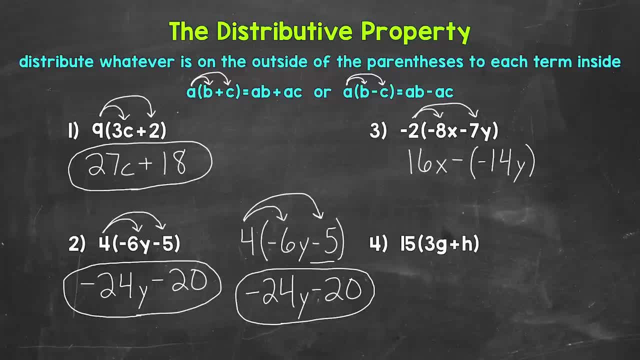 We have a double sign- The subtraction, and then the negative. We don't need both of those signs. We can rewrite it with just 1.. Think about working with negatives. When we subtract a negative, that's the same as adding a positive. 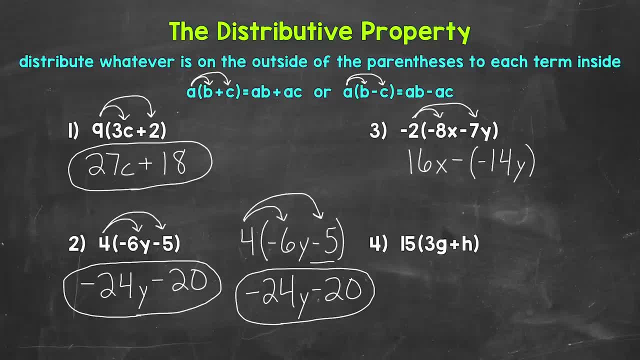 We can change this to addition and that will make this simpler And, like I said, clean it up a little bit. We can rewrite this as 16x plus 14y. We don't have any like terms that we can combine, So we are simplified again: 16x plus 14y. 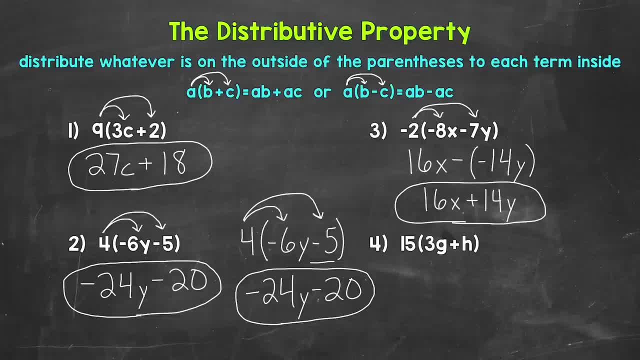 Just like number 2, I'll go through this a slightly different way. as far as thinking through the distributive property when it comes to subtraction, I will rewrite the expression off to the side here, And then we can distribute that negative 2 to the negative 8x. 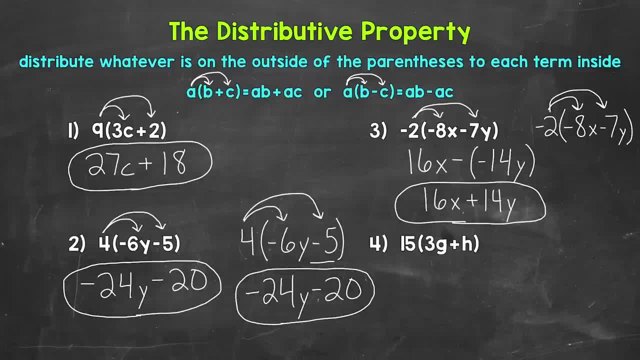 And then we can distribute that negative 2 to the negative 8x, And then we can distribute that negative 2 to the negative 7y. So we are including that sign in front of the term. Negative 2 times negative 8x gives us 16x. 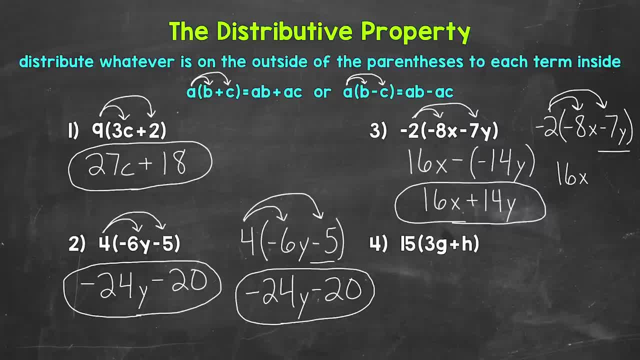 And then negative. 2 times negative. 7y gives us a positive 14y. So plus 14y. So we get the same thing. So we get the same thing there as well. Lastly, let's move on to number 4, where we have 15, and then 3g plus h in the parentheses. 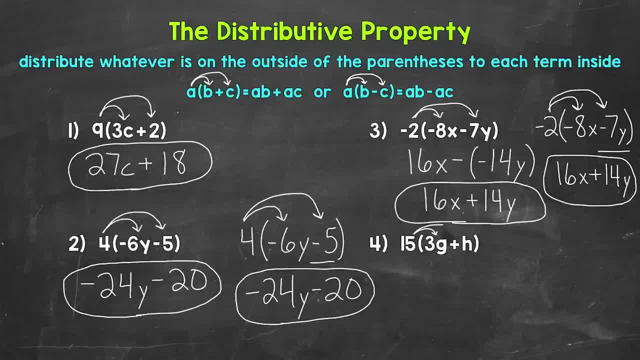 So let's distribute that 15 to the 3g and to the h. So we have 15 times 3g, That gives us 45g Plus, and then 15 times h. Well, that's just 15h. 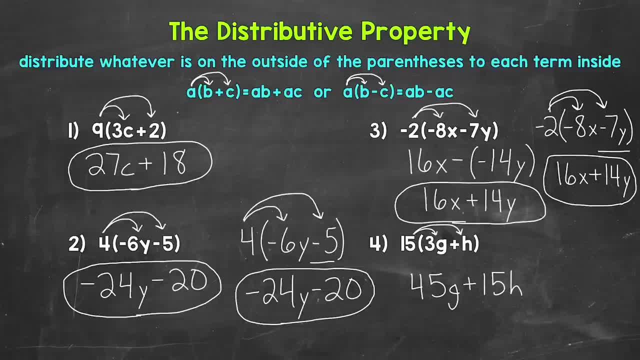 So we end up with 45g. So we end up with 45g plus 15h. We don't have any like terms that we can combine, So we can't simplify this any further. This is simplified, So, again, 45g plus 15h. 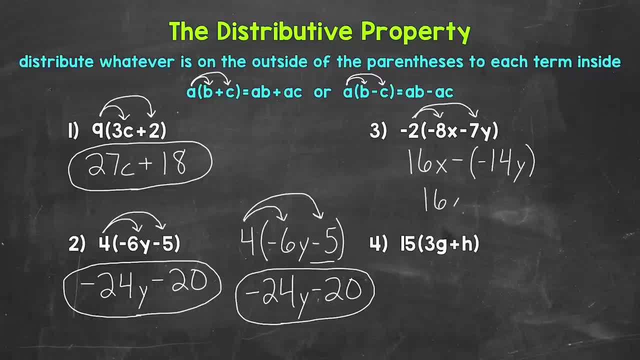 We can rewrite this as 16x plus 14y. We don't have any like terms that we can combine, So we are simplified again: 16x plus 14y. Just look Like number 2,. I'll go through this a slightly different way as far as thinking through the. 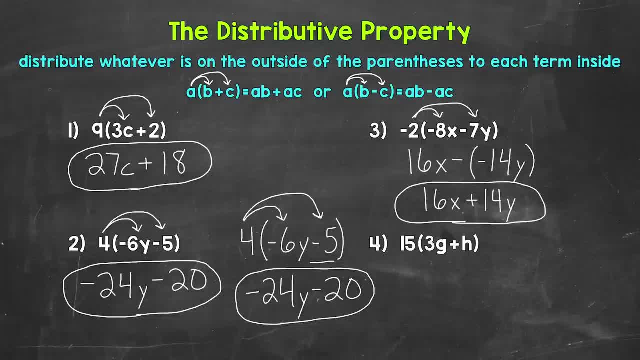 distributive property. when it comes to subtraction, I will rewrite the expression off to the side here: And then we can distribute that negative 2 to the negative 8x. And then we can distribute that negative 2 to the negative 7y. 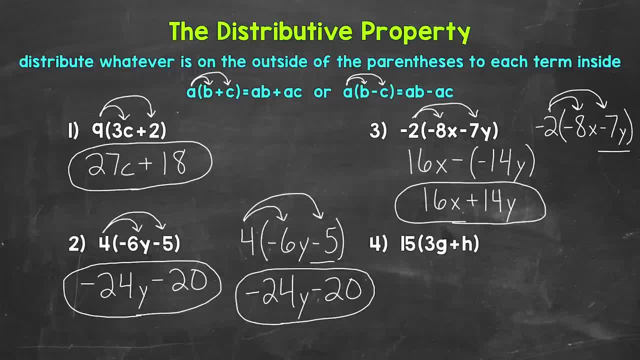 So we are including that sign. And then there is our derivative of the term Negative: 2 times negative- 8x- gives us 16x. And then negative 2 times negative- 7y- gives us a positive 14y. So plus 14y. 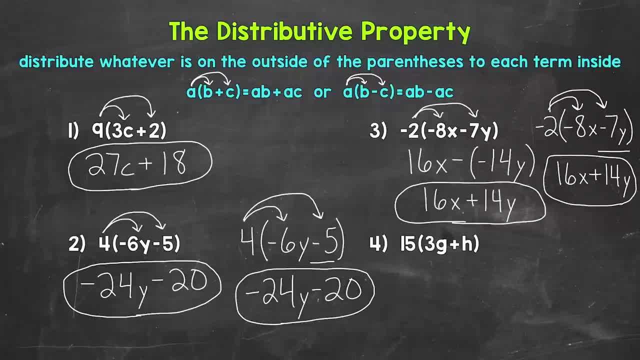 So we get the same thing there as well. Lastly, let's move on to number 4, where we have 15 and then 3g plus h in the parentheses. So let's distribute that 15 to the 3G and to the H. 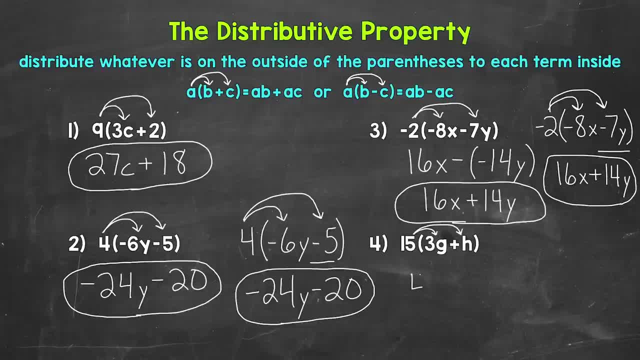 So we have 15 times 3G, That gives us 45G plus, and then 15 times H- Well, that's just 15H. So we end up with 45G plus 15H. We don't have any like terms that we can combine. 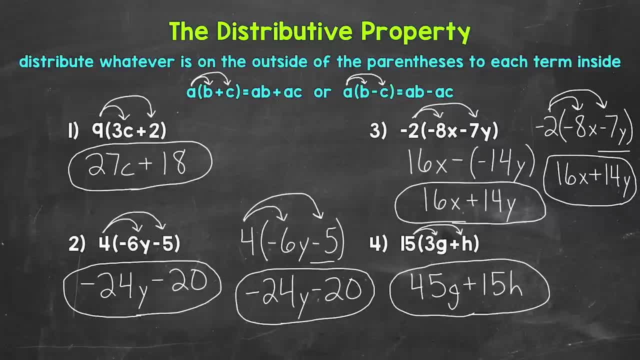 So we can't simplify this any further. This is simplified. So again, 45G plus 15H. So there are the basics of using the distributive property to simplify algebraic expressions. Let's move on to some examples of algebraic expressions that will need to be simplified. 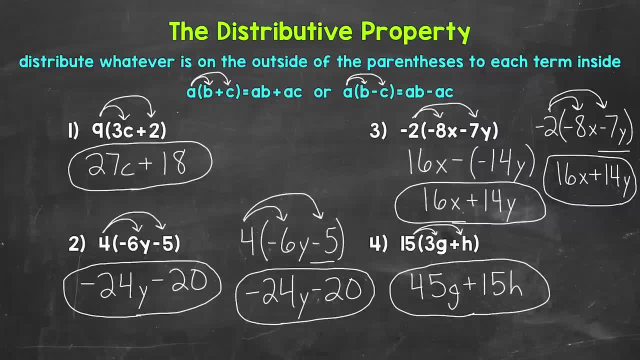 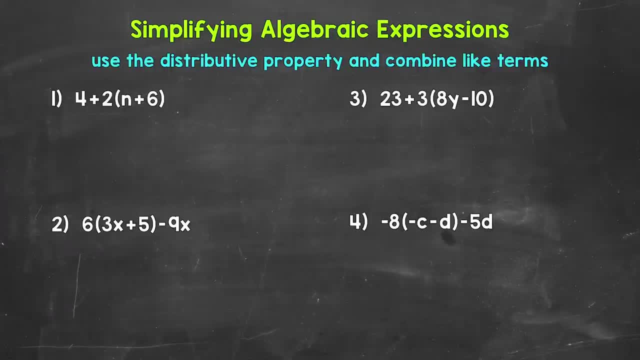 using both the distributive property and combining like terms. Here are four more algebraic expressions that we need to simplify. We will use both the distributive property and the algebraic expressions that we need to simplify. Let's jump into number one, where we have 4 plus 2 and then in parentheses, N plus 6.. 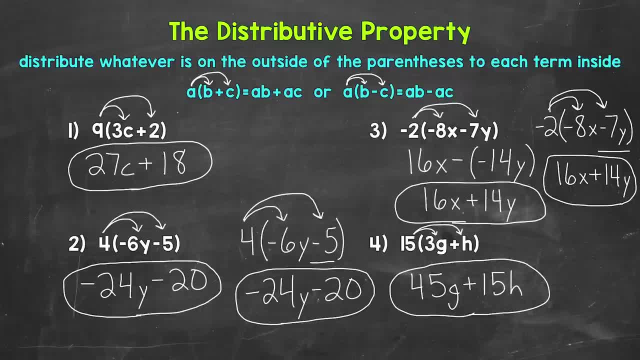 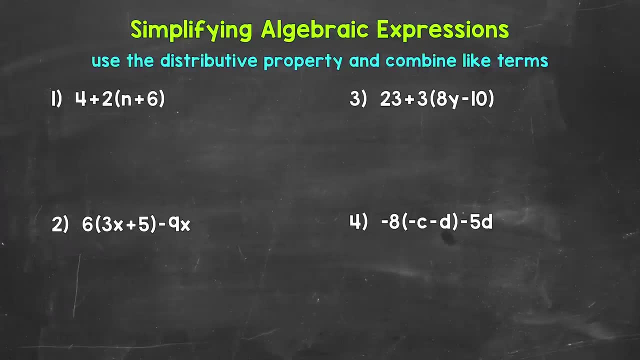 So there are the basics of using the distributive property to simplify algebraic expressions. Let's move on to some examples of algebraic expressions that will need to be simplified using both the distributive property and combining lines. Here are four more algebraic expressions that we need to simplify. 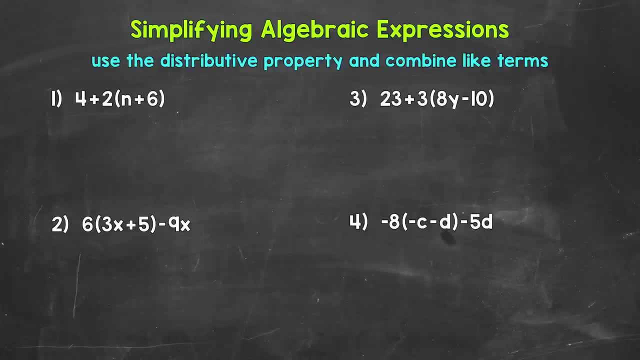 We will use both the distributive property and combining like terms. Let's jump into number 1, where we have 4 plus 2 and then, in parentheses, n plus 6.. Now, since this expression has parentheses, we need to start there. Do not do 4 plus 2 first. 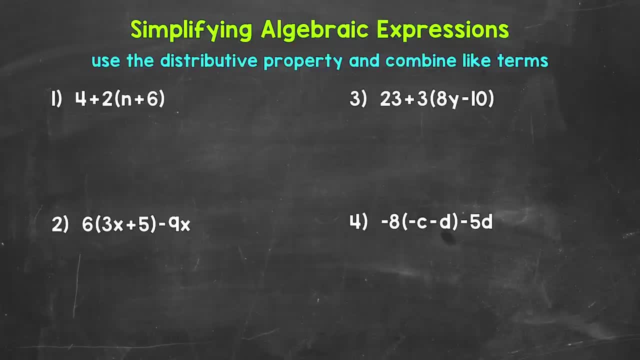 We still need to consider the order of operations. Within the parentheses we have n plus 6.. n and 6 are unlike terms, So we can't combine those terms. What we can do is use the distributive property to remove the parentheses. 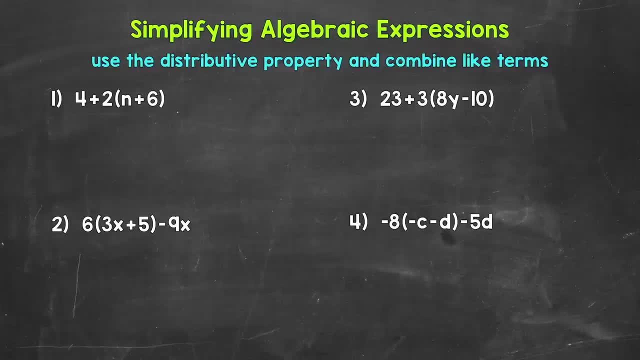 And then we can look to combine like terms to simplify the expression further. So let's distribute the 2 to the n and to the 6.. 2 times n gives us 2n, And then we have 2 times 6,, which gives us a positive 12.. 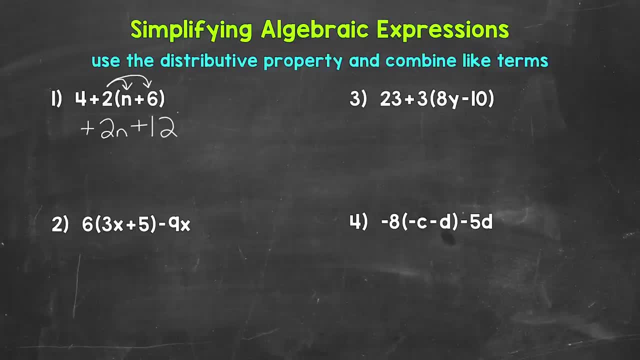 So plus 12.. This is a positive 2n And then we can bring down that 4.. Now that the parentheses have been removed, we can look to simplify further by combining like terms. 4 and 12 are like terms. 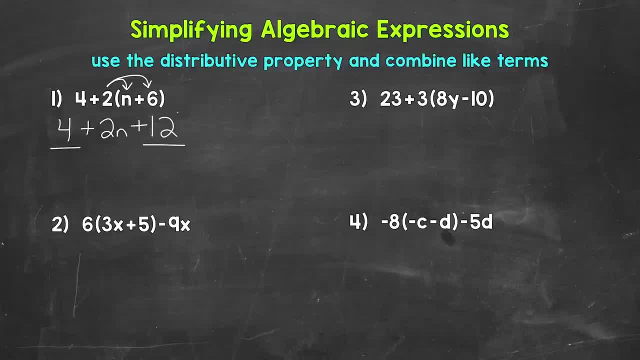 Those are constant terms, So we can combine them: 4 plus 12 gives us 16.. So our final Simplified expression is 2n plus 16.. Now when we write expressions, typically speaking, we want any variable terms first. 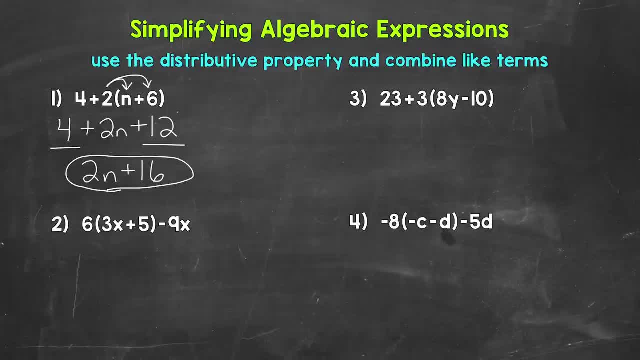 and then constant terms go last. So that's why we have 2n plus 16.. If we end up having multiple terms that involve variables, they go in order from greatest to least as far as exponents, And then if variable terms have the same exponents. 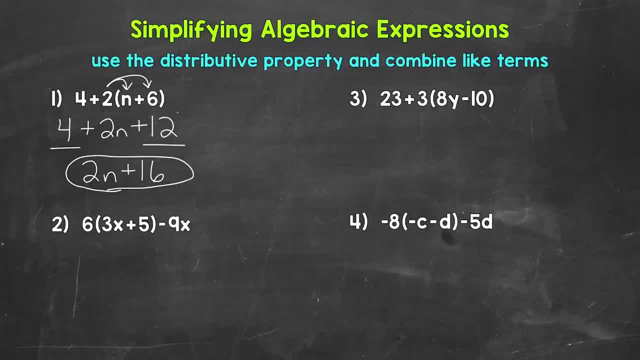 they go in ABC order. So again for number 1, we just have 2 terms: a variable term and then a constant term. So 2n plus 16 is our final simplified expression. Now that final simplified expression is equivalent to the original expression. 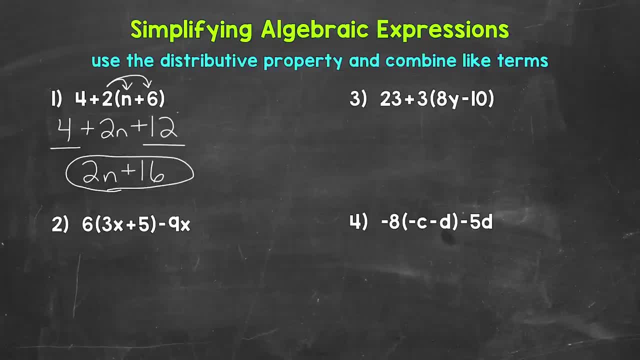 We were just able to simplify that original expression by using the distributive property and combining like terms. Let's move on to number 2, where we have 6, and then in parentheses 3x plus 5, and parentheses minus 9x. 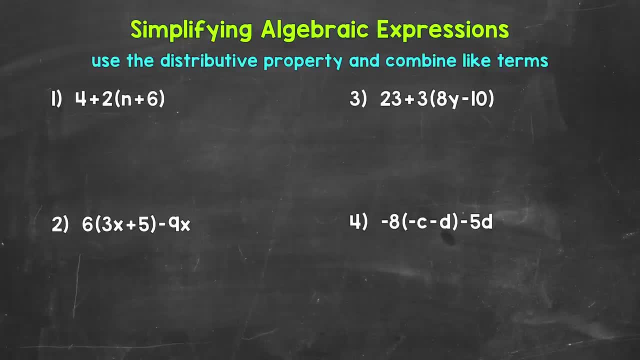 Now, since this expression has parentheses, we need to start there. Do not do 4 plus 2 first. We still need to consider the order of operations. Within the parentheses, we have N plus 6.. N and 6 are unlike terms. 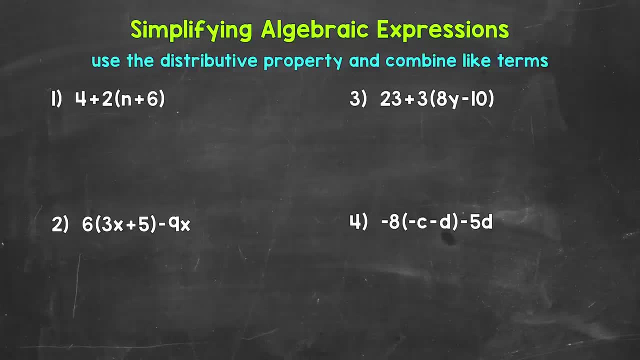 So we can't combine those. What we can do is use the distributive property to remove the parentheses And then we can look to combine like terms to simplify the expression further. So let's distribute the 2 to the N and to the 6.. 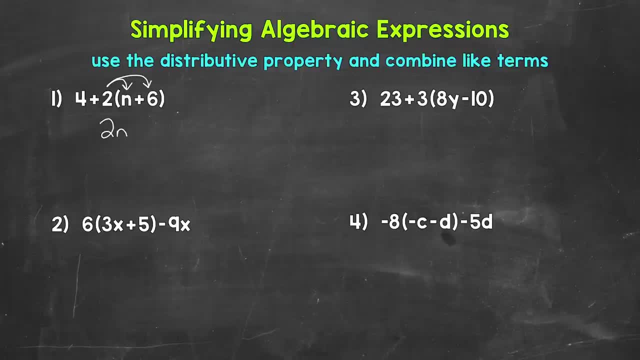 2 times N gives us 2N, And then we have 2 times 6,, which gives us a positive 12.. So plus 12. This is a positive 2N, And then we can bring down that 4.. 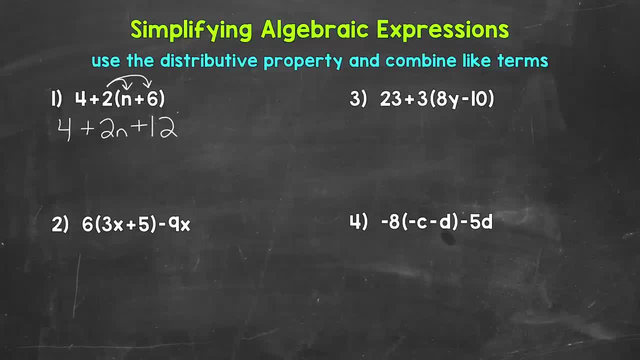 Now that the parentheses have been removed, we can look to simplify further by combining like terms. 4 and 12 are like terms. Those are constant terms, So we can combine them: 4 plus 12 gives us 16.. So our final simplified expression is 2N plus 16.. 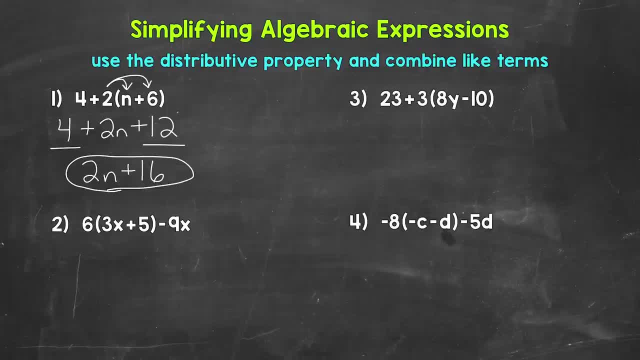 Now, when we write expressions, typically speaking, we want any variable terms first and then constant terms go last. So that's why we have 2N plus 16.. If we end up having multiple terms that involve variables, they go in order from greatest to least. as far as exponents, 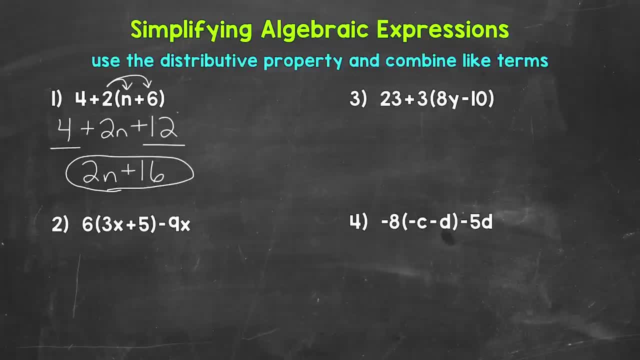 And then, if variable terms have the same exponents, go in ABC order. So again for number one, we just have two terms: a variable term and then a constant. So 2N plus 16 is our final simplified expression. Now that final simplified expression is equivalent to the original expression. 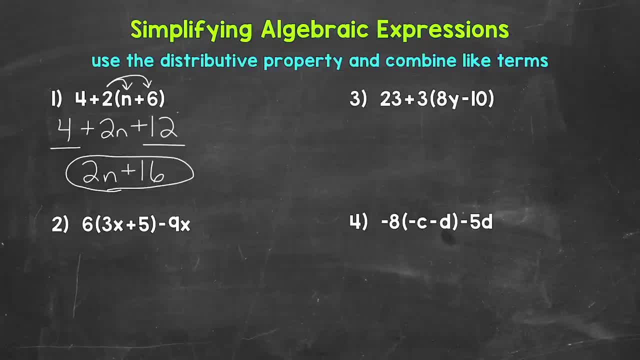 We were just able to simplify that original expression by using the distributive property and combining like terms. Let's move on to number two, where we have 6, and then in parentheses 3X plus 5, and parentheses minus 9X. 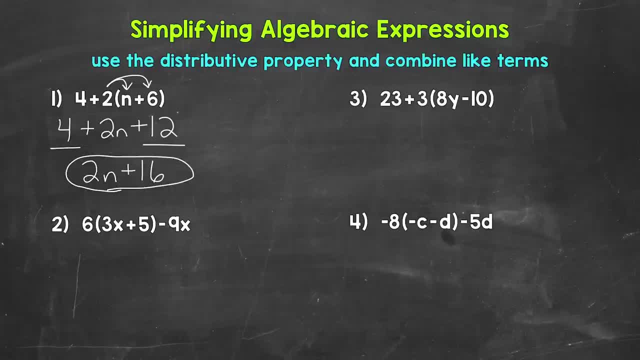 Let's start by using the distributive property to remove the parentheses. So let's distribute this: 6 to the 3x and to the 5.. 6 times 3x gives us 18x, and then 6 times 5 gives us a positive 30,. 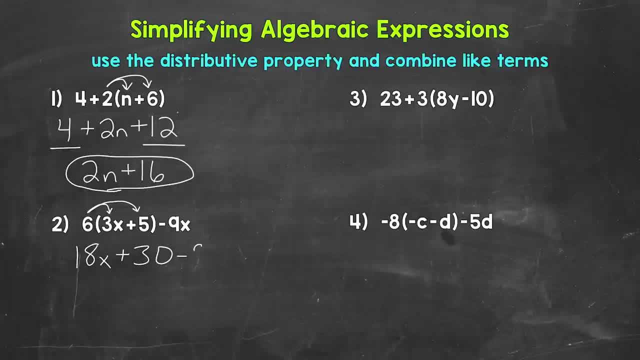 so plus 30. Then we have, Then we have minus 9x, so a negative 9x. Now that we removed the parentheses we can look to combine like terms. 18x and negative 9x are like terms. 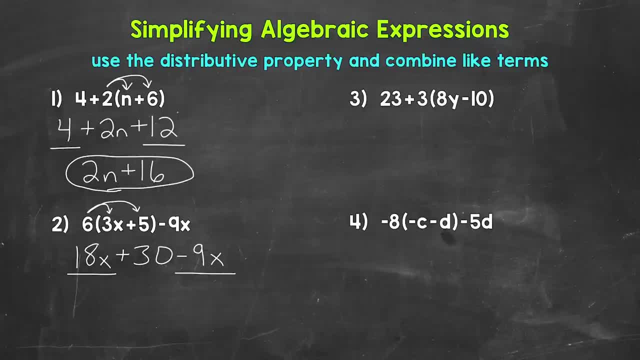 so we can combine them. Make sure to include the sign that's in front of a term That's negative 9x. So we have 18x minus 9x or 18x combined with negative 9x. That gives us: 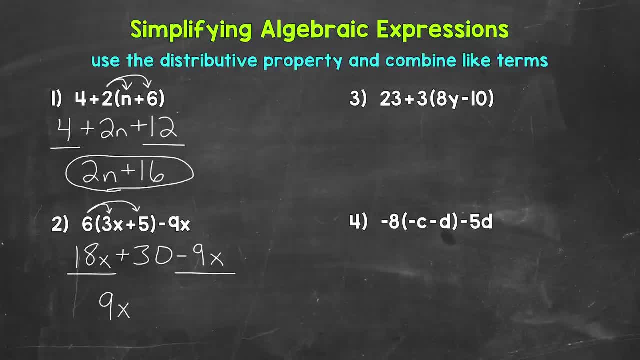 a positive 9x, and then we have plus 30,, a positive 30. So our final simplified expression is 9x plus 30.. Let's move on to number 3, where we have 23 plus 3, and then, in parentheses, 8y minus 10.. 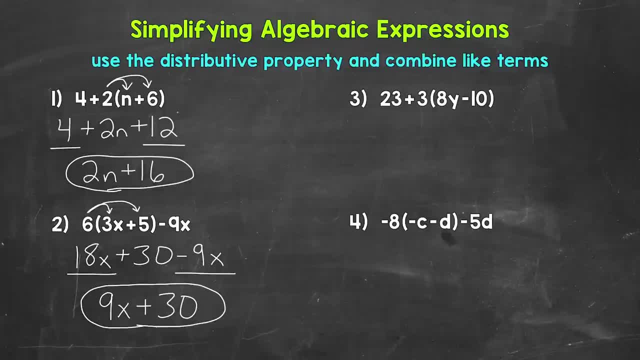 Let's remove the parentheses by using the distributive property. So let's distribute the 3 to the 8y and to the negative 10.. 3 times 8y gives us 24y, and then 3 times negative 10 gives us negative 30.. 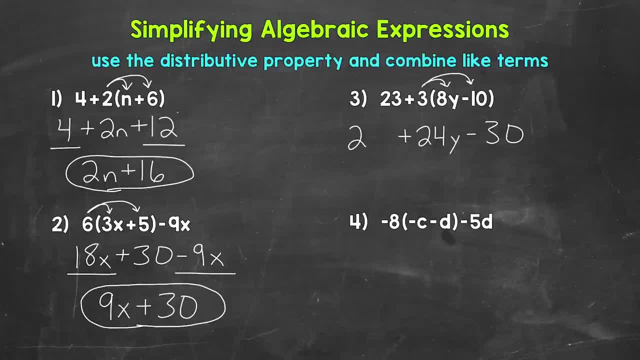 This is a positive 24y, and then bring down the 23.. Now, as far as the distributive property and subtraction, we can also think through that as 3 distributed to 8y, so 3 times 8y, that gives us 24y. 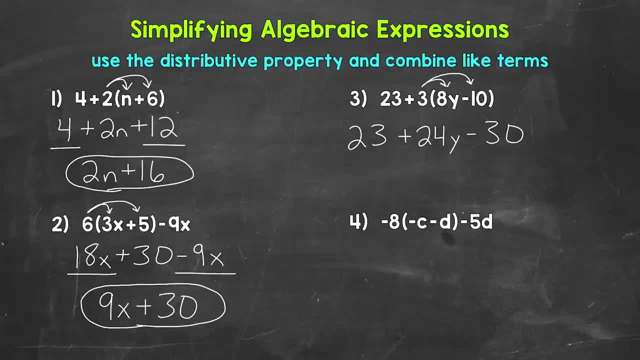 Then we can bring the subtraction sign down and then distribute the 3 to the 10. So 3 times 10, that gives us 30. So 24y minus 30. We got the same thing thinking through the distributive property that way as well. 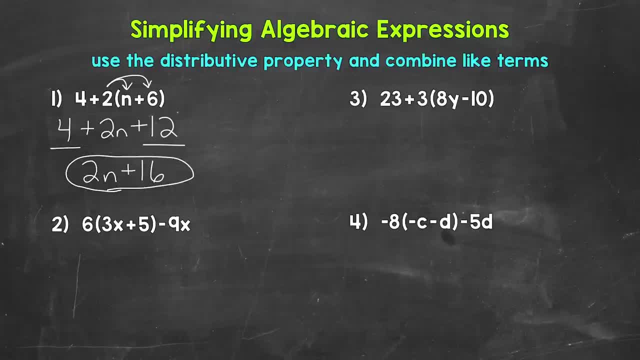 Let's start by using the derivative property. Let's start by using the distributive property to remove the parentheses. So let's distribute this: 6 to the 3X and to the 5.. 6 times 3X gives us 18X. 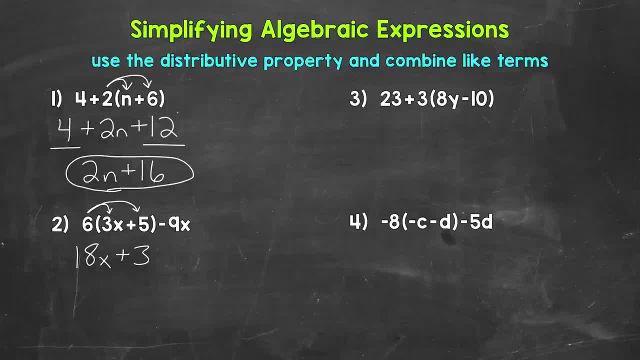 and then 6 times 5 gives us a positive 30,, so plus 30. Then we have minus 9X, so a negative 9X. Now that we removed the parentheses, we can look at the next step. We can look to combine like terms: 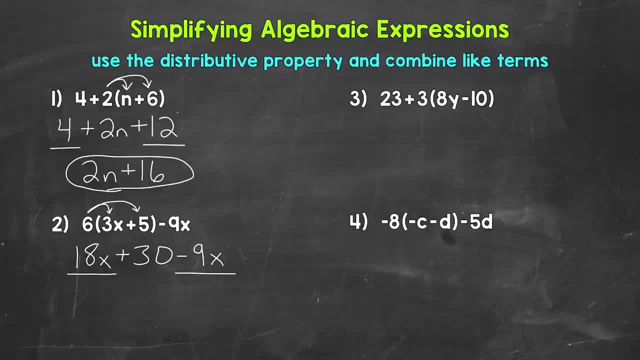 18X and negative 9X are like terms so we can combine them. Make sure to include the sign that's in front of a term That's negative 9X. So we have 18X minus 9X or 18X combined with negative 9X. 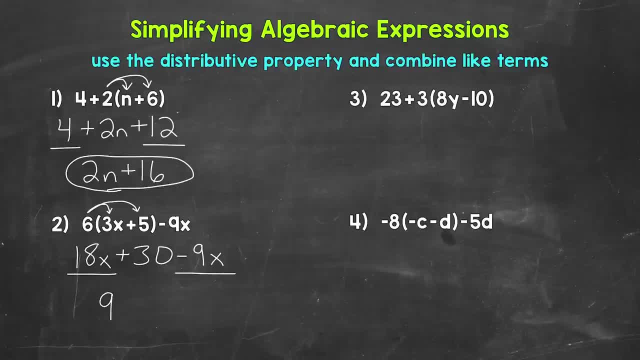 That gives us a positive 9X, and then we have plus 30,, a positive 30. So our final simplified expression is 9X plus 30.. Let's move on to number 3, where we have 23 plus 3,. 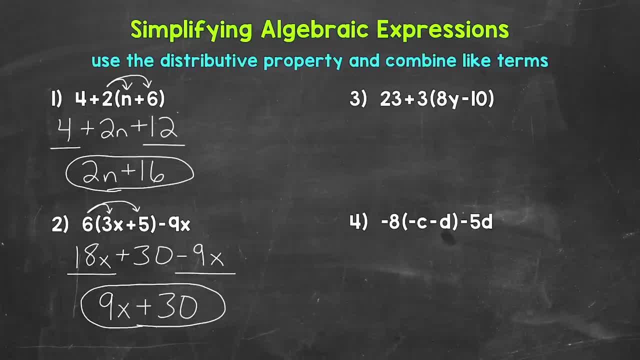 and then in parentheses, 8Y minus 10.. Let's remove the parentheses by using the distributive property. So let's distribute the 3 to the 8Y and to the negative 10.. 3 times 8Y gives us 24Y. 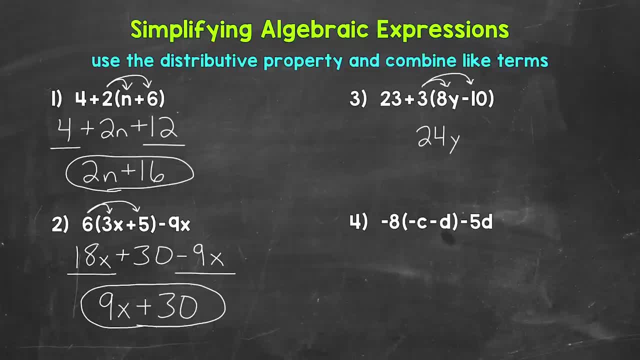 and then 3 times 8Y gives us 24Y. times negative 10 gives us negative 30. This is a positive 24y, and then bring down the 23.. Now, as far as the distributive property and subtraction, we can also think through that as: 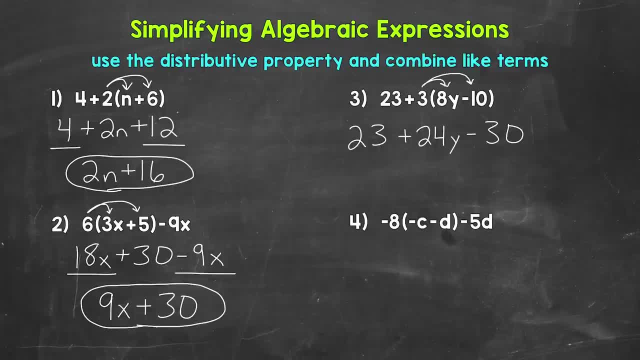 3 distributed to 8y, so 3 times 8y, that gives us 24y. Then we can bring the subtraction sign down and then distribute the 3 to the 10, so 3 times 10, that gives us 30. So 24y minus 30. We got the. 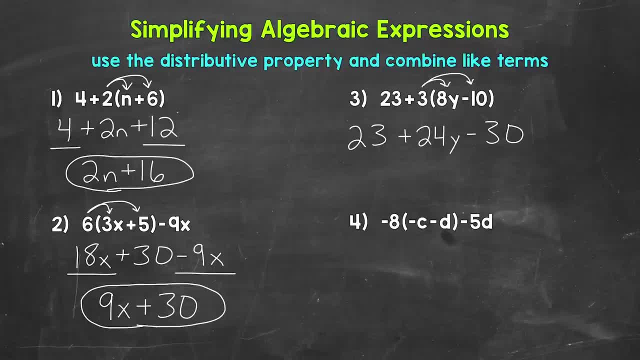 same thing, thinking through the distributive property that way as well. Now that we removed the parentheses, we can look to combine like terms. We have two constant terms, 23 and negative 30, so we can combine those like terms. So we have 24y. 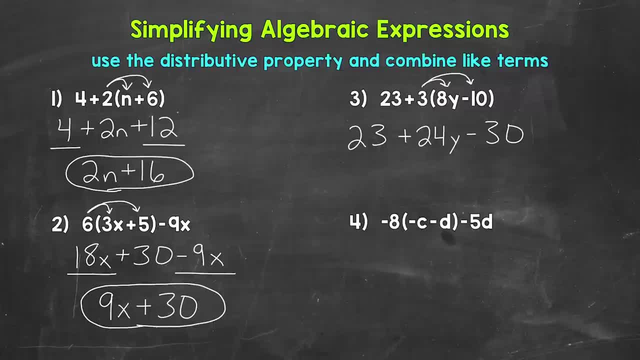 Now that we removed the parentheses we can look to combine like terms. We have two constant terms, 23 and negative 30. So we can combine those like terms. So we have 24y and then 23 minus 30,. 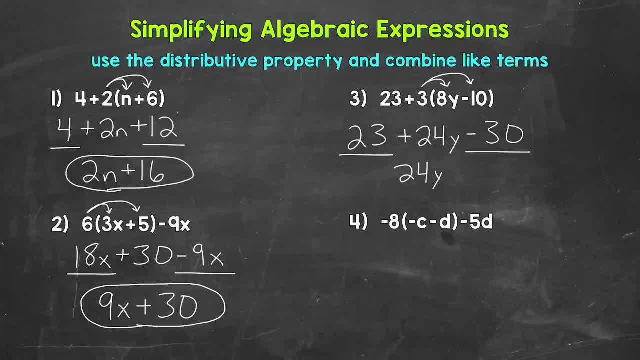 or 23, combined with negative 30, gives us negative 7.. So minus 7.. Our final simplified expression: 24y minus 7.. Lastly, let's move on to number 4, where we have negative 8, and then, in parentheses: 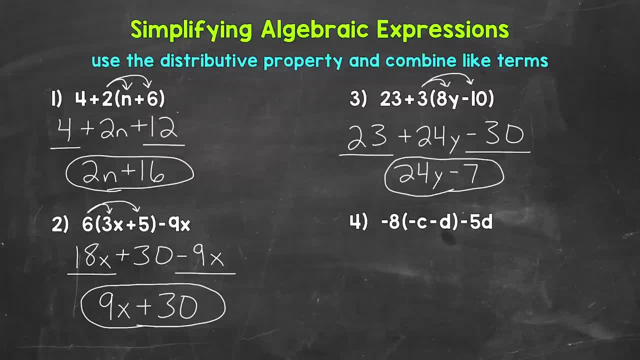 negative c minus 7.. D end parentheses minus 5d. Let's start by removing the parentheses by using the distributive property. Distribute the negative 8 to the negative c and distribute the negative 8 to negative d. 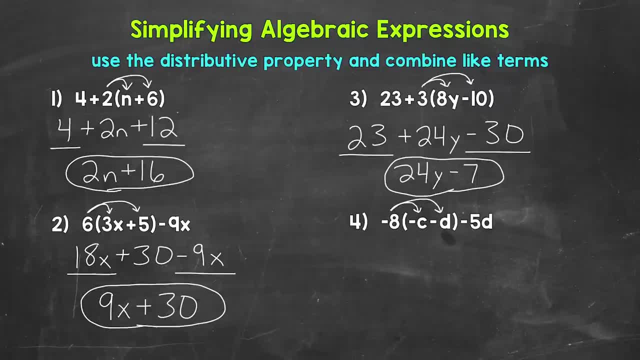 Negative 8 times negative. c gives us a positive 8c. Remember a negative times a negative equals a positive. Negative 8 times negative. d gives us a positive 8d. And then we have minus 5d, so a negative 5d. 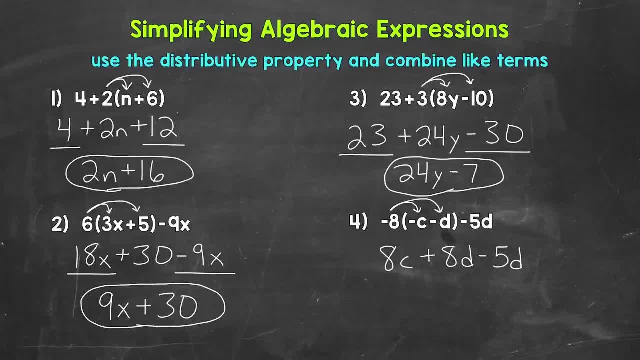 Now that we removed the parentheses we can look to combine like terms. 8d and negative 5d are like terms, So let's combine those like terms. We end up with 8c and then 8d minus 5d. 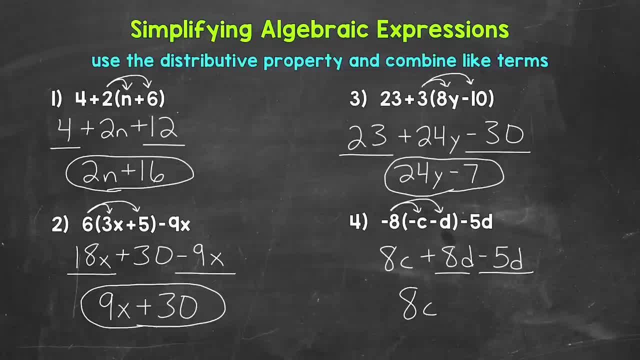 5d or 8d. combined with negative 5d gives us a positive 3d, so plus 3d. Our final simplified expression: 8c plus 3d. So there's how to use the distributive property and combining like terms. 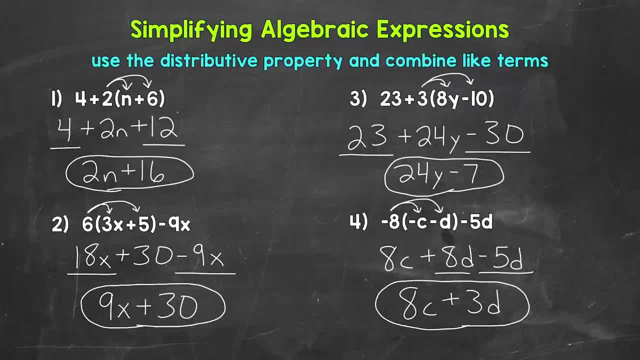 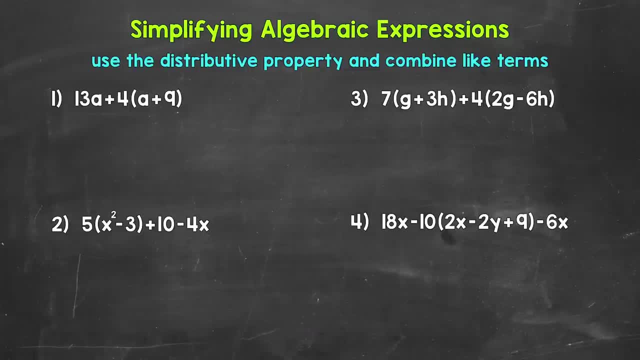 to simplify an algebraic expression. Let's take a look at four more examples, and these will get a little more complex. Here are four more algebraic expressions that we need to simplify using the distributive property and combining like terms. These will get a little more complex. 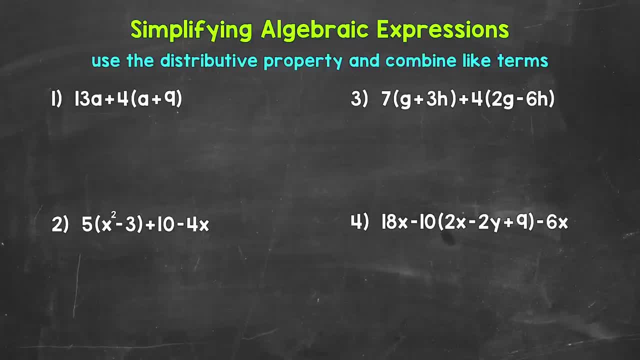 than the previous four examples. Let's jump into number one, where we have 13a plus 4, and then, in parentheses, a plus 9.. Now, since we have parentheses, we need to start there. We can't combine the terms in the parentheses. 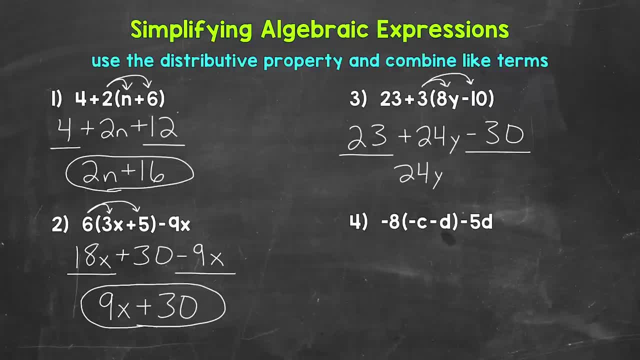 Y, and then 23 minus 30, or 23 combined with negative 30, gives us negative 7,, so minus 7.. Our final simplified expression: 24y minus 7.. Lastly, let's move on to number 4, where we have: 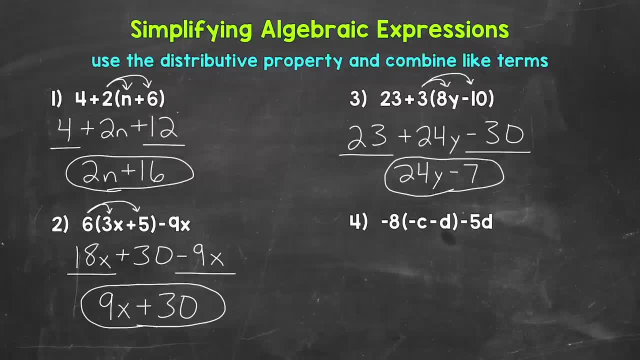 negative 8, and then, in parentheses, negative c minus d. end parentheses minus 5d. Let's start by removing the parentheses by using the distributive property. Distribute the negative 8 to the negative c and distribute the negative 8 to negative d. Negative 8 times negative c gives. 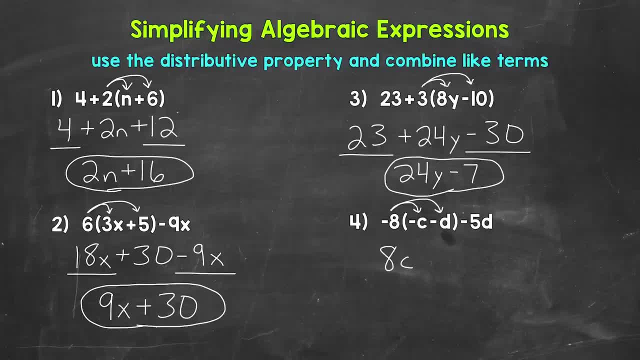 us a positive 8c. Remember: a negative times a negative equals a positive. Negative 8 times negative. d gives us a positive, So we have negative 8d. and then we have minus 5d, so a negative 5d. Now that we removed the 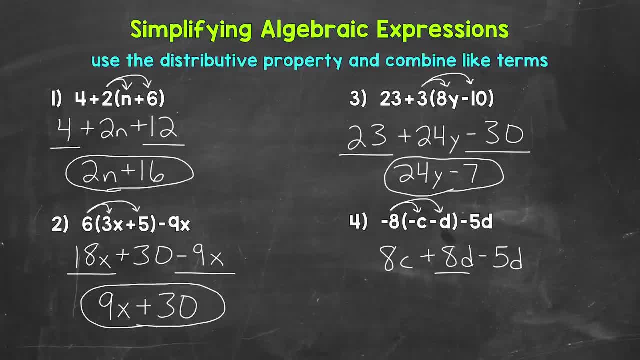 parentheses. we can look to combine like terms. 8d and negative 5d are like terms, so let's combine those like terms. We end up with 8c and then 8d minus 5d or 8d combined with negative 5d. 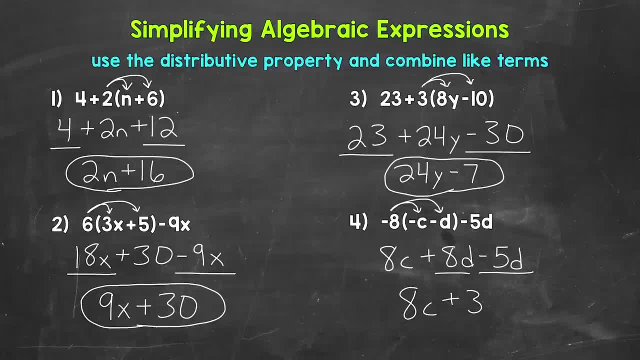 gives us a positive. Our final simplified expression: 8c plus 3d. So there's how to use the distributive property and combining like terms to simplify an algebraic expression. Let's take a look at four more examples, and these will get a little more. 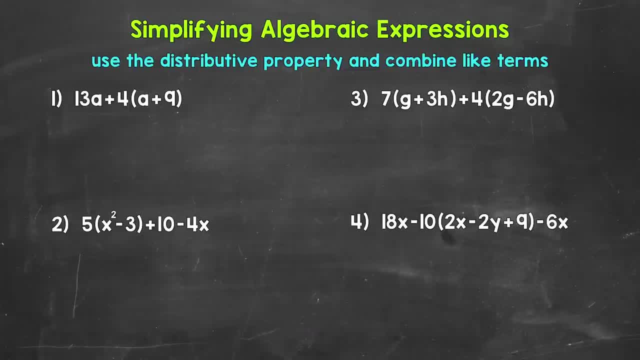 complex. Here are four more algebraic expressions that we need to simplify. using the distributive property and combining like terms. These will get a little more complex than the previous four examples. Let's jump into number 1,, where we have 13a plus 4, and then, in parentheses, a plus 9.. 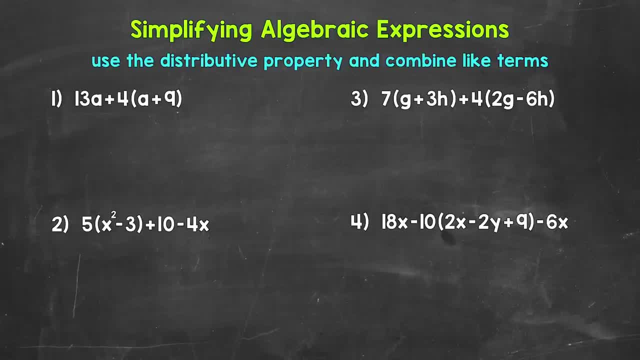 Now, since we have parentheses, we need to start there. We can't combine the terms in the parentheses. they are unlike terms, so we can use the distributive property to remove the parentheses. Once the parentheses are removed, we can look to combine like terms. 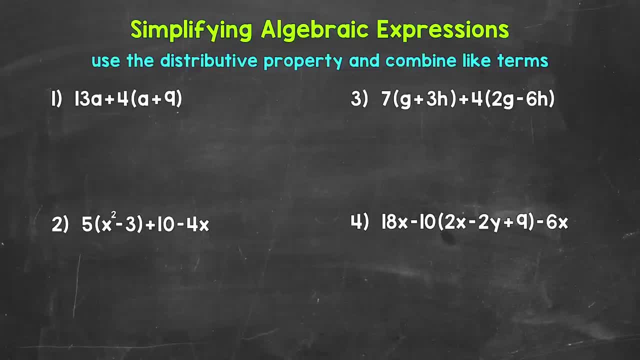 They are unlike terms, so we can use the distributive property to remove the parentheses. Once the parentheses are removed we can look to combine like terms. So let's distribute that 4 to the a and to the 9.. So we have 4 times a. 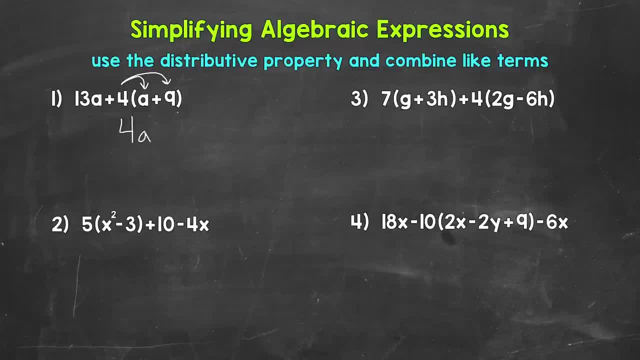 which is 4a, and then 4 times 9 is a positive 36, so plus 36.. This is a positive 4a, and then we can bring down 13a. Now that we removed the parentheses, we can look to combine like terms. 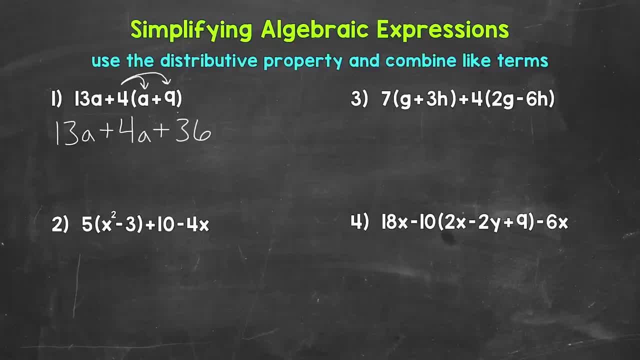 in order to simplify this further. So do we have any like terms that we can combine? Yes, 13a and 4a are like terms, so we can combine those terms. 13a plus 4a is 17a. 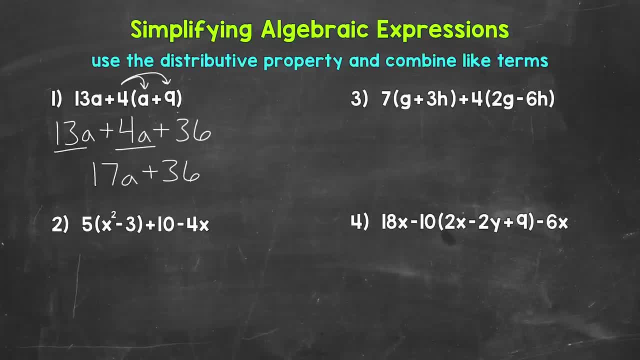 and then we have that positive 36.. So plus 36. And this is our final simplified expression: 17a plus 36.. Now that simplified expression is equivalent to the original expression. We were just able to simplify that original expression by using the distributive property. 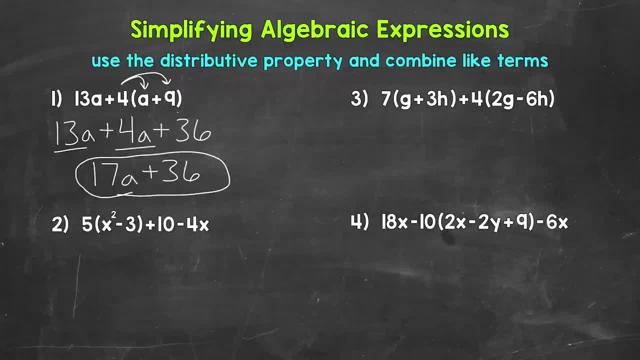 and combining like terms. Let's move on to number 2, where we have 5, and then, in parentheses, x squared minus 3.. End parentheses: Plus 10 minus 4x. Let's start by using the distributive property. 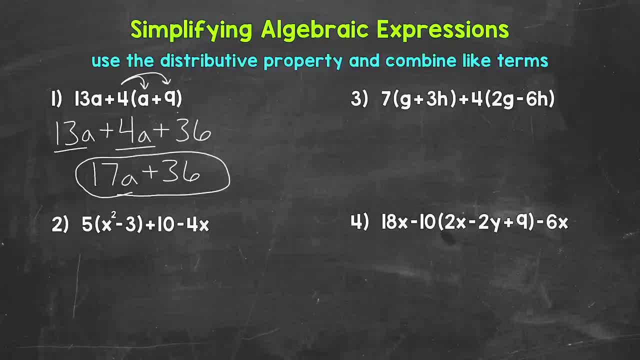 in order to remove the parentheses. Then we can look to combine like terms. Let's distribute this: 5 to the x squared and to the negative 3.. 5 times x squared gives us 5x squared, and then 5 times negative 3. 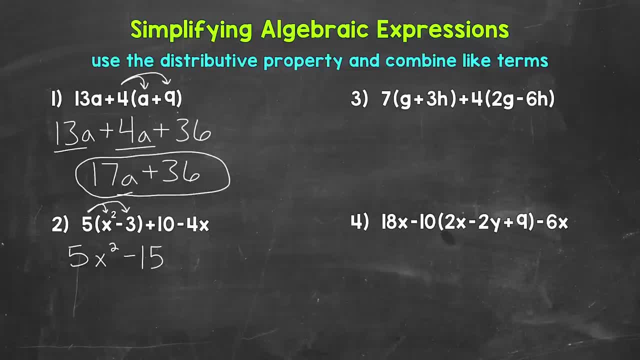 gives us negative 15.. Now another way to think through that distributive property there is to do 5 times x squared, which is 5x squared, Bring the subtraction sign down and then do 5 times 3. We get 5x squared minus 15. 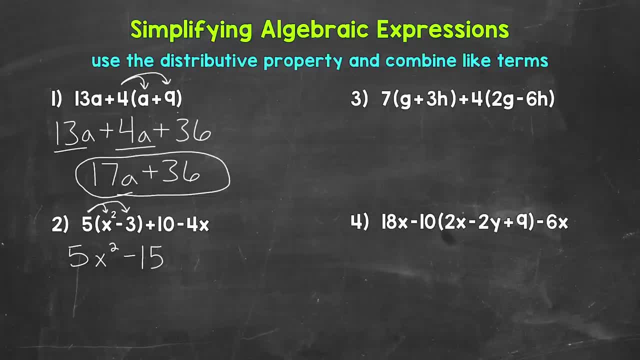 that way as well, Just a slightly different way to think through the distributive property. Then we have a positive 10,, so plus 10, and then a negative 4x, so minus 4x. Now that we have the distributive property. 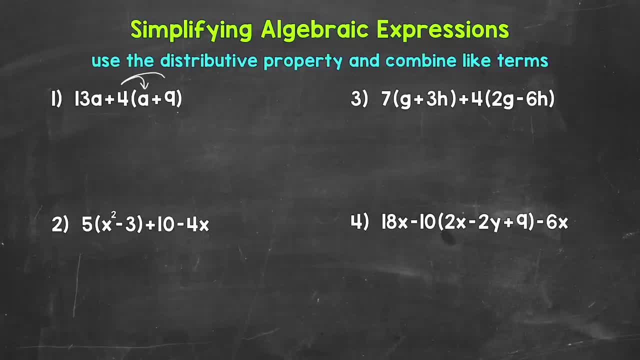 So let's distribute that 4 to the a and to the 9.. So we have 4 times a, which is 4a, and then 4 times 9 is a positive 36, so plus 36.. This is a positive 4a, and then we can bring down 13a. 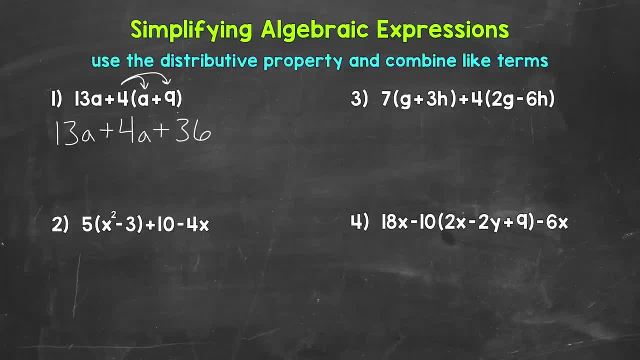 Now that we've removed the parentheses, we can look to combine like terms in order to simplify this further. So do we have any like terms that we can combine? Yes, 13a and 4a are like terms, so we can combine those terms. 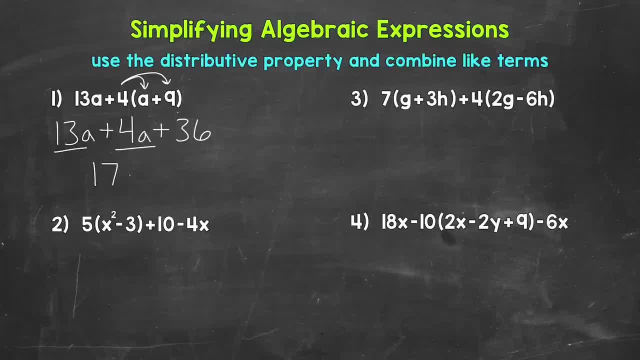 13a plus 4a is 17a, and then we have that positive 36,, so plus 36.. And this is our final simplified expression: 17a plus 4a is a positive 36.. So we can combine those terms. 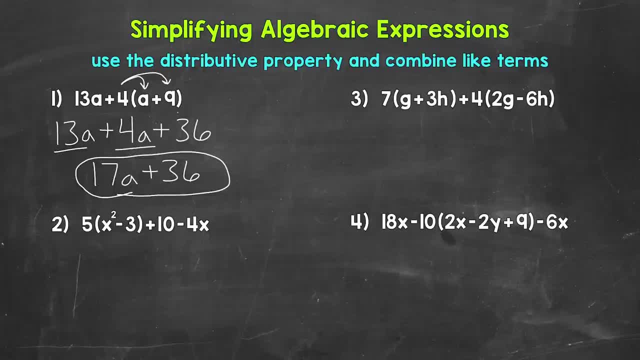 Now that simplified expression is equivalent to the original expression. We were just able to simplify that original expression by using the distributive property and combining like terms. Let's move on to number 2, where we have 5, and then, in parentheses, x squared minus 3,. 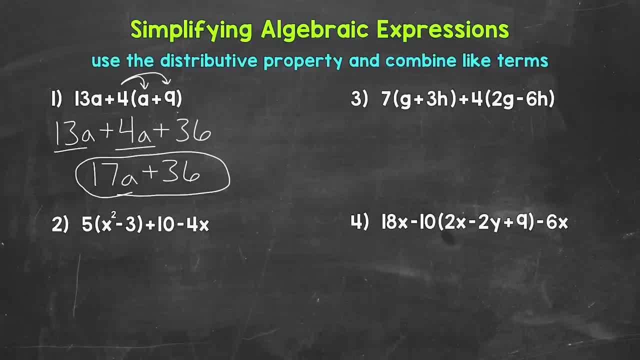 end parentheses. plus 10, minus 4x. Let's start by using the distributive property in order to remove the parentheses. Then we can look to combine like terms. Let's distribute this 5 to the x squared and to the negative 3.. 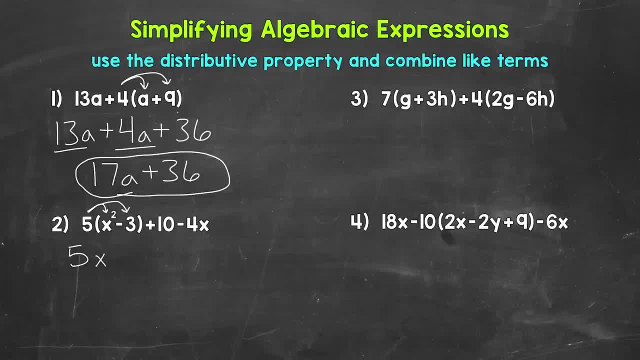 5 times x squared gives us 5x squared, and then 5 times negative 3 gives us negative 15.. Now another way to think through that distributive property: there is to do 5 times x squared, which is 5x squared. 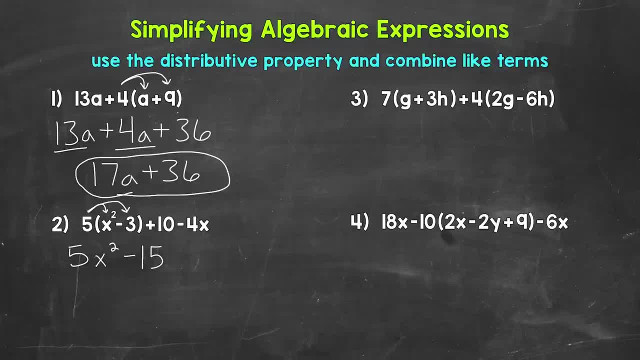 Bring this down, Bring the subtraction sign down and then do 5 times 3.. We get 5x squared minus 15. that way as well, Just a slightly different way to think through the distributive property. Then we have a positive 10,, so plus 10, and then a negative 4x, so minus 4x. 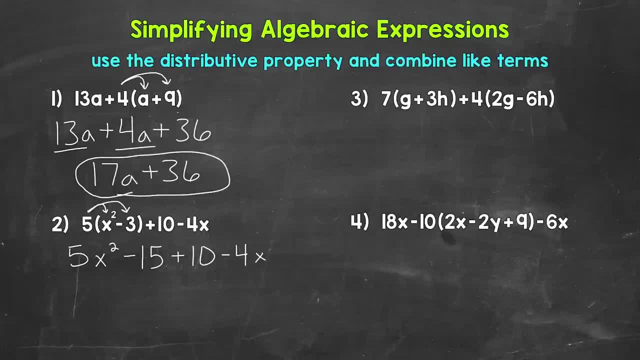 Now that we removed the parentheses, we can look to combine like terms. So do we have any like terms that we can combine? Yes, we have two constant terms Negative, 15 and 10.. So let's combine those like terms. So we have 5x squared minus 4x. 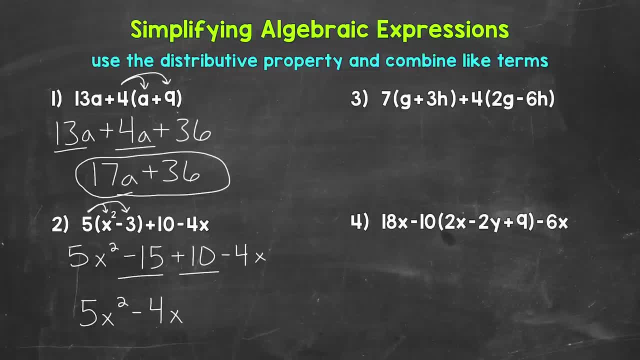 That's a negative 4x. The term will take the sign that's in front of it. So make sure we have negative 4x there, And then the constant term comes last. So we have negative 15 plus 10.. Or negative 15 combined with positive 10.. 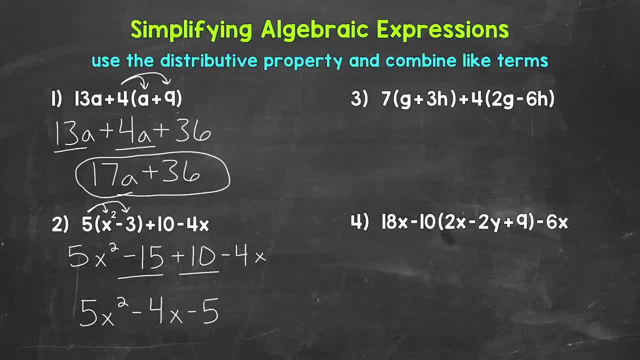 That gives us negative 5.. So minus 5.. And this is our final simplified expression: 5x squared minus 4x minus 5.. Now I do want to mention as far as how this simplified expression is written. typically speaking, when writing expressions, the greatest exponent comes first. 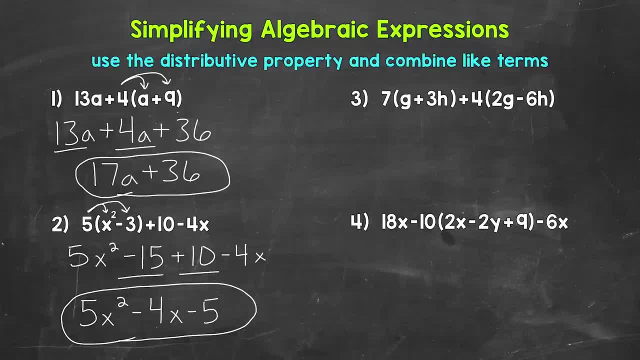 So greatest, to least If exponents are the same, go in ABC order. Constant terms go last. So we have 5x squared. The exponent of 2 comes first, because that's the greatest exponent. Then we have negative 4x. 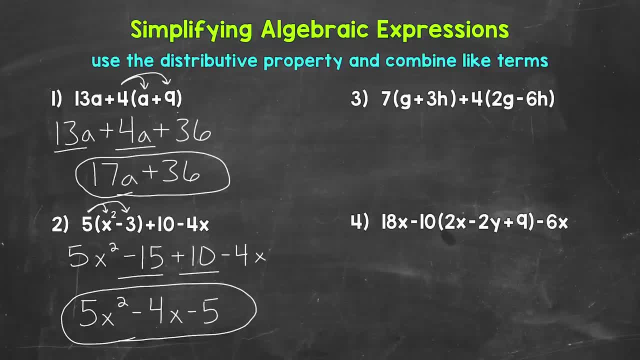 So that variable has an understood exponent of 1.. Remember, whenever there isn't an exponent written, there is an understood exponent of 1.. So to the power of 1.. Anything to the power of 1.. And then we have the constant term of negative 5. last. 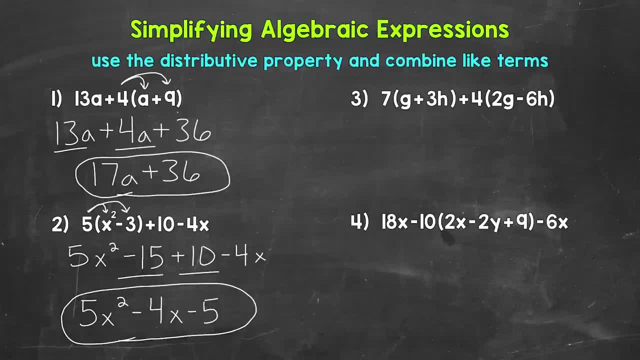 So that's something to keep in mind as far as writing out expressions. Let's move on to number 3, where we have 7. And then, in parentheses, g plus 3h And parentheses plus 4.. And then, in parentheses, 2g minus 6h. 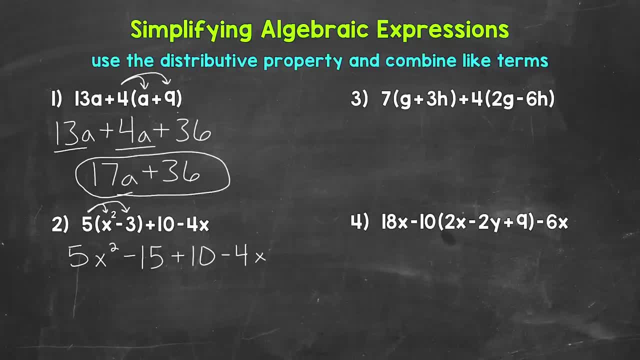 we can look to combine like terms. Do we have any like terms that we can combine? Yes, we have two constant terms, Negative, 15 and 10.. Let's combine those like terms. We have 5x squared minus 4x. 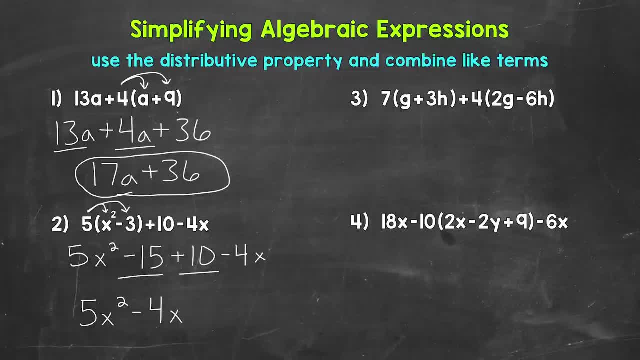 That's a negative 4x. The term will take the sign that's in front of it, so make sure we have negative 4x there. and then the constant term comes last. We have negative 15 plus 10 or negative 15. 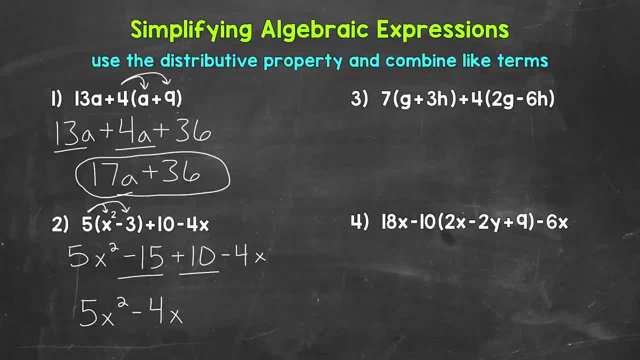 combined with positive 10. That gives us negative 5, so minus 5.. This is our final simplified expression: 5x squared minus 4x minus 5.. I do want to mention as far as how this simplified expression is written. 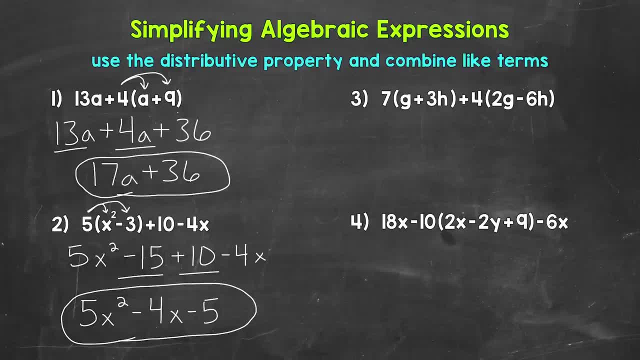 typically speaking, when writing expressions, the greatest exponent comes first, so greatest to least. If exponents are the same, go in ABC order, Constant terms go last. so we have 5x squared. The exponent of 2 comes first because that's the greatest exponent. 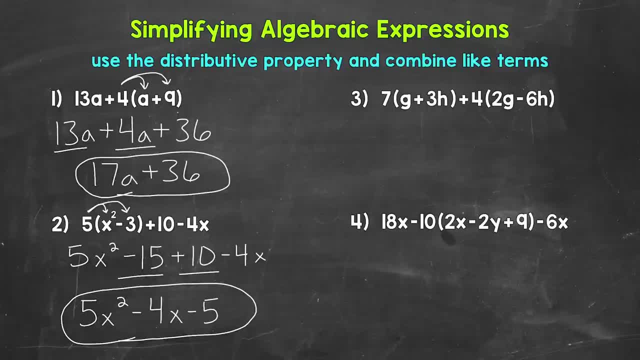 Then we have negative 4x, so that variable has an understood exponent of 1.. Remember, whenever there isn't an exponent written, there is an understood exponent of 1, so to the power of 1.. Anything to the power of 1. 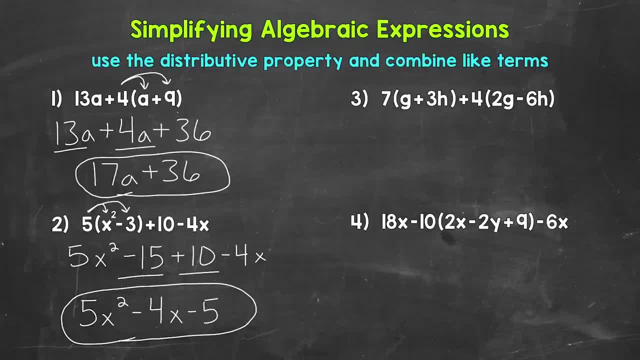 is just itself. Then we have the constant term of negative 5 last. That's something to keep in mind as far as writing out expressions. Let's move on to number 3, where we have 7 and then in parentheses, g plus 3h. 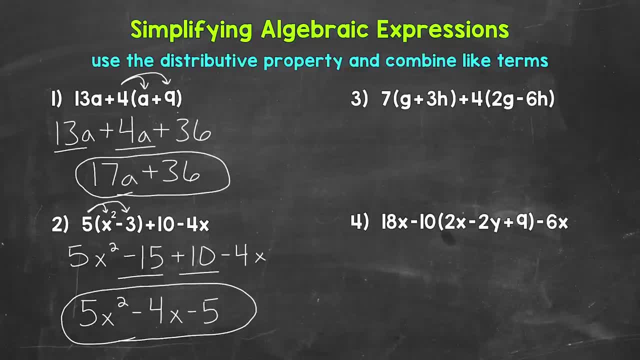 and parentheses plus 4, and then in parentheses, 2g minus 6h. Let's start by using the distributive property to remove any parentheses and then we can look to combine like terms. Let's distribute this 7 to the g and to the 3h. 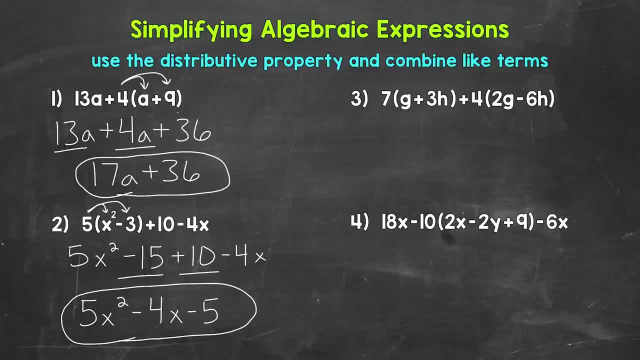 Let's start by using the distributive property to remove any parentheses And then we can look to combine like terms. Let's distribute this 7 to the g and to the 3h, So we have 7 times g. That gives us 7g. 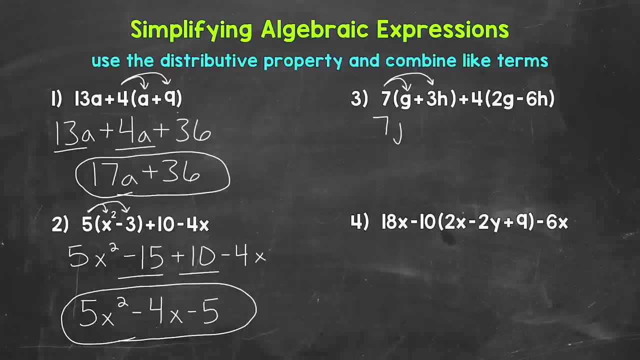 So we have 7 times g, That gives us 7g, And then we have 7 times 3h, That gives us a positive 21h. So plus 21h, Then we can distribute the 4s, 4 to the 2g. 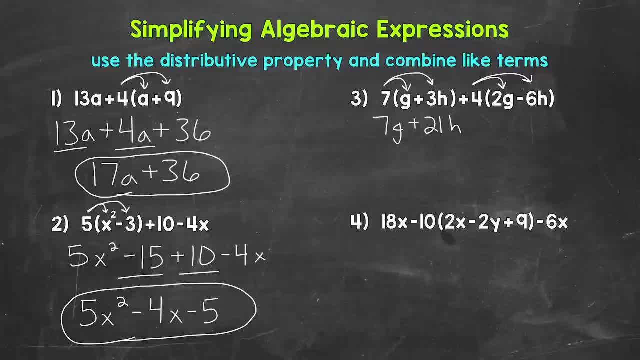 and to the negative: 6h. 4 times 2g gives us a positive 8g, So plus 8g. And then 4 times negative 6h gives us negative 24h. A positive times. a negative equals a negative. 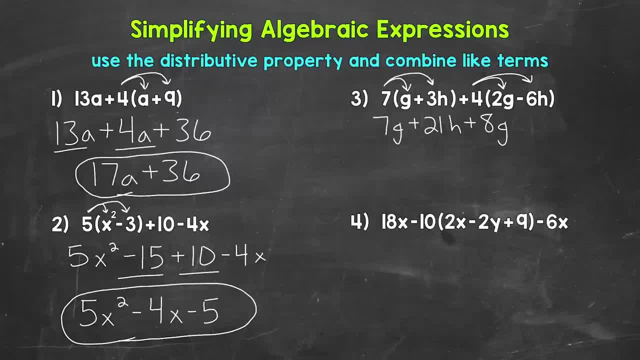 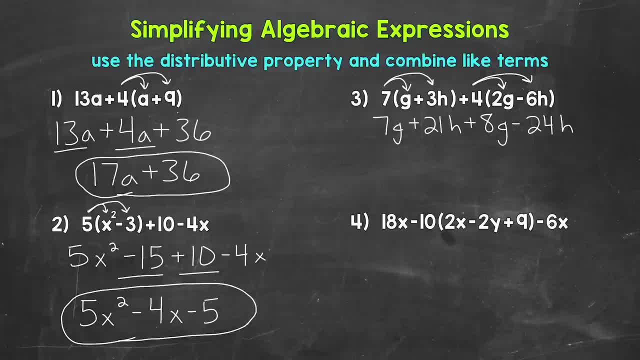 I'm going to rewrite it, with all of the like terms next to each other. This is a strategy we can use to organize the expression and make combining like terms a little simpler, since all of the like terms will be right next to each other. So let's identify any like. 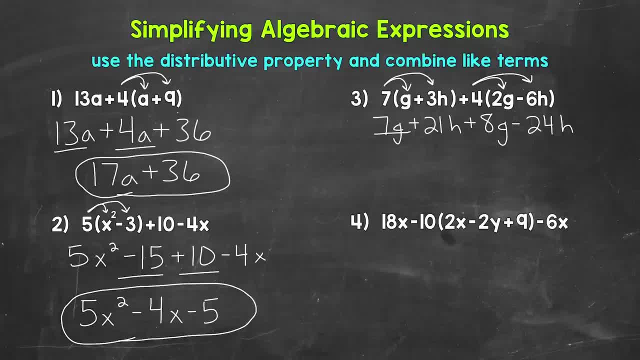 terms in this expression. We have 7g and 8g, And then 21h, which I will box in in order to separate, And then negative 24h. Let's rewrite this with those like terms next to each other. So we have 7g. 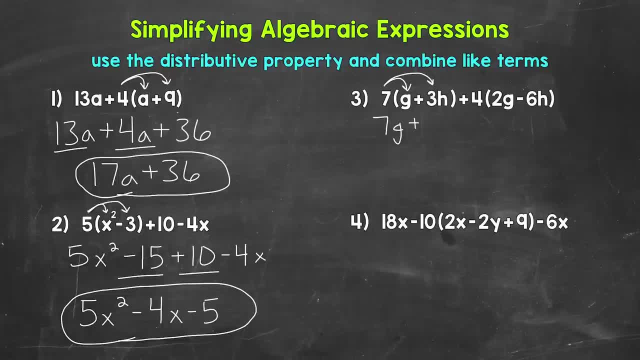 And then we have 7 times 3h. That gives us a positive 21h. So plus 21h. Then we can distribute the 4 to the 2g and to the negative 6h. 4 times 2g gives us a positive 21h. 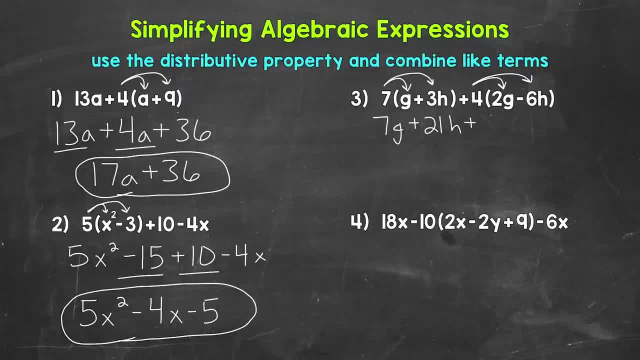 So plus 21h. Negative 8g, So plus 8g, And then 4 times negative: 6h gives us negative 24h. A positive times. a negative equals a negative, So negative 24h or minus 24h. 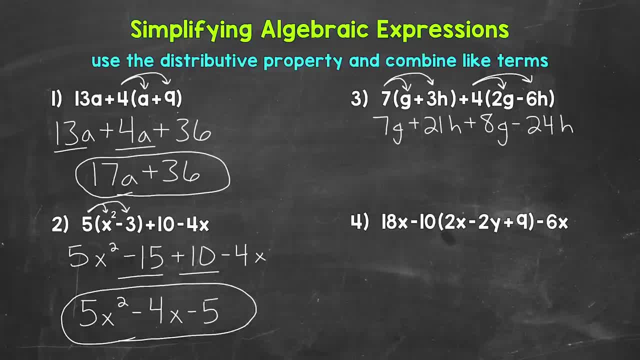 Now for this expression. I'm going to rewrite it with all of the like terms next to each other. This is a strategy we can use to organize the expression And make combining like terms a little simpler, Since all of the like terms will be right next to each other. 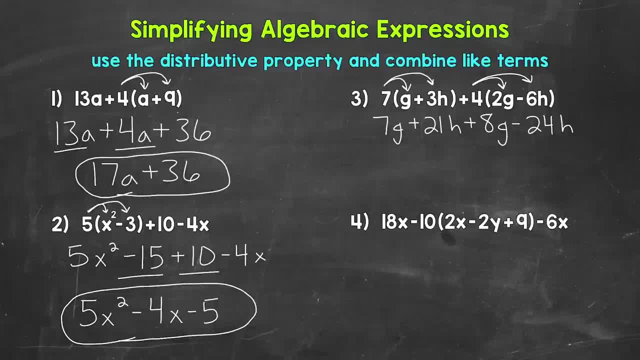 So let's identify any like terms in this expression. We have 7g and 8g, And then 21h, which I will box in in order to separate, And then negative 24h. Let's rewrite this with those like terms next to each other. 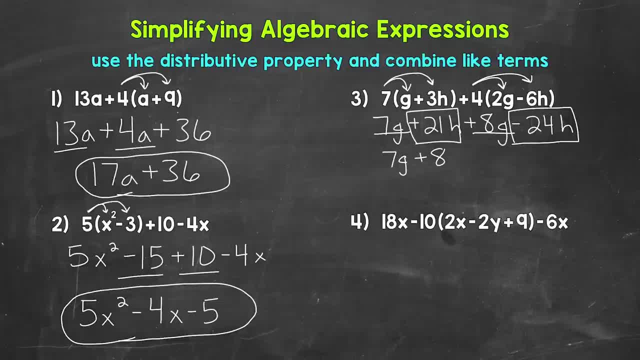 So we have 7g plus 8g, And then we have 7g plus 8g, And then we have 7g plus 8g, And then we have 7g plus 8g plus 21h, minus 24h. 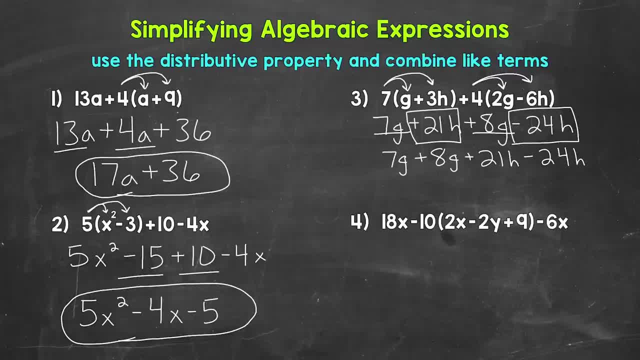 Remember that's a negative 24h. Now all of the like terms are right next to each other, So, like I mentioned, it's a little simpler to combine the like terms. So now we can combine like terms. Let's start with 7g and 8g. 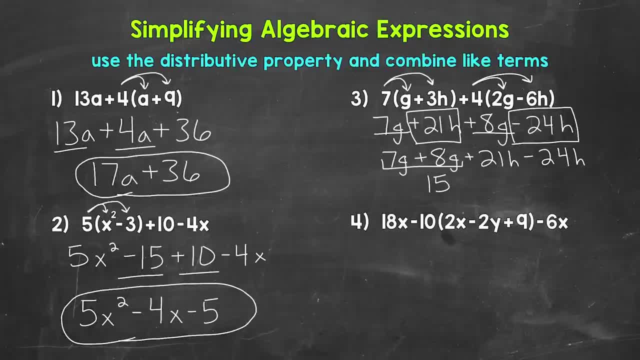 7g plus 8g gives us 15.. 7g plus 8g gives us 15.. 7g plus 8g gives us 15.. Then we have 21h minus 24h, So positive 21h combined with negative 24h. 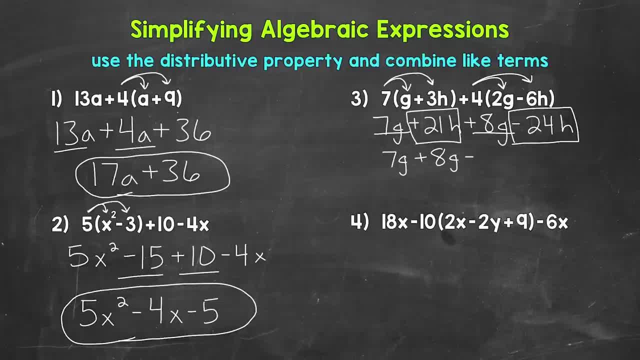 plus 8g, plus 21h minus 24h- Remember that's a negative 24h. Now all of the like terms are right next to each other. So, like I mentioned, it's a little simpler to combine the like terms. So now we can. 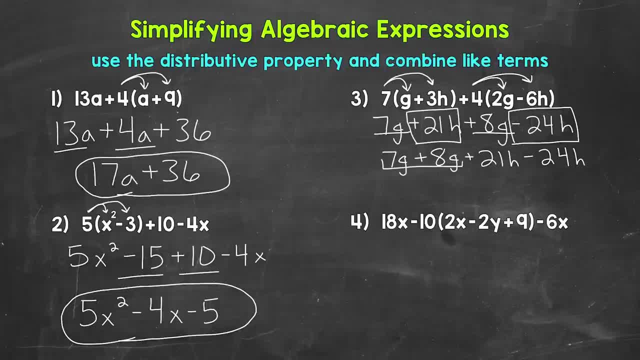 combine like terms. Let's start with 7g and 8g. 7g plus 8g gives us 15g. Then we have 21h minus 24h, So positive 21h combined with negative 24h. That gives us. 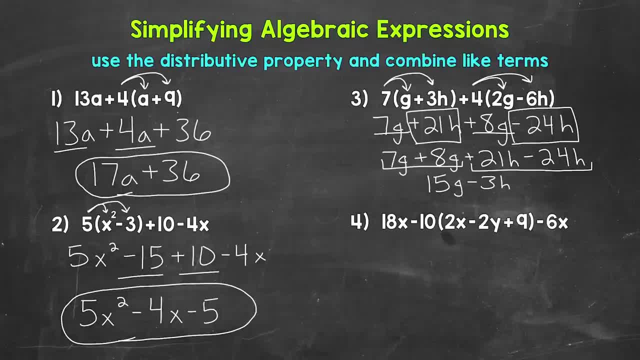 That gives us negative 3h, So minus 3h. And this is our final simplified expression: 15g minus 3h. Lastly, let's move on to number 4. Where we have 18x minus 10.. 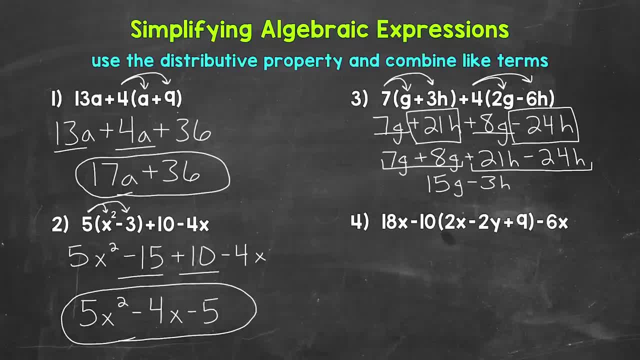 negative 3h, So minus 3h. And this is our final simplified expression: 15g minus 3h. Lastly, let's move on to number 4, where we have 18x minus 10 and then, in parentheses, 2x minus. 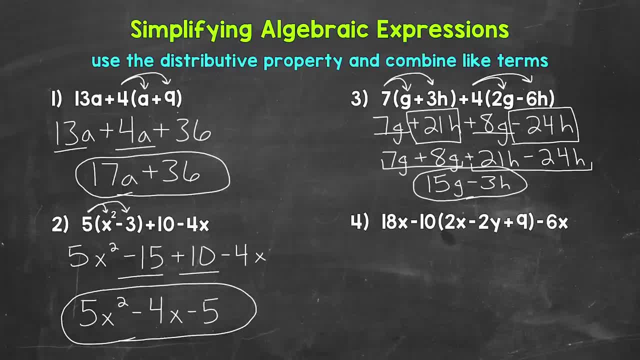 2y plus 9 and parentheses minus 6x. Let's start by using the distributive property to remove the parentheses. We're going to distribute negative 10.. We take the sign that's in front. So this is negative 10.. We need to. 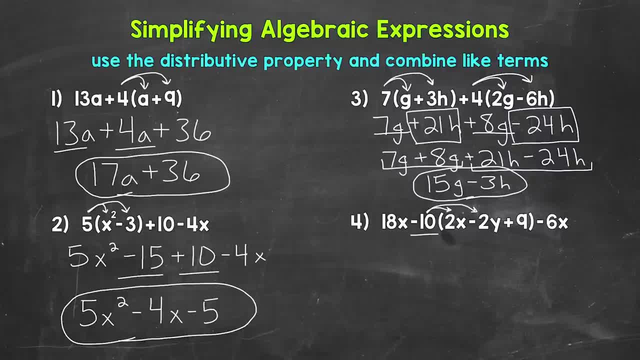 distribute to the 2x, to the negative 2y and to the 9.. Negative 10 times 2x gives us negative 20x. Negative 10 times negative 2y gives us positive 20y. Remember a negative times. 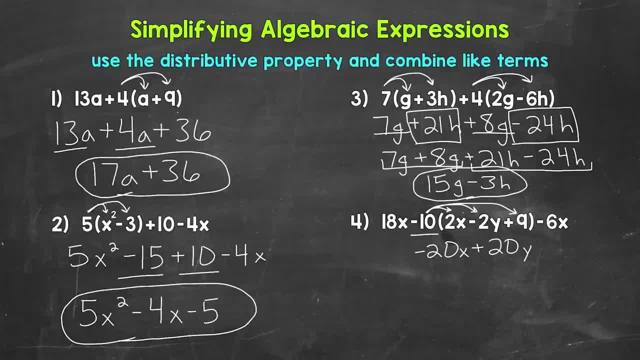 a negative equals a positive, And then we have negative 10 times a positive 9. That gives us negative 90. We then have the negative 6x and the positive 18x that we need to bring down. Now we can look for any like terms. 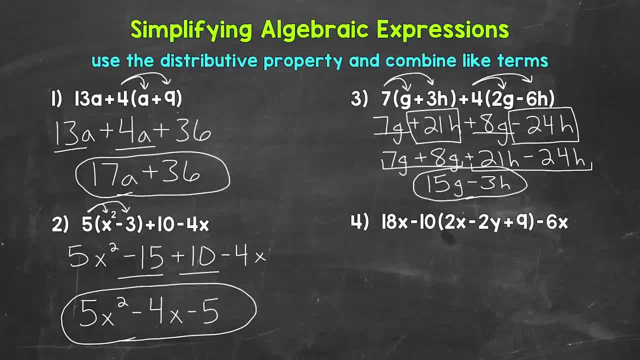 And then in parentheses 2x minus 2y plus 9. And parentheses minus 6x. Let's start by using the distributive property to remove the parentheses. We're going to distribute negative 10.. We take the sign that's in front. 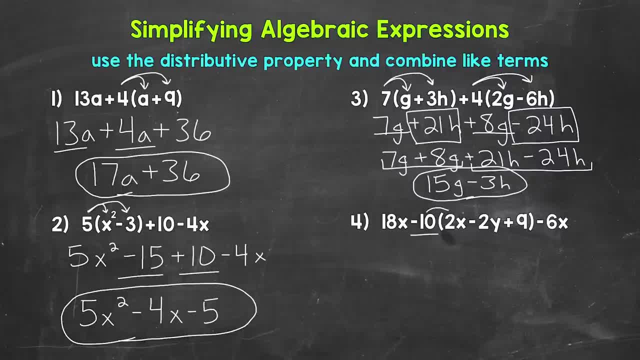 So this is negative 10. We need to distribute to the 2x, To the negative, 2x To the 2y And to the 9. Negative 10 times 2x gives us negative 20x. Negative 10 times negative 2y gives us positive 20y. 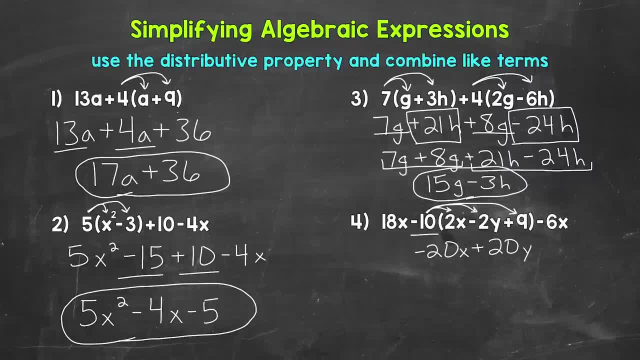 Remember, a negative times a negative equals a positive. And then we have negative 10 times a positive 9. That gives us negative 90. We then have the negative 6x and the positive 18x that we need to bring down. 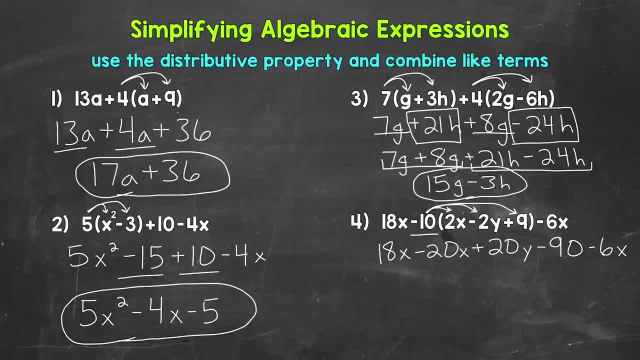 Now we can look for any like terms that we can combine. So do we have any like terms: Yes 18x, negative 20x and negative 6x? Let's rewrite the expression with those like terms next to each other. 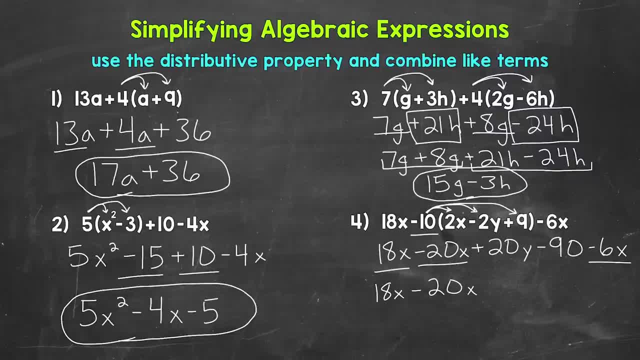 So 18x minus 20x Negative, 20x Negative, 6x Negative, 6x minus 6x plus 20y minus 90.. Now we can combine like terms. So we have 18x minus 20x minus 6x. 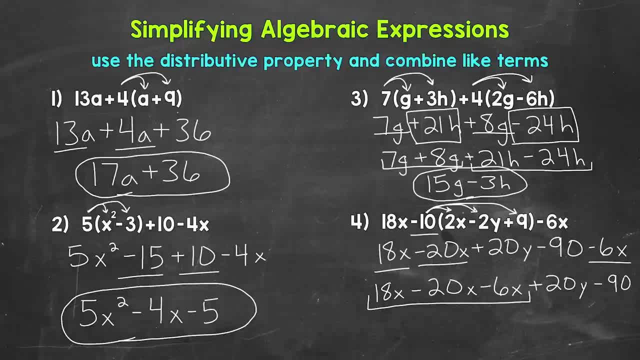 So we are combining a positive 18x, a negative 20x and a negative 6x. 18x minus 20x is negative 2x, Negative, 2x minus 6x. that gives us negative 8x. 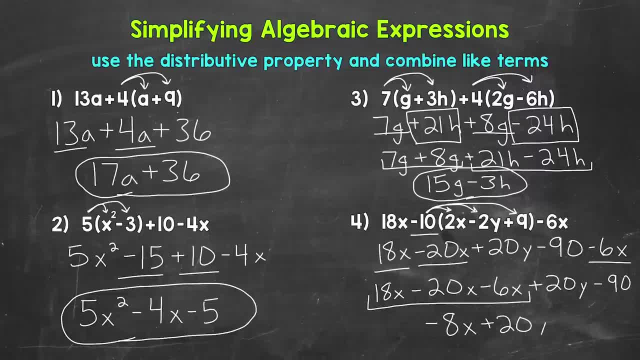 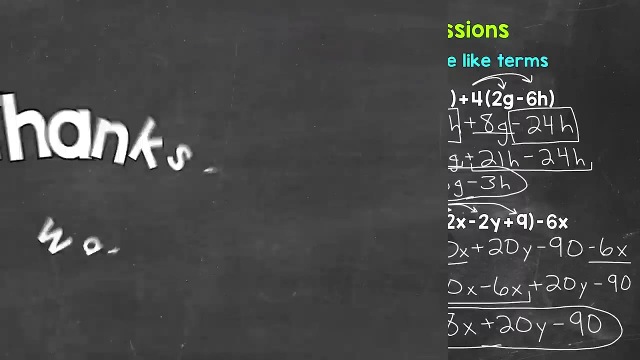 Then we have plus 20y minus 90. So negative 8x plus 20y minus 90 is our final simplified expression. So there's how to simplify algebraic expressions by combining like terms and using the distributive property. I hope that helped. 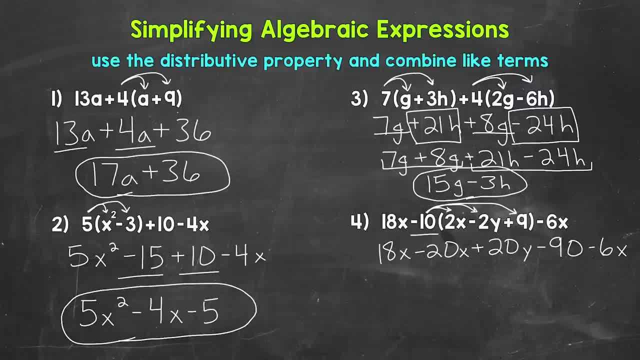 that we can combine. So do we have any like terms? Yes, 18x, negative 20x and negative 6x. Let's rewrite the expression with those like terms next to each other, So 18x minus, 20x minus. 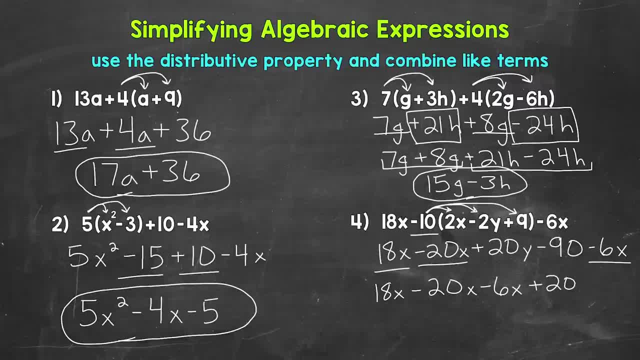 6x plus 20y minus 90. Now we can combine like terms. So we have 18x minus 20x minus 6x. So we are combining a positive 18x, a negative 20x and a negative. 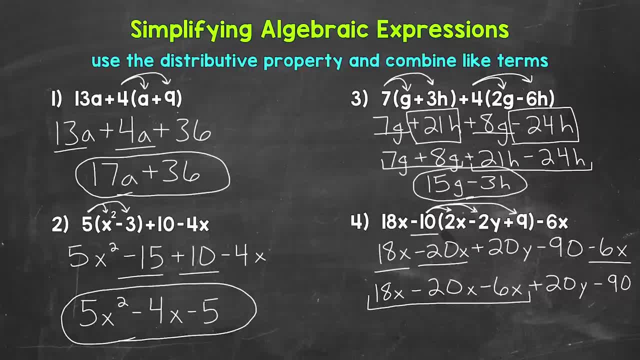 6x, 18x minus 20x is negative 2x. Negative 2x minus 6x, that gives us negative 8x. Then we have plus 20y minus 90. So negative 8x plus 20y minus. 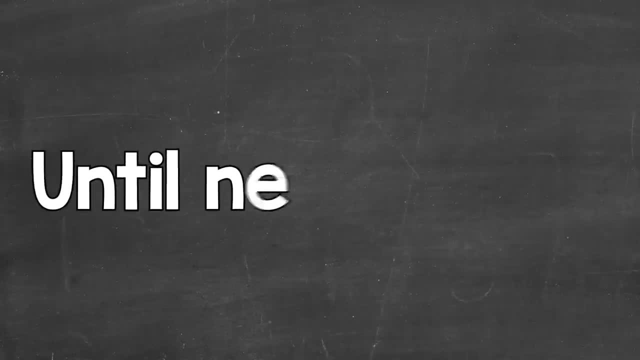 Thanks so much for watching. Until next time, peace. 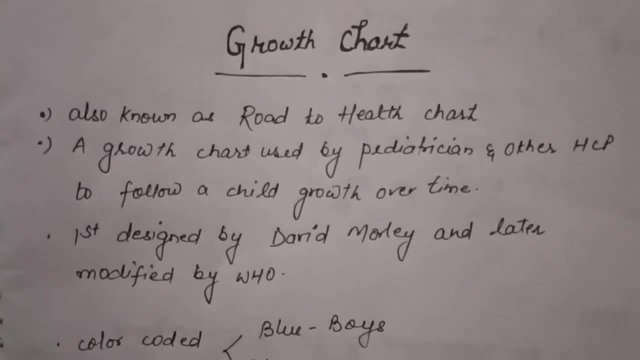 Hello students, a warm welcome in my YouTube channel. In this video, we will be discussing about growth chart or growth curve. Growth curve is also known as road to health chart. It is the chart that is used by pediatrician or other healthcare professionals so that we can 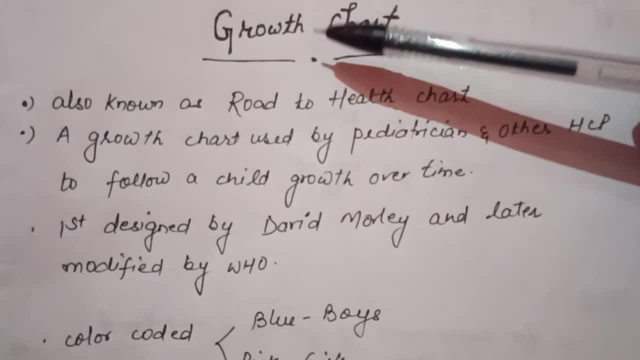 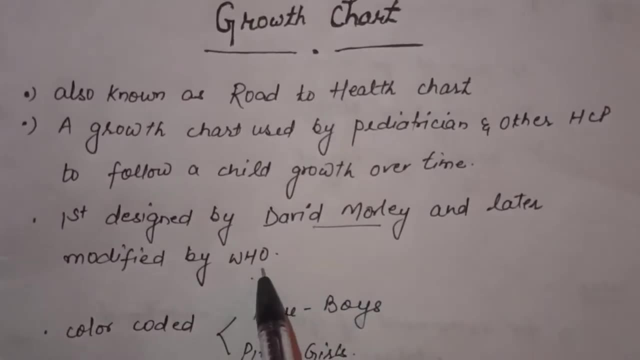 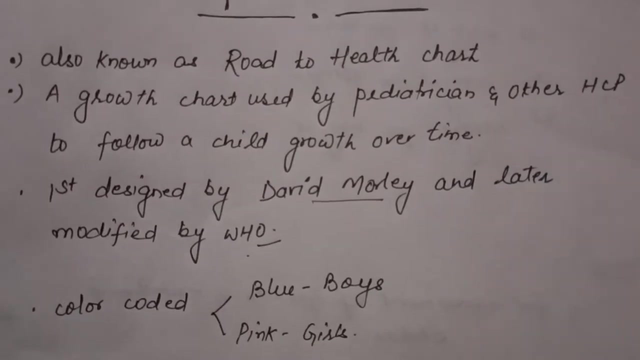 able to assess the growth of a child according to age, whether it is appropriate or not. It was first designed by David Morley and later it was modified by WHO. We are having two colors of growth chart: Blue is for boys and pink is for girls. You can see that this blue color- 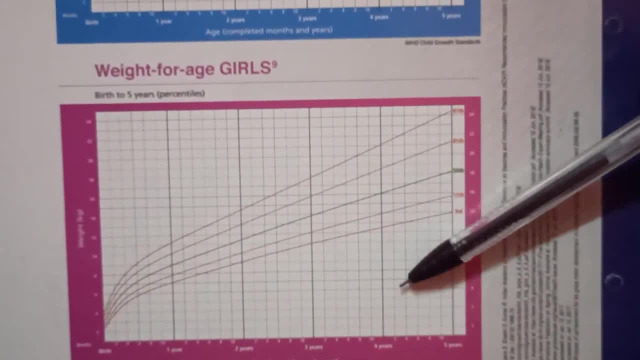 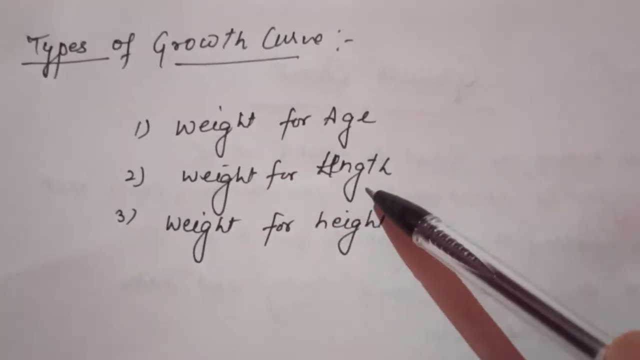 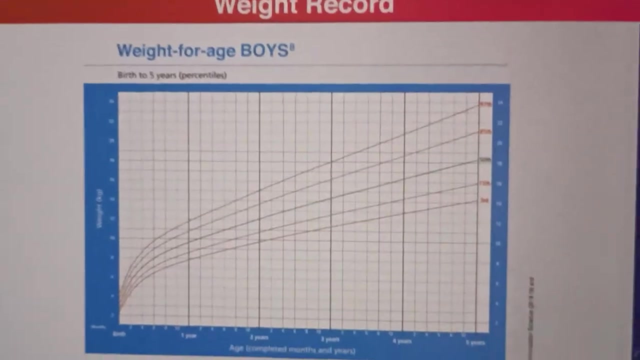 growth chart is for boys and pink color growth chart is for girls. Growth curve is of three types. One is weight for age, weight for length and weight for height. Now we will see how we will measure the growth chart. This growth curve is for weight, for age and it is blue in color. so 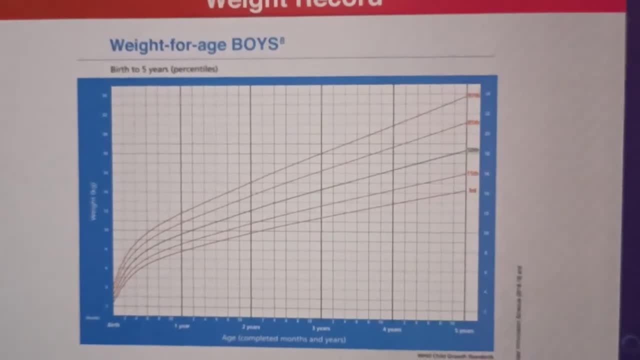 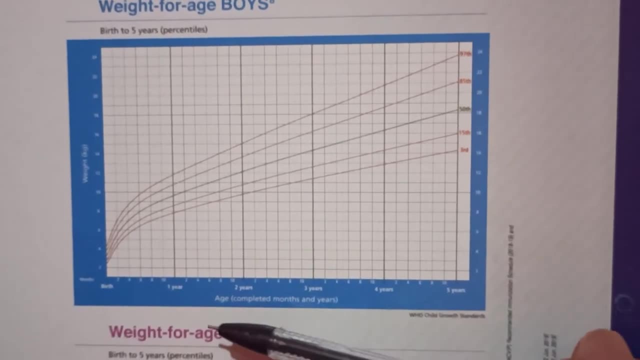 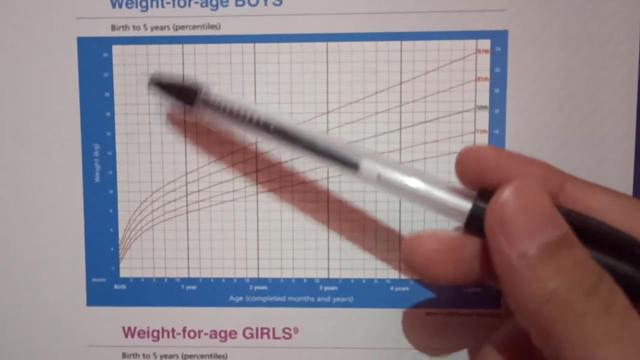 for boys. So weight for age. that means we are having weight component and the age component. So on the x-axis you can able to see that age is written in the month and the years and on the y-axis you can able to see that the weight is written of a child. You can able to see some of 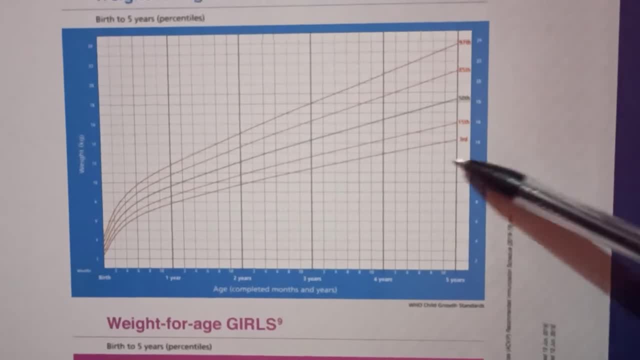 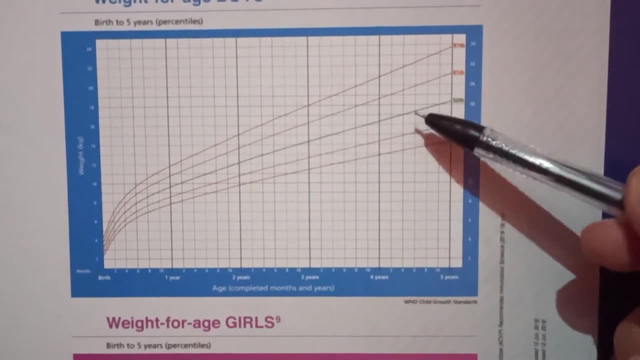 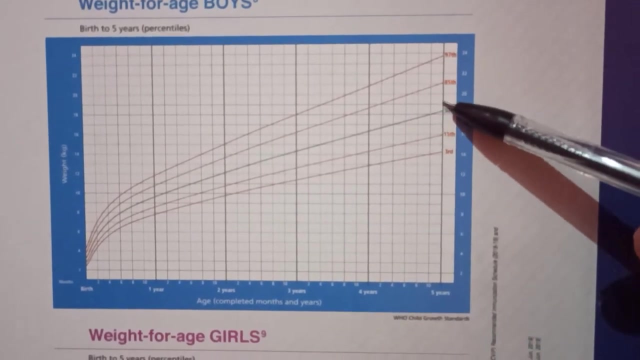 the lines they have been drawn. These lines, they are known as reference line. This is the midline. So on the x-axis you can able to see on the plus sign that the child is having weight component and below the line that means the child is having underweight or malnutrition If it is falling.